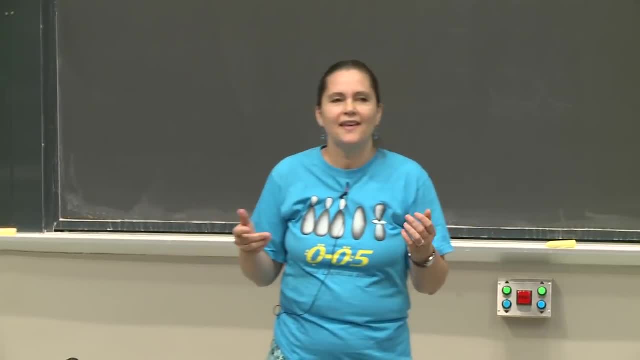 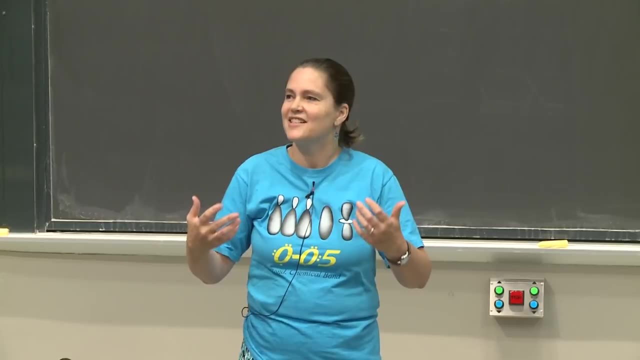 is what we're going to be doing. We're going to start on thermodynamics on Friday, And last night I had another dream about orbitals, So I think this is one more, some more orbitals, and then we go to thermodynamics. 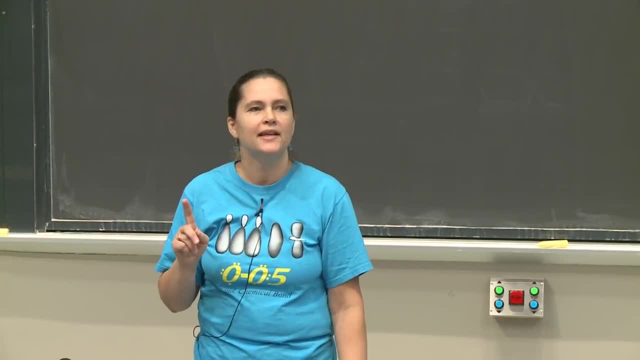 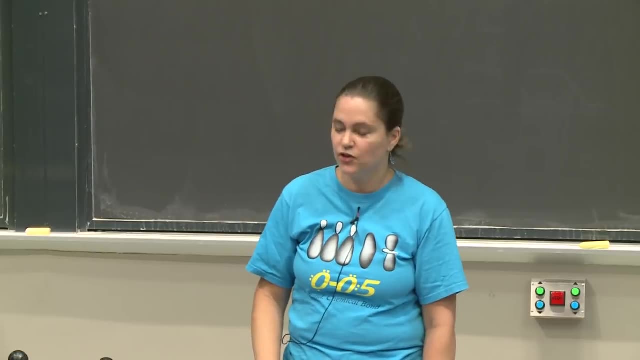 And I remembered my dream because at that moment my giant dog jumped on top of me as I was sleeping to wake me up and realize that thermodynamics needs to come pretty soon. OK, But one more, One more, One more theory. 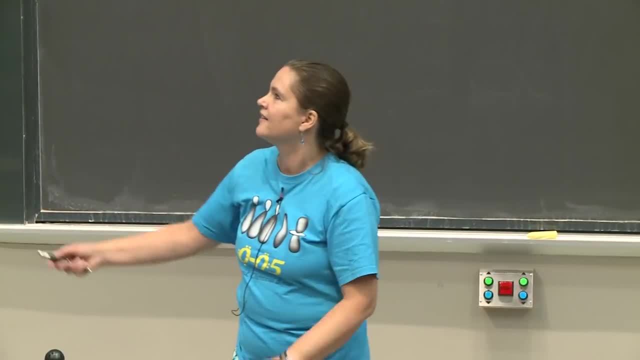 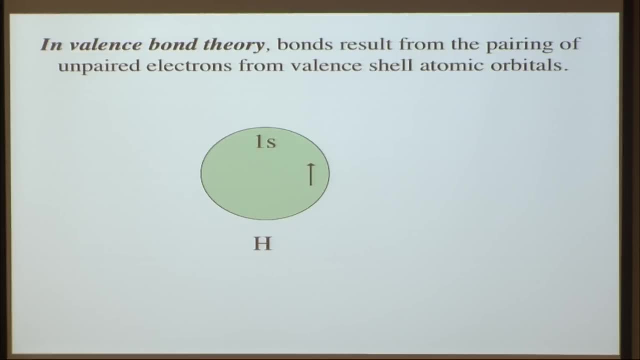 Valence bond. This is not so bad. OK. Bonds result from the pairing of unpaired electrons from the valence shell of atomic orbitals. That's it. That's it. So we have one, We bring in another, so we can make molecular hydrogen H2,. 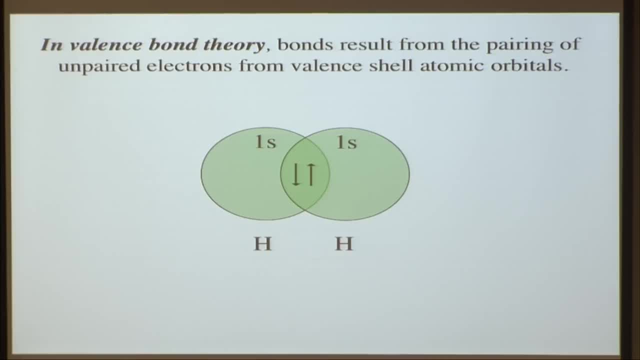 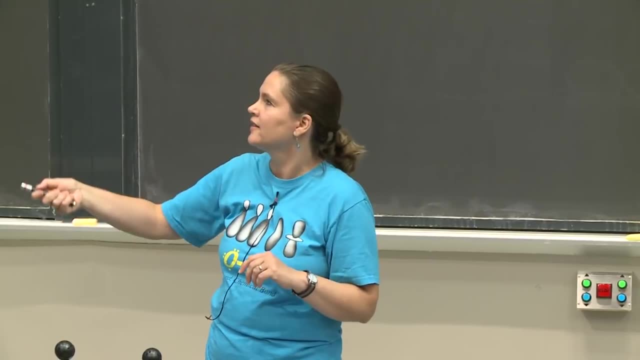 because they each have one unpaired electron and they come together to form a bond. I like this, So that's a good theory that you can say that you can put on a magnet in your refrigerator. That's a good theory to me. 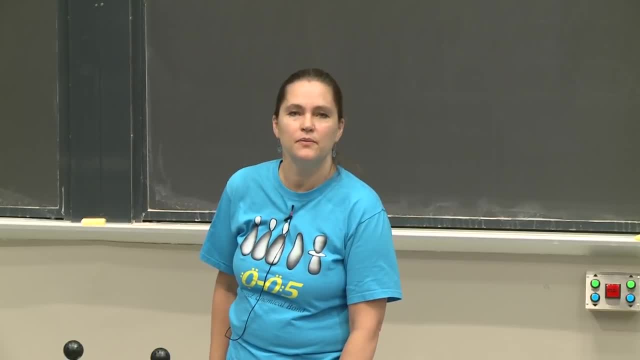 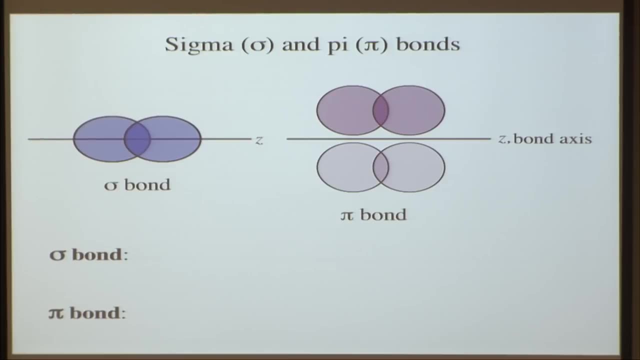 So also as part of valence bond theory, we have some names of bonds And we've been talking about sigma molecular orbitals and pi molecular orbitals And now we're going to talk about sigma bonds and pi bonds. So we had orbitals in MO theory. 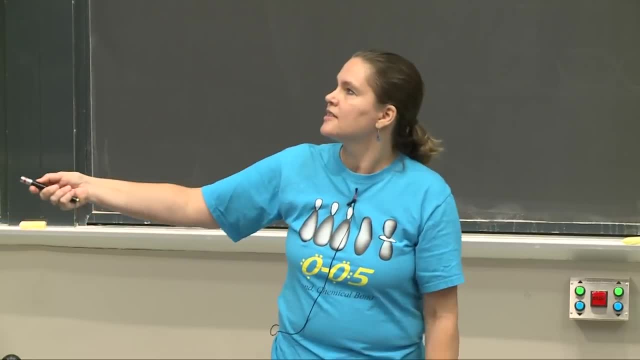 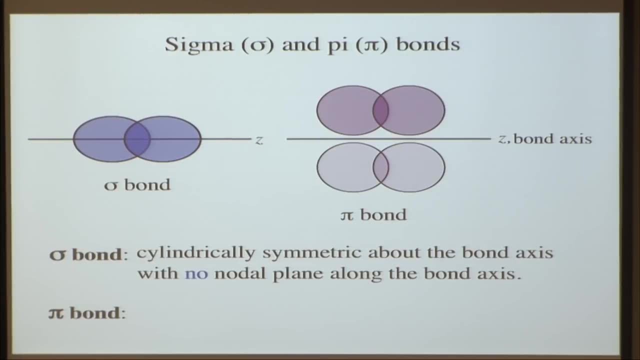 we now have bonds. Sigma orbital is cylindrically symmetric about the bonding axis. Thank goodness they didn't define them differently. that would have been a nightmare. So we have sigma orbitals that are cylindrically symmetrical about the bond axis, and sigma bonds are cylindrically symmetrical about the bond. 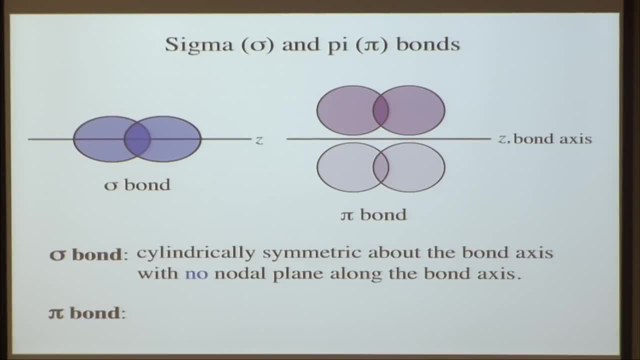 axis. So no nodal plane along the bond axis. Good, We should be able to remember that. So with pi bonds we have electron density in two lobes with a single nodal plane along the bond axis. So again with pi orbitals. 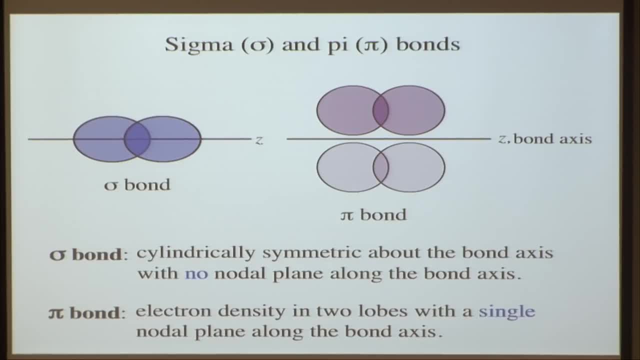 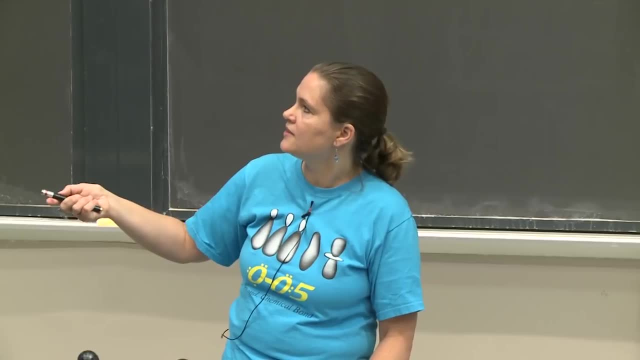 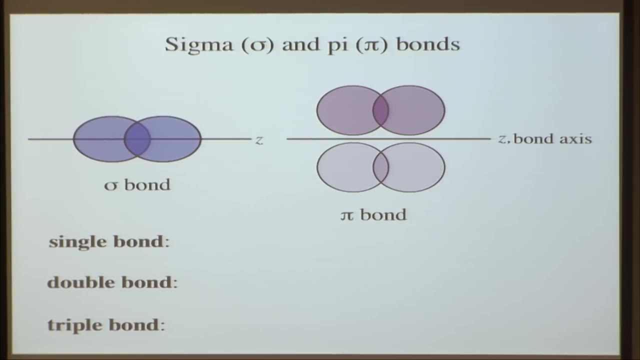 we had more, it wasn't cylindrically symmetric. So this we should be able to remember. A couple other things about sigma bonds and pi orbitals. Sigma bonds are not cylindrically symmetrical, They're not pi bonds. A single bond is a sigma bond, So when there's one bond it's a sigma. 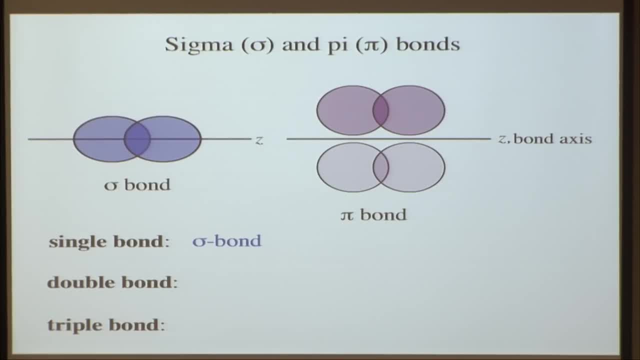 bond. So what's a double bond? A double bond is a sigma bond plus one pi bond. So it's got, if it's a double bond, it's got two types of bonds: sigma and pi. And what do you think a triple bond is? 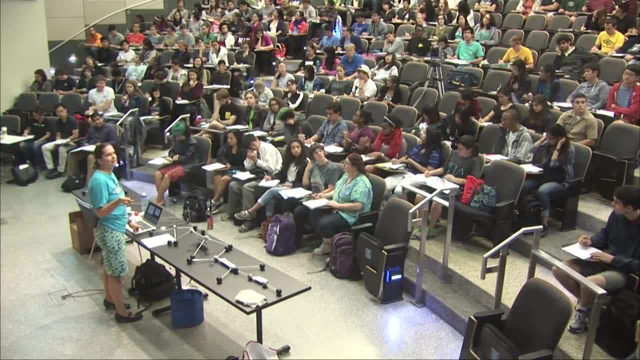 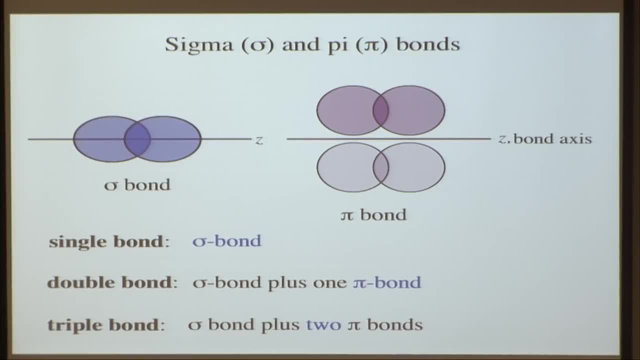 Sigma bond and two pi bonds. So you've got a triple bond like nitrogen, You've got two pi's. It's really a good life when you have a triple bond. All right, Single bonds always going to be sigma, double sigma and pi, triple sigma and two pi bonds. 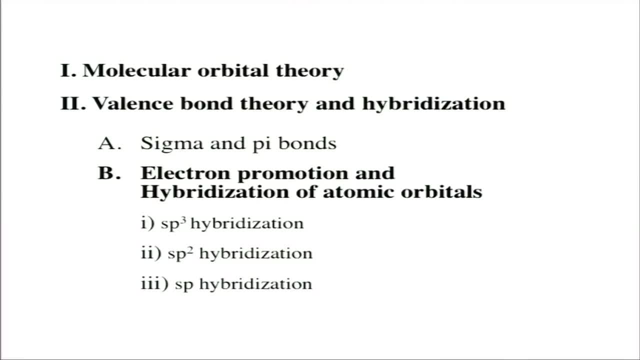 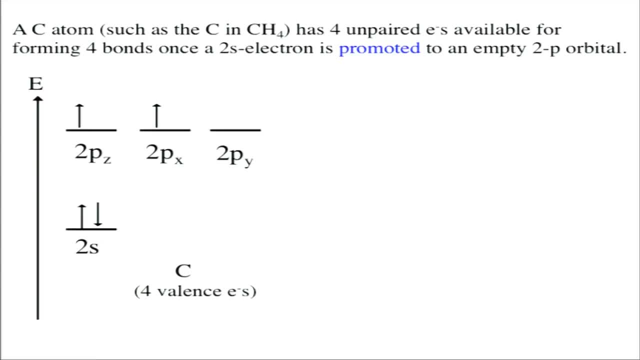 So now we're going to hybridize our orbitals And we're going to talk about electron promotion as well. So I start with carbon, carbon-based life. Carbon is really important, And if you are an organic chemist- and by organic it means studying things with carbon- you care a lot. 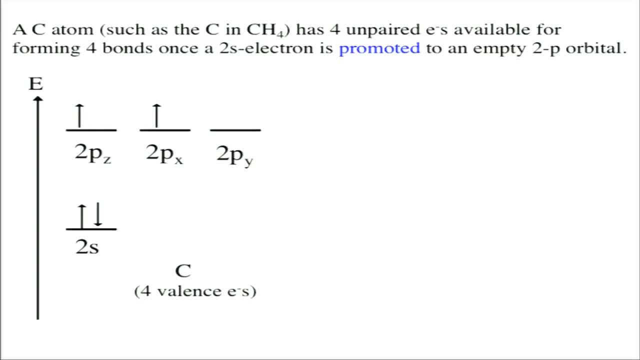 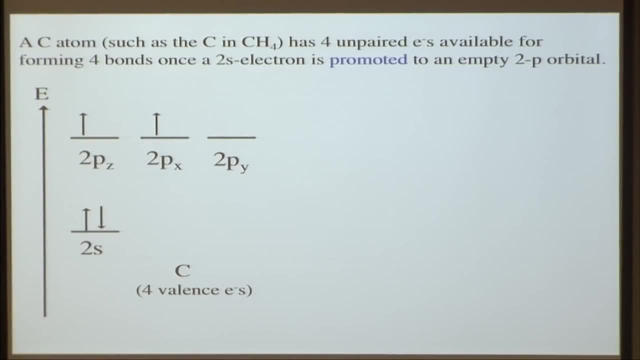 about hybridization And the stuff I'm teaching you today. you'll see a lot if you go on to take organic chemistry 512. So a carbon such as one in methane. So we have our methane molecule here. The carbon has four unpaired. 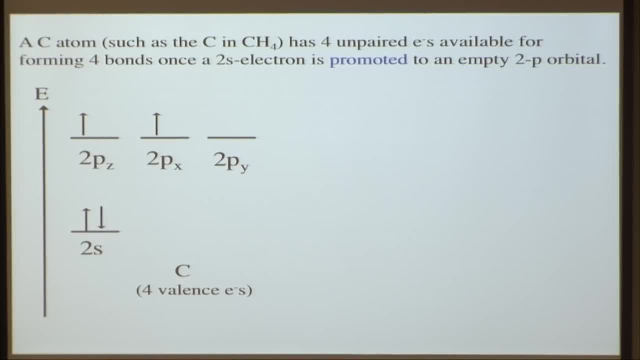 It can form bonds with four electrons, But to do so we need to do something with our electrons. So carbon comes in. It has two electrons and it's 2s, And it has two electrons and its two p's t orbitals. But we want to form four bonds And in valence, bond theory. 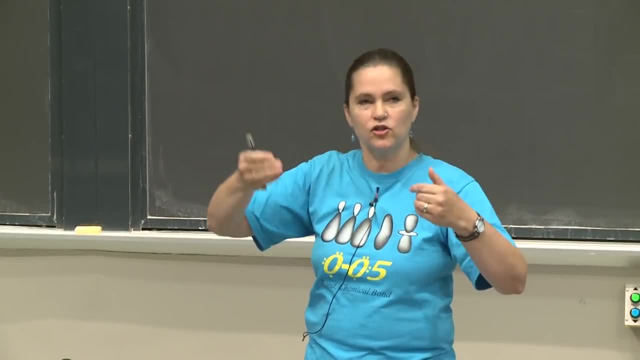 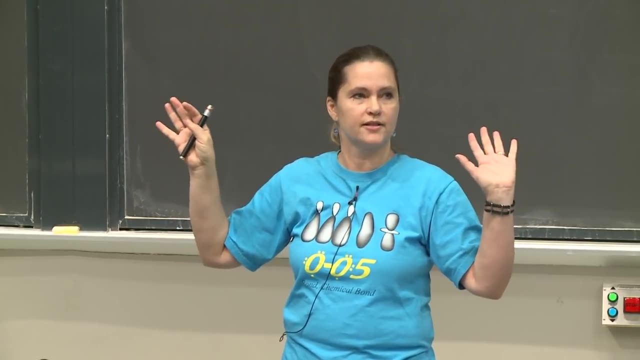 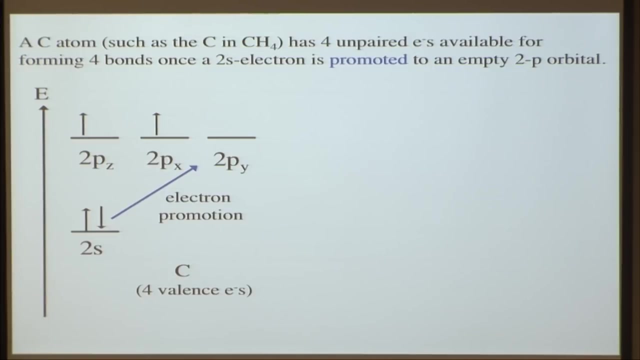 every bond. you bring an electron from one atom, an electron from the other And they pair And that forms a bond. So we don't have four single bonds or four unpaired electrons to make four bonds with this configuration of electrons. So we can talk about promotion of an electron from here up there. 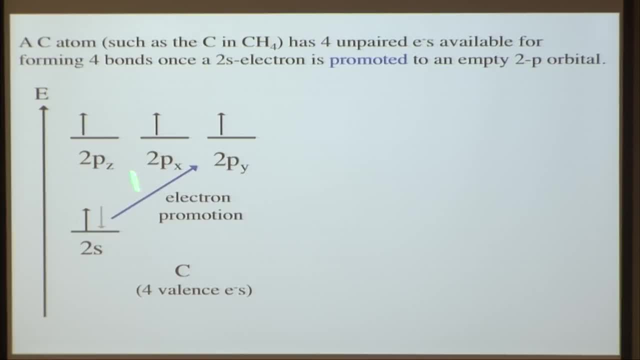 And if we do that now we have our four single unpaired electrons ready to make four bonds. And carbon does like to make four bonds, It does it quite often. So that's electron promotion To form those four bonds. a 2s electron is promoted to an empty 2p orbital. 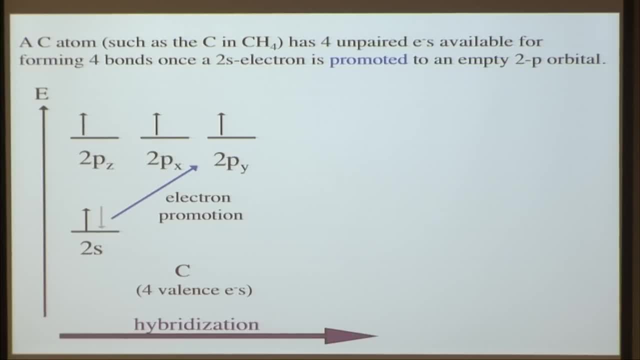 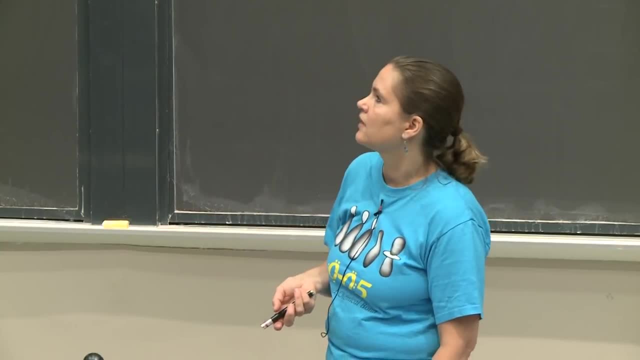 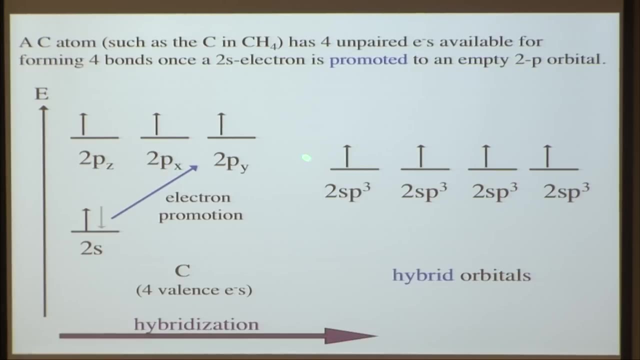 And then we can hybridize our orbitals, And that means that we want to give all our orbitals some s and some p character. So here are our hybrid orbitals And let me show you the nomenclature. So we're talking about n equals 2.. 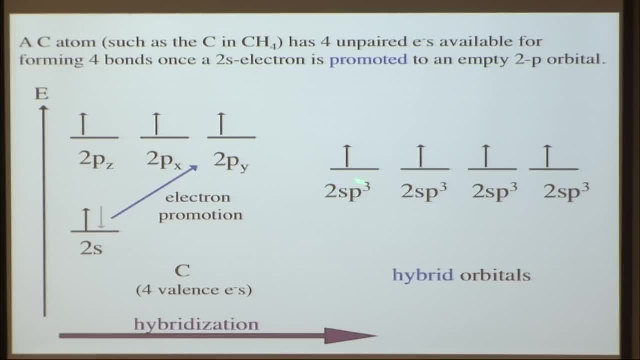 So we have a 2. We have s character And we have p character And we're using three p orbitals to make our hybrid orbitals. So we're going to make a 2sp3 hybrid orbital And we're going to make four of them, because we've used four atomic orbitals to make them. 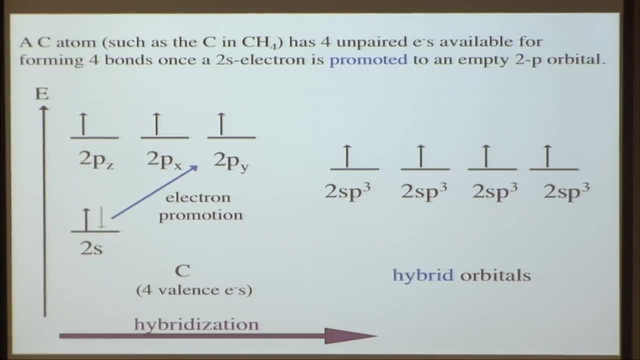 So if we are using four, we need to make four. So let's kind of take a look at what's going on here And I'll say that these molecular orbitals differ only in terms of the number of unpaired electrons. They differ only in terms of their orientation in space. 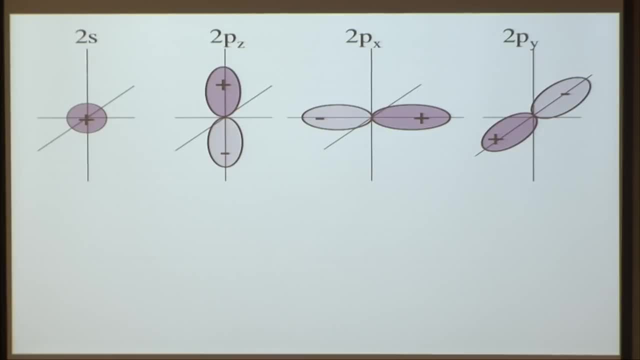 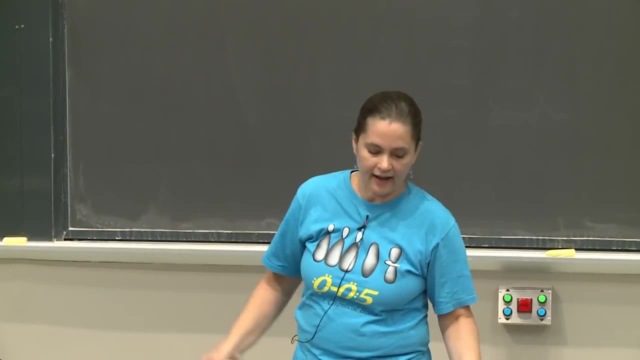 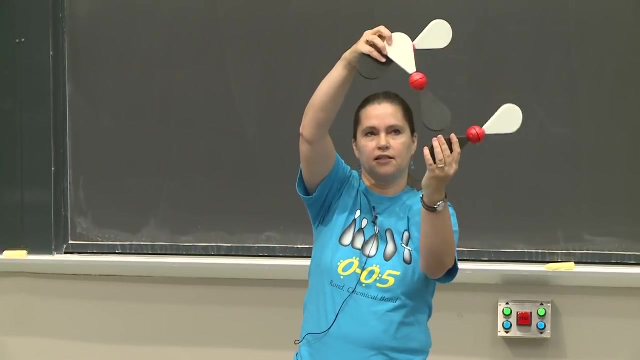 So they don't have different shapes, They're just oriented differently. So here we have our 2s- remember, It's symmetric- And we have our three p orbitals, And they're all the same, except that they're all oriented differently in space. 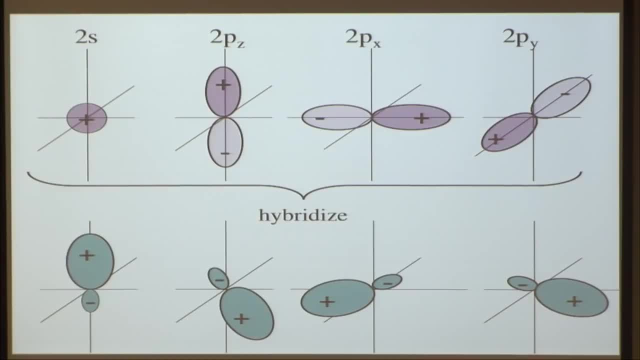 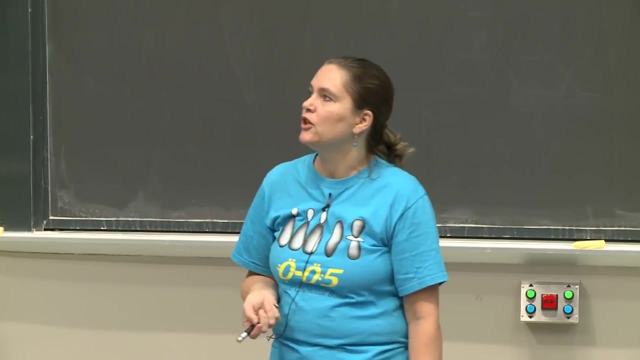 And when we bring these together we form four hybrid orbitals And they kind of look the same. They're not going to look like turtles, but they're turtles oriented differently in space, But otherwise they're the same. So those are our sp3 hybridized orbitals. 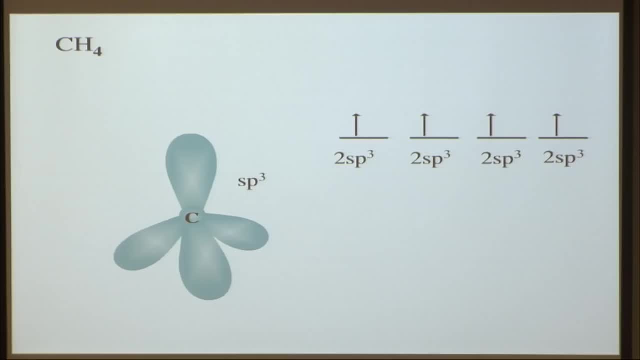 So carbon has this sp3 hybridized orbital And it has four unpaired electrons available to form bonds with four hydrogens. So let's bring our hydrogens in to form our bonds, And each hydrogen brings with it its one electron, So now we have two electrons in all four of our hybrid orbitals. 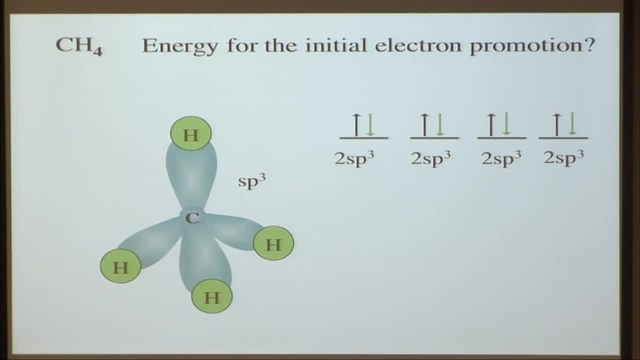 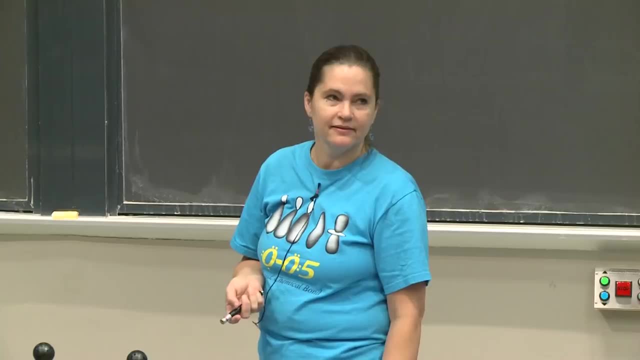 And we can think about where the energy came from. I just moved that electron and think about it. I'm like, yeah, that just goes up here. So where did the energy come from To do that? And that is, it came from bonding. 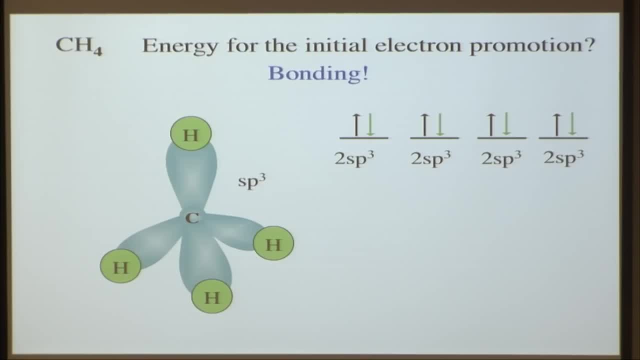 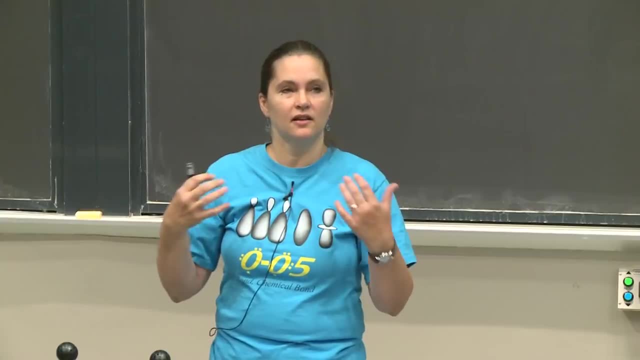 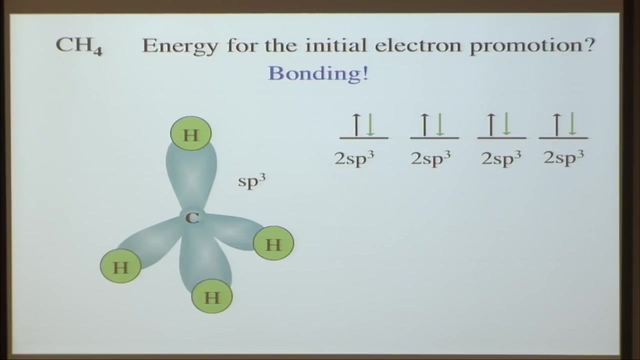 So this molecule now is more stable because it's bonded. Methane is quite a stable molecule. That's another problem in and of itself, So the bonding allows you to do that. You get back from this bonding. So let's look at those bonds then that are formed, that make 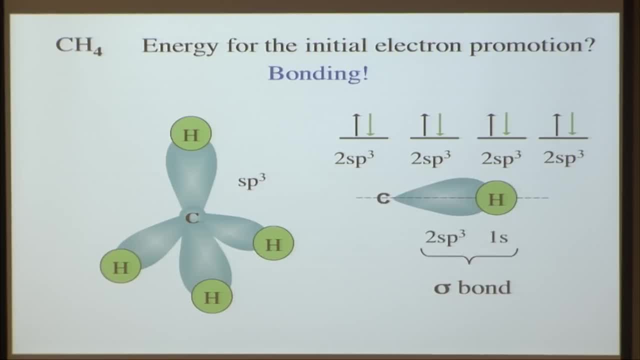 that electron promotion worthwhile. And so you're forming a bond between the carbon and the hydrogen, And so you're going to have a bond which you're going to form and the hydrogen. you're forming four of them And you're forming single bonds. 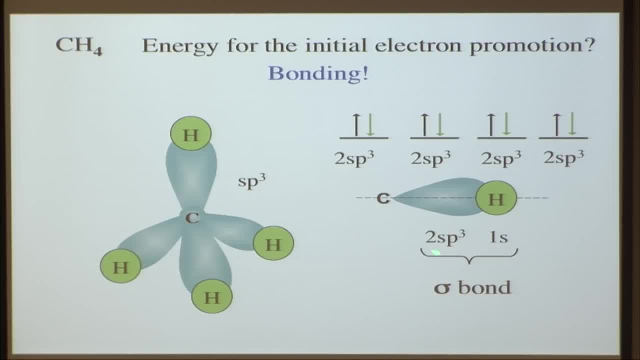 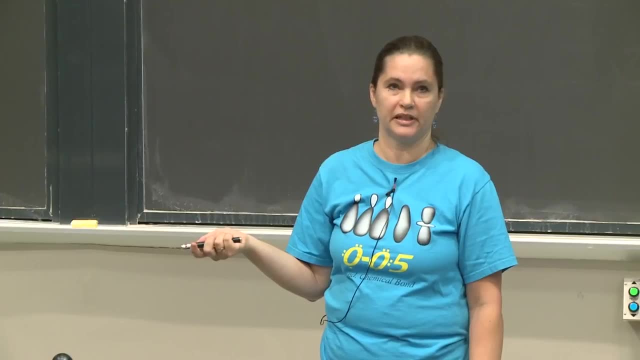 They're sigma bonds And the bond is formed between the carbon's 2sp3 orbital and the hydrogen's 1s orbital. Hydrogen can't hybridize, It's got one 1s orbital. That's all it's got. 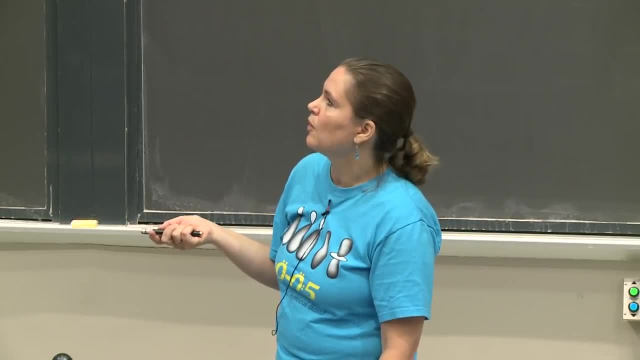 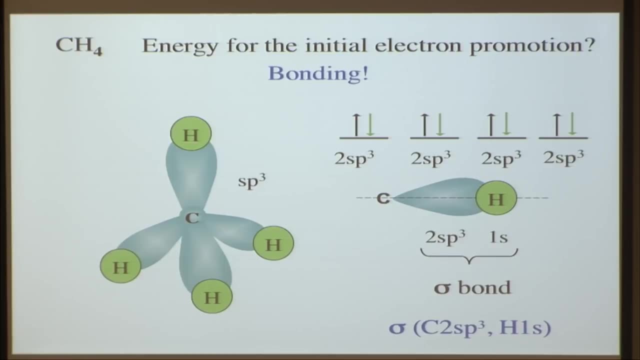 Can't do anything else, And that gives you a bond, then a sigma bond that you'll see this a lot And you'll write this a lot. This is how we're going to name that sigma bond. So we're going to say sigma. 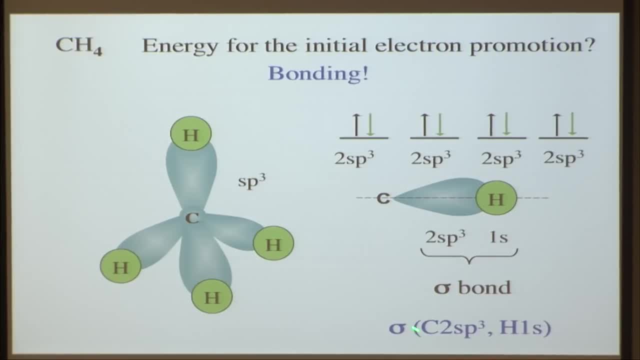 We're going to have a parentheses. Identify the element. It's carbon. n is 2.. Type of orbital: sp3, comma- hydrogen, the name of the other element and its orbital, which is 1s. So when it asks you to name the type of bond, 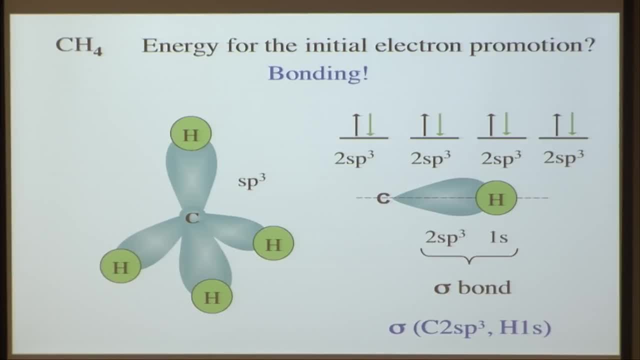 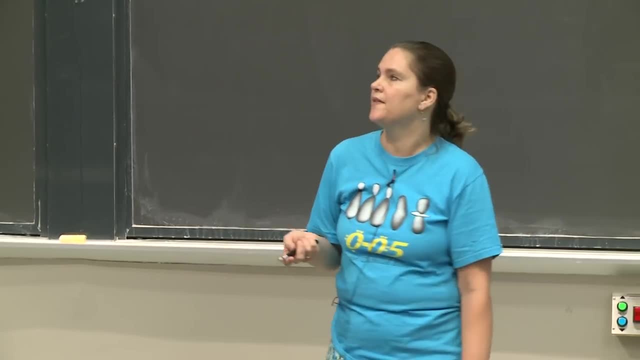 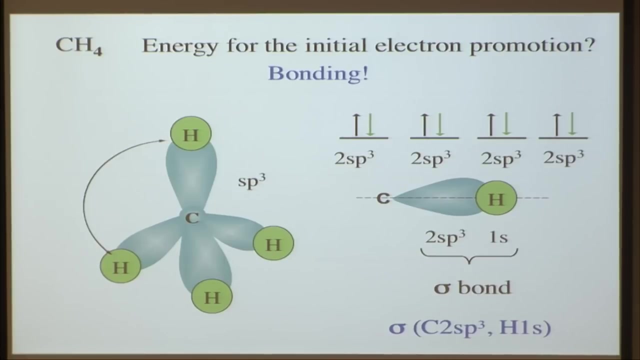 this is the complete answer. This is the complete answer that we're looking for, And we'll have more practice on this. Now. we can also think about the shape that this molecule would have. What is the angle here between this hydrogen and that hydrogen? 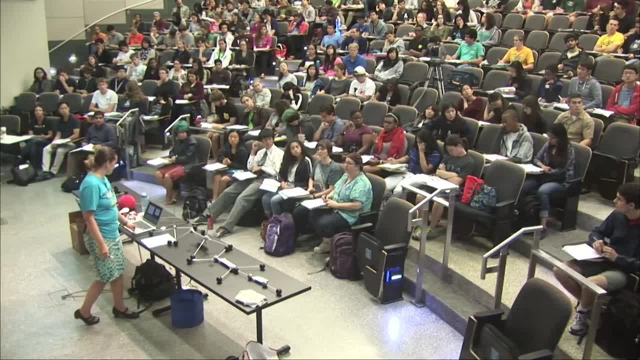 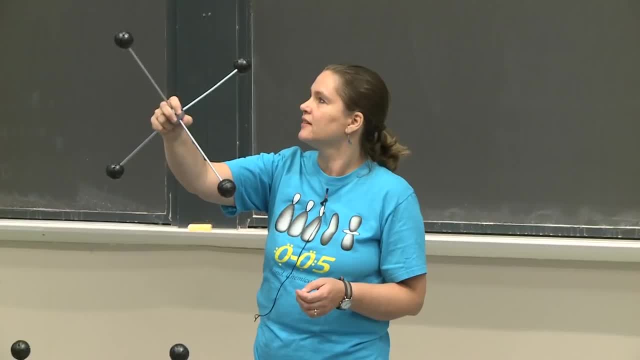 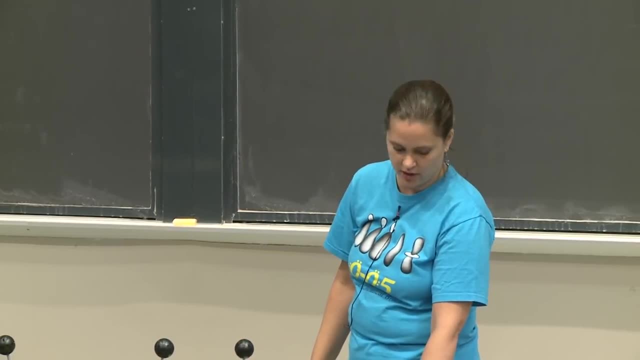 and, frankly, between any of the hydrogen carbon hydrogens, 109.5.. Yep, 109.5.. And the name of that geometry Tetrahedral. So sp3 gives you a tetrahedral geometry, a tetrahedral-based geometry here. 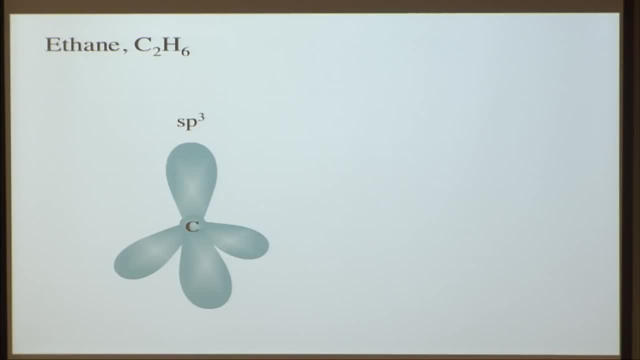 All right. so now let's get more complicated. Let's bring two carbons in, So we have ethane. two carbons, six hydrogens, So this also has its carbons are sp3.. And this is what we saw before for methane. 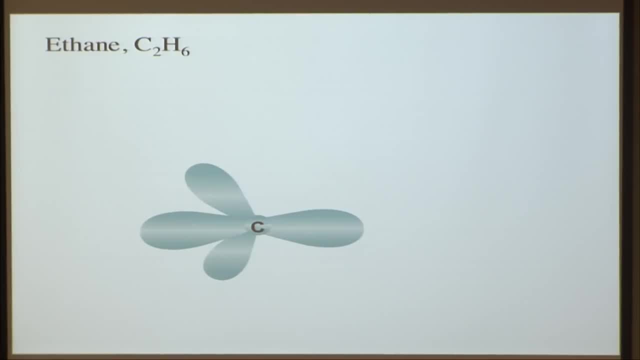 But now I'm going to rotate this around. And that's one carbon, But we need another carbon. But first we can think about this one carbon, So one of the carbons of ethane. it would have this 109.5 angle. 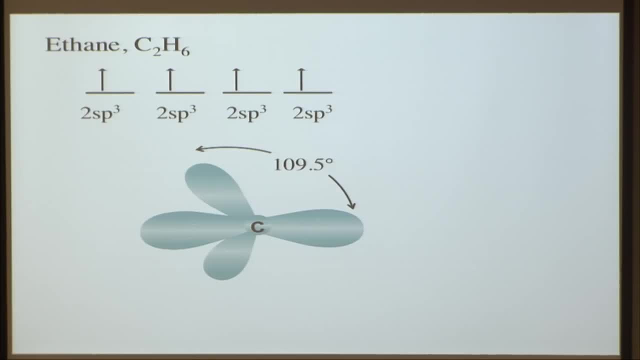 It has four unpaired electrons available And it's four hybrid orbitals to form interactions, one with carbon and three of them with hydrogen, And then we need another one of these, So we'll bring that in And it comes in with its set of hybrid orbitals. 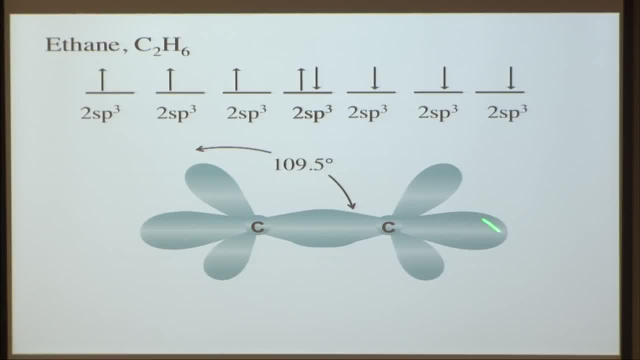 And it's set of electrons And we form a bond between them. And the bond we're going to form is a single bond, a sigma bond. And now let's bring in our hydrogens. So we had six hydrogens, three for each carbon. And so there are now two types of bonds. We have the carbon-carbon bond And we also have the carbon-hydrogen bond, And we have the carbon-hydrogen bonds And so the carbon-carbon bond, which is a sigma bond. 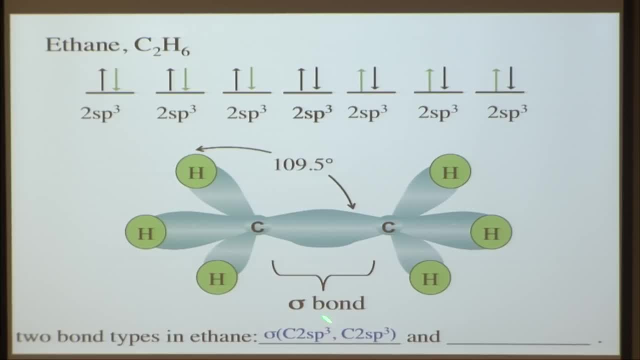 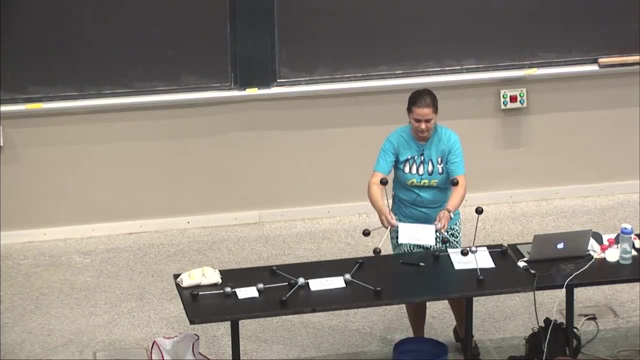 is sigma- parentheses- carbon. it has carbon to sp3, comma. the other carbon is the same carbon to sp3, and in the bracket. So that's that sigma bond, It's a single bond. And here is our ethane molecule. 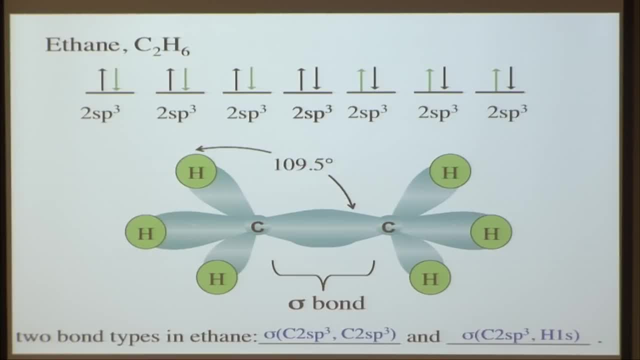 And then we have our carbon-hydrogen bond. They're also sigma. Please don't give me pi bonds to hydrogen. It only has that one electron. It's happy with two electrons. It doesn't want to do anything complicated. It doesn't have p orbitals, just that 1s. 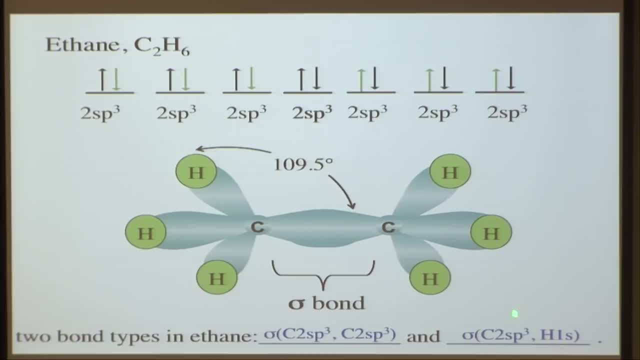 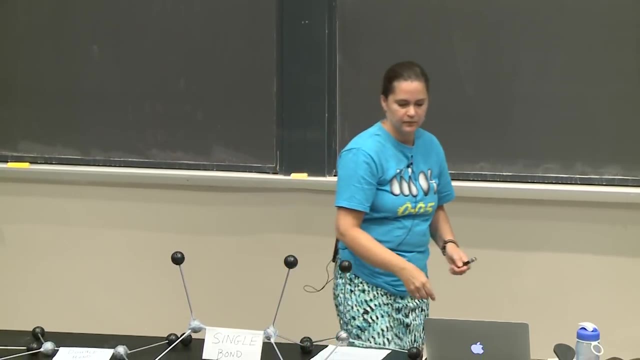 So sigma carbon 2,, sp3,, comma hydrogen 1s, And now we have defined this molecule. So we've bought together two tetrahedral centers and formed this molecule with a single bond. So let's talk about nitrogen. 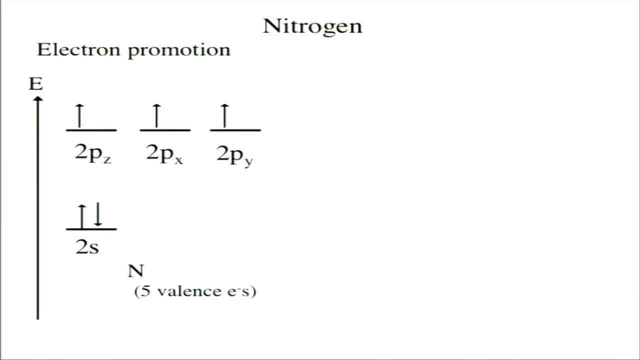 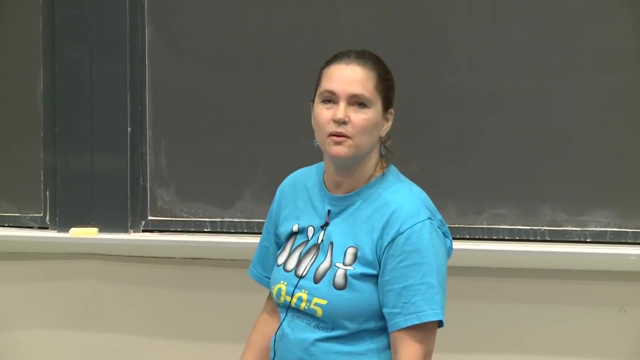 Nitrogen, also again very important. So here we have five valence electrons. What about electron promotion? Should I do it? No, Because I mean you could put it up here, but it can't make any more bonds. 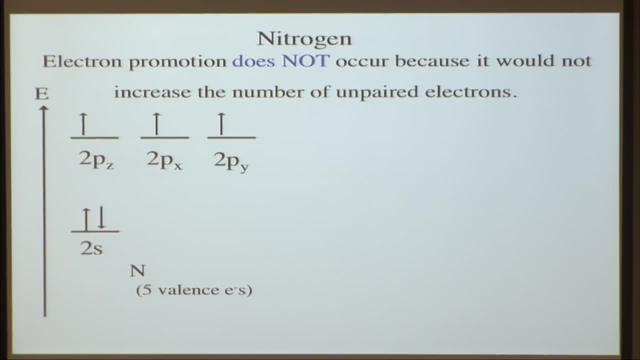 So it doesn't really matter, So it doesn't occur because it would not increase the number of unpaired electrons to form bonds. But we can hybridize. So we can still hybridize our orbitals And we can get four hybrid orbitals. 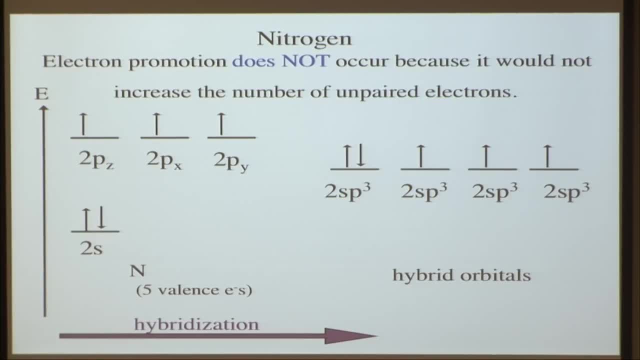 because we're going to use our 2s and all three of our 2p orbitals, So we'll get the same set of hybrid orbitals, But this time one of them has two electrons in it, So it's not ready to bond. 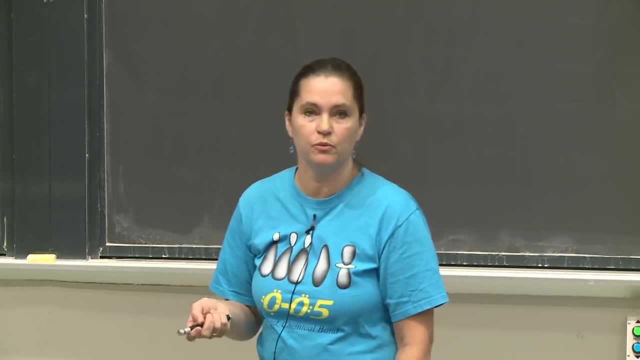 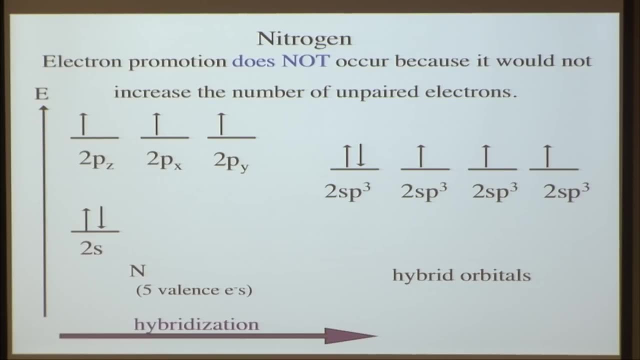 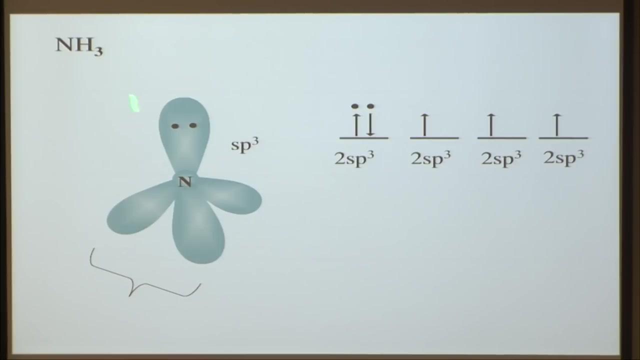 It's happy according to valence bond theory, And these are our lone pairs. But we can form three bonds with these. So let's look at an example: NH3.. So now we have our lone pair. It's in this orbital up here. 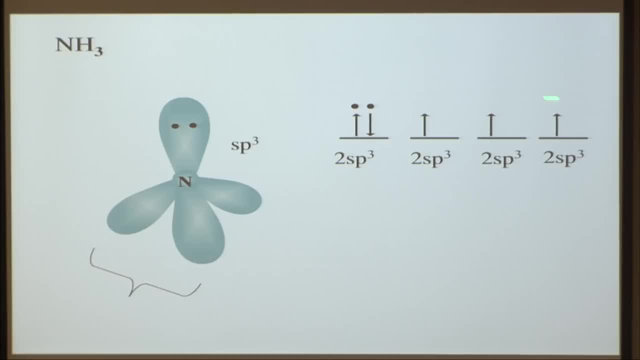 And then we have three orbitals available for bonding, each with an unpaired electron ready for the three atoms of hydrogen to come in. So we bring in our three atoms of hydrogen, Each came with an electron, And now you can tell me with a clock. 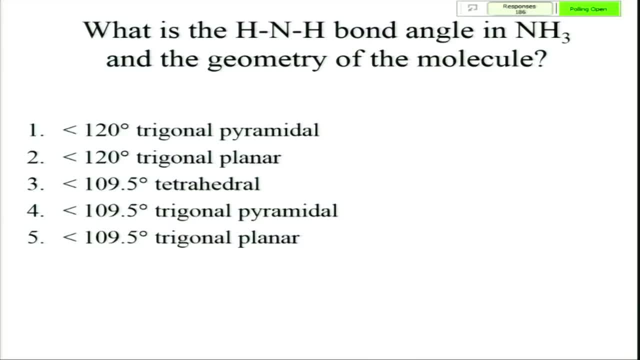 with a clicker about the angle and the geometry of this molecule. All right, Let's just do 10 more seconds. All right. so this is back to VSEPR again. So we have an angle here. It's based on an SN4 system: one lone pair, three bonded atoms. 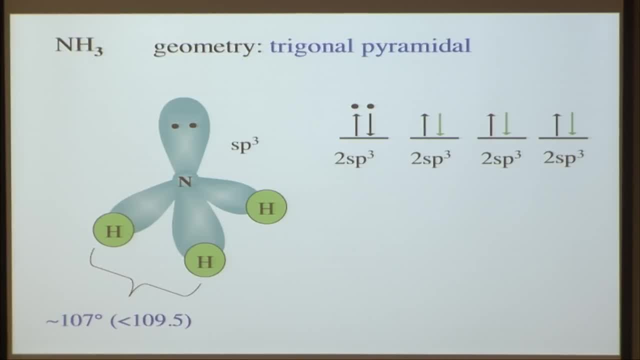 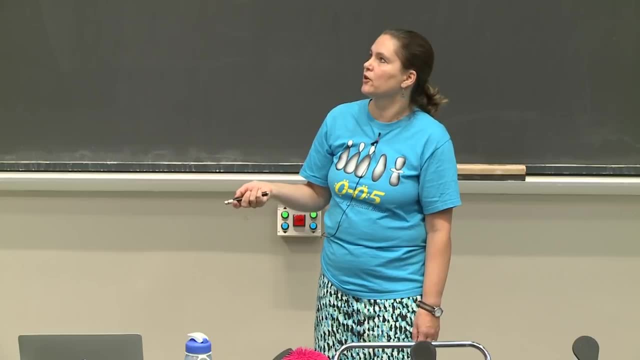 So it's based on our 109.5.. But those lone pairs make for bad roommates And they're pressing all of these hydrogen together, And so the angle is less than 109.5.. And we name this structure based on the atoms. 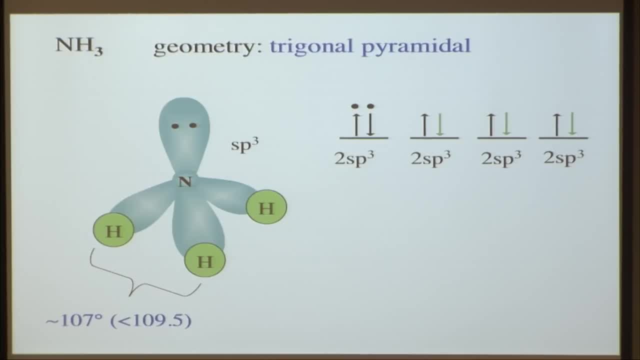 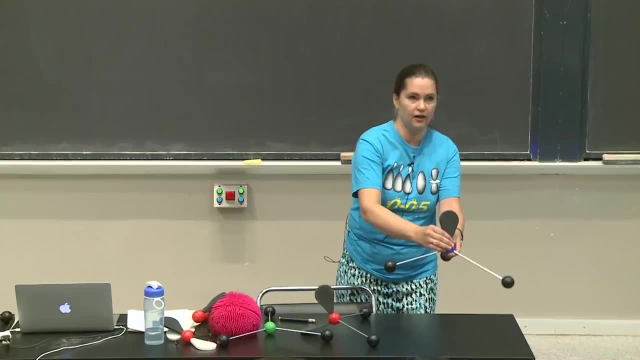 we see, not the lone pairs. So this is trigonal pyramidal, And so here we have it here. So we're naming it without thinking about the position of those lone pairs that are pressing down on the bond. So it looks trigonal, like a triangle. 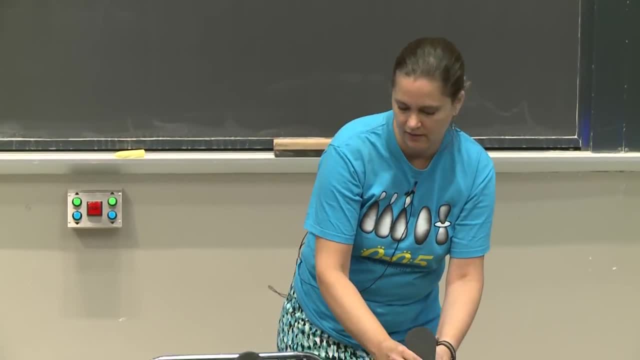 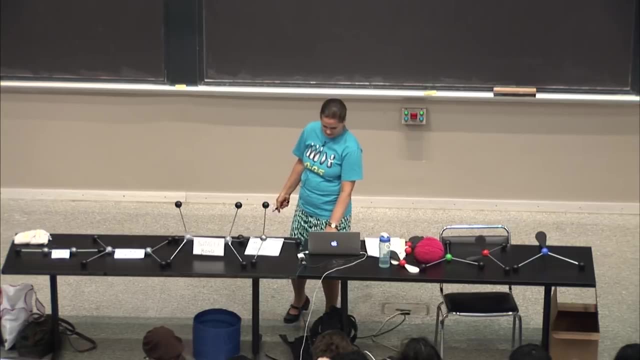 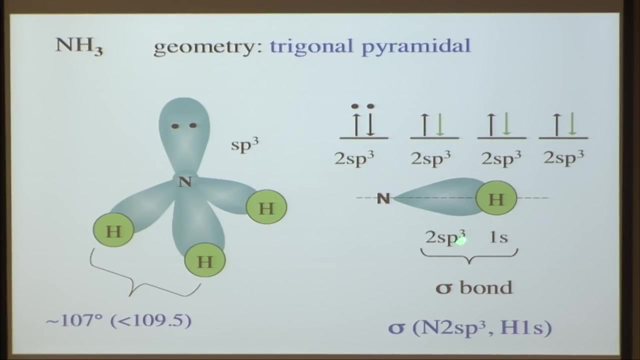 but it's also a little pyramid. so VSEPR, VSEPR and hybridization, they just go right together. It's awesome, OK, So we can also name the type of bond. So our nitrogen had 2sp3 hybridization. 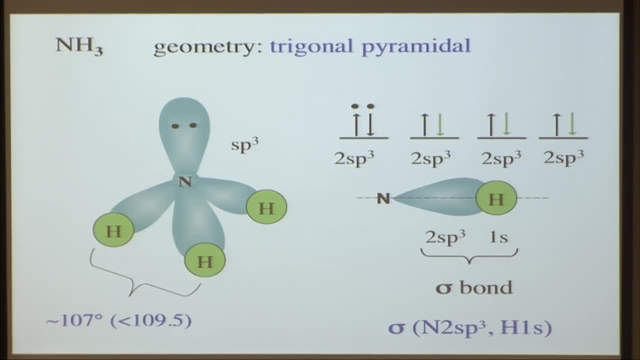 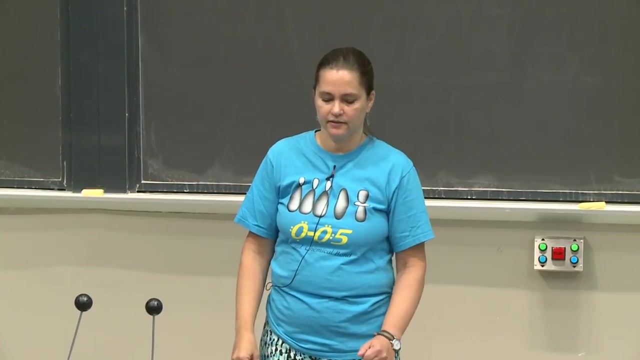 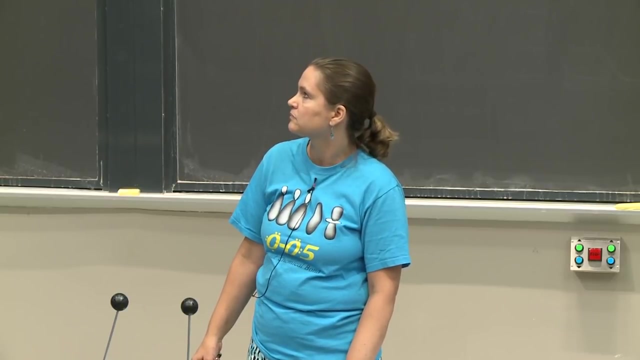 And our hydrogen just 1s. It's a sigma bond, It's a single bond, So we name that sigma nitrogen, 2sp3 comma h1s, So nitrogen. Now we're going to go back to oxygen and think about hybridization of oxygen. 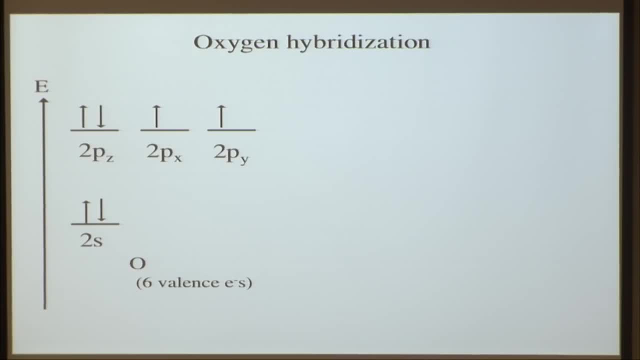 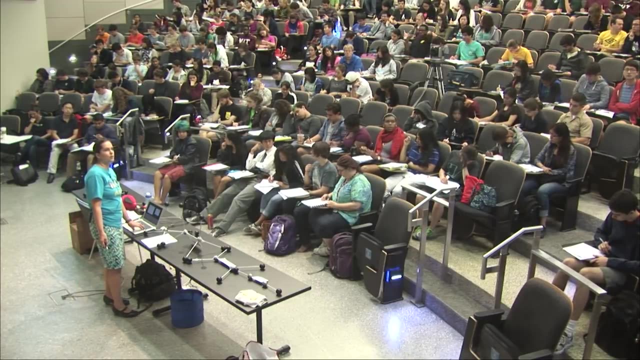 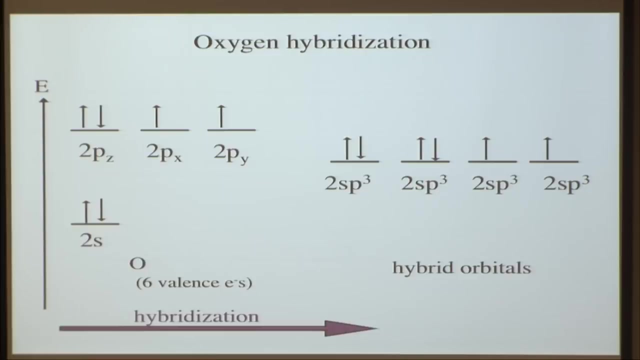 Oxygen. Should I do an electron promotion? No, It's not going to help me. It's not going to create any more electrons available to form bonds. But I can hybridize And I can get the same, for hybrid orbitals are for 2sp3. 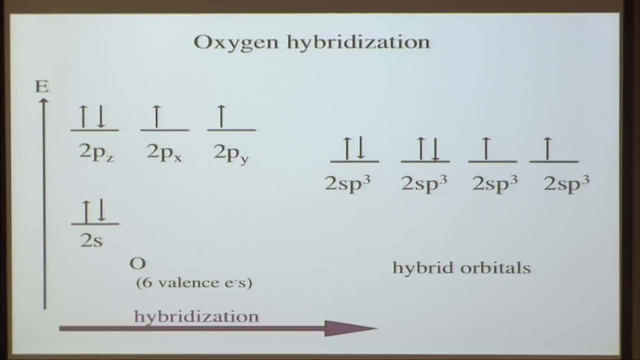 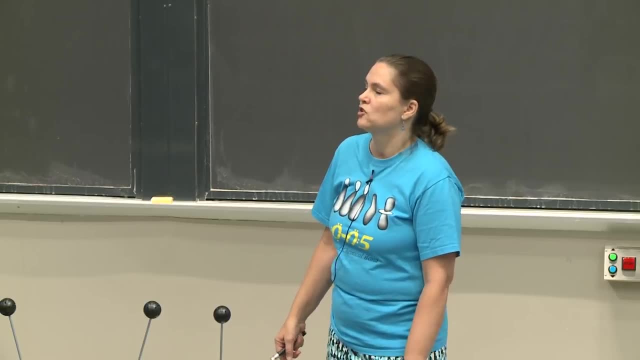 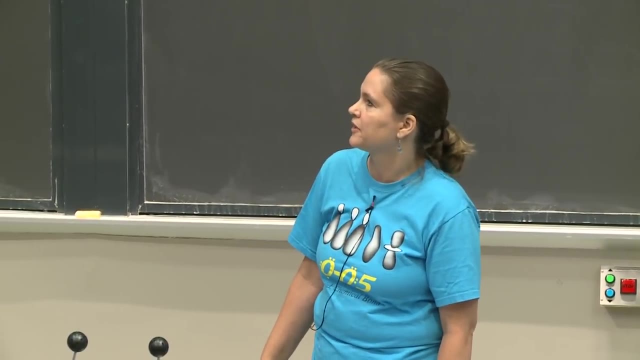 orbitals, But now two of them have two electrons in them and two are available to form bonds. Oxygen loves to form bonds with hydrogen and form water. Most of the planet is water. There's a lot of water, and water is really important for life. 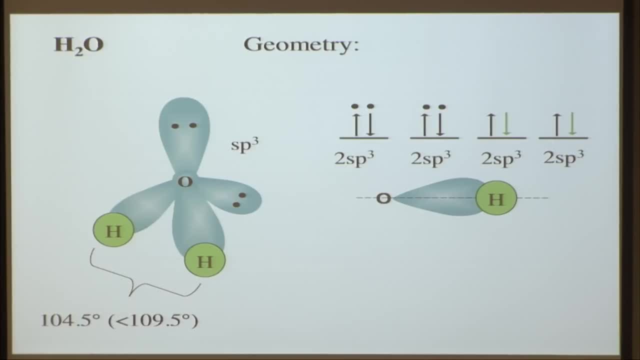 So it's great that oxygen and hydrogen get along so well. So the oxygen again has two lone pairs which are here. You bring in our hydrogens and they come with one electron, And again now it's still a steric number of four systems. 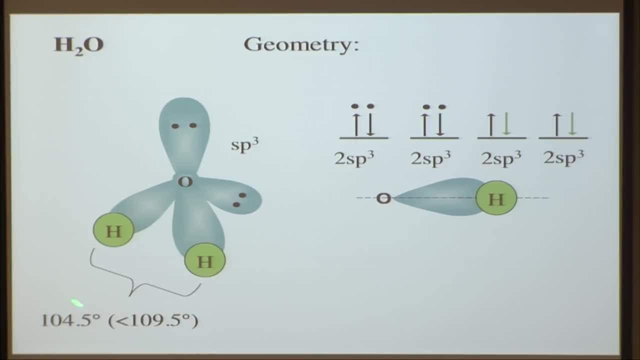 So it's less than 109.5.. And it's actually a lot less than the nitrogen, because you have those two lone pairs that are just taking up so much room and squeezing together these hydrogen atoms over here, creating this 104.5 angle. 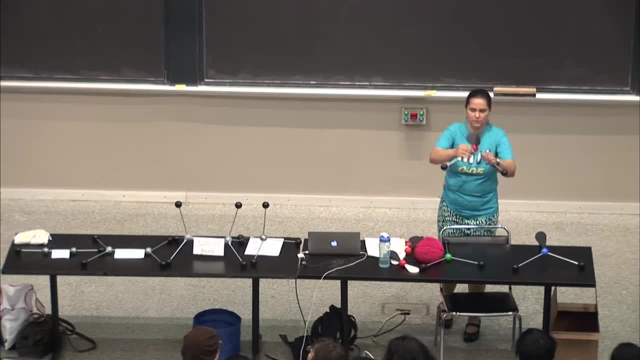 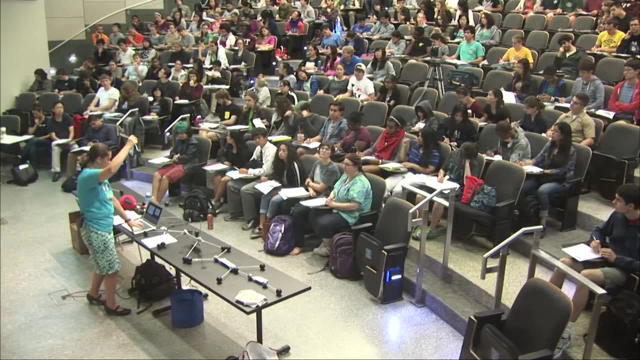 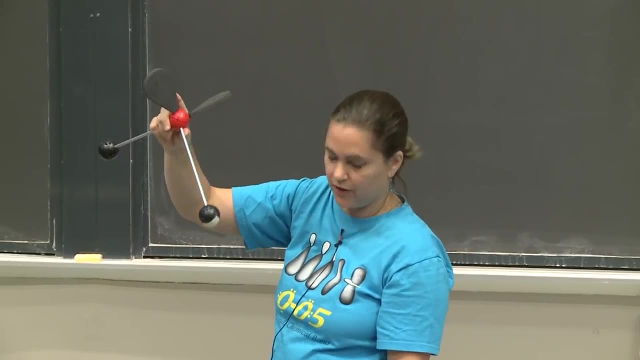 And so here we have our oxygen molecule with its two lone pairs and its two hydrogens, And what's the name of that? geometry Bent. And again we have these polar bonds that create a dipole. So it's a polar molecule which is very important in life. 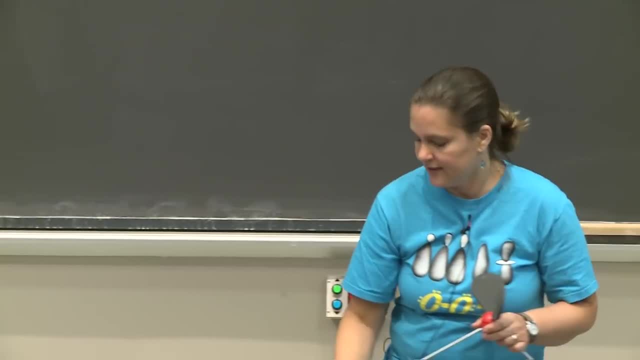 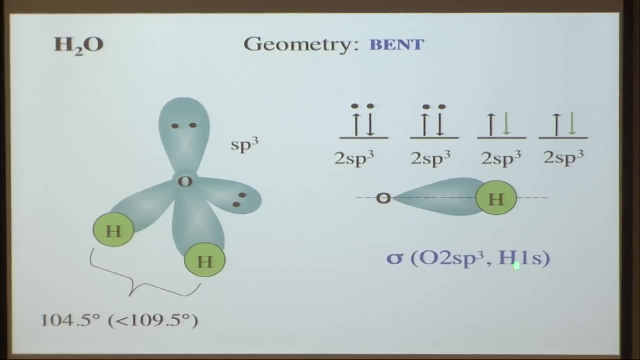 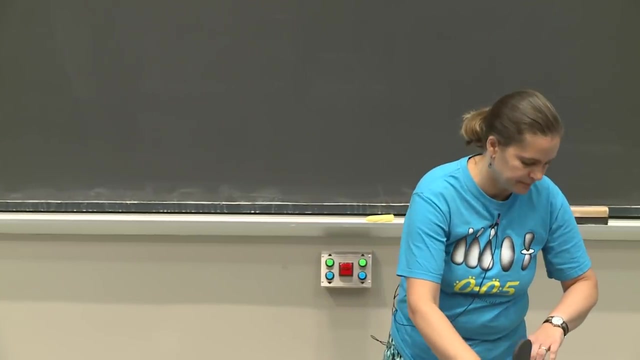 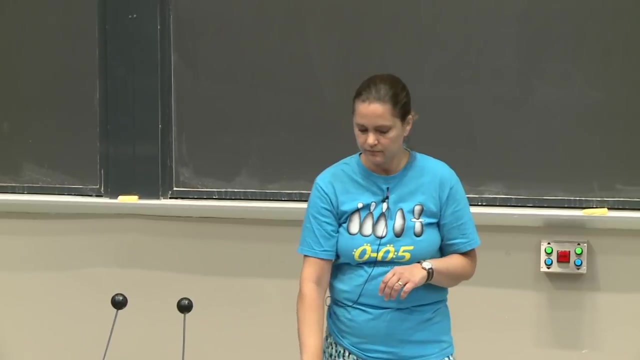 And we can name that bond. It's a sigma bond. It's made up of oxygen, O2sp3, comma H1s. All right, so that's sp3.. Hybridization: Now let's talk about sp2 hybridization. So sp2 hybridization. 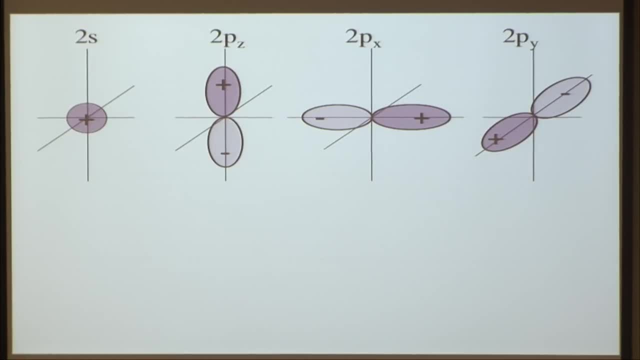 So back to our atomic orbitals. And now we're not going to hybridize all of our orbitals, We're just going to hybridize our 2s and two of our p orbitals. So we'll hybridize these guys And we will form three hybrid orbitals. 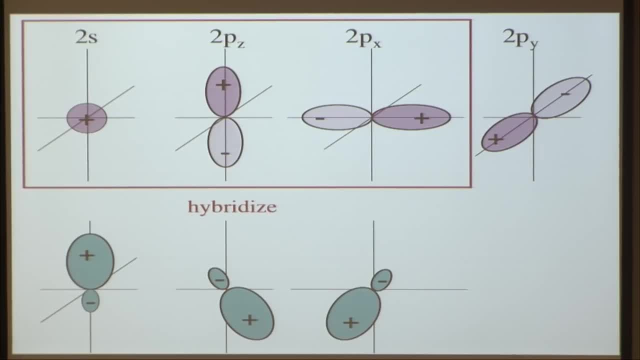 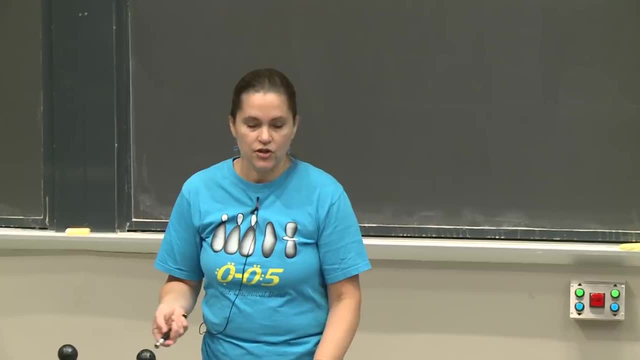 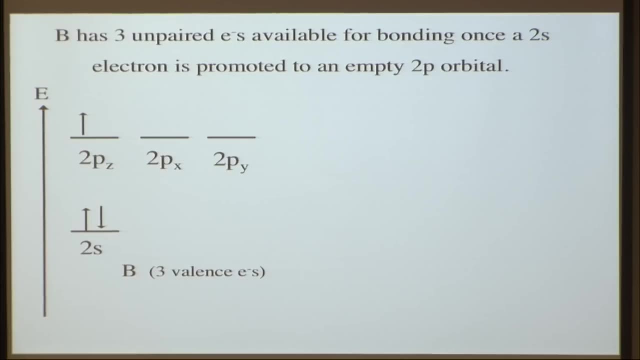 And we will still have one unhybridized orbital. We will have 2py left alone. So let's see what this does. How is this hybridization useful? So let's talk about boron. Boron has three unpaired electrons, but they are not. 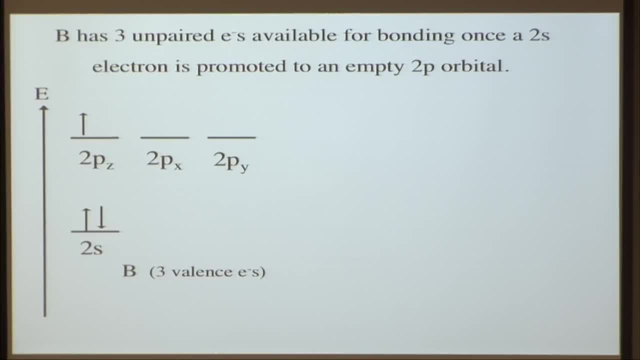 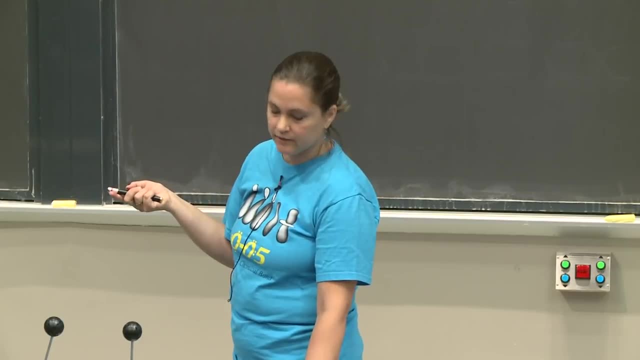 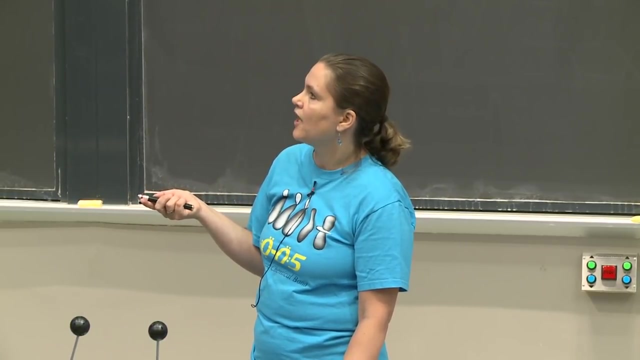 available. They are still available right now to form bonds according to valence bond theory. So here we do want to do an electron promotion to put one of them up here, so that now all three are available to form bonds And we can again hybridize these three atomic orbitals. 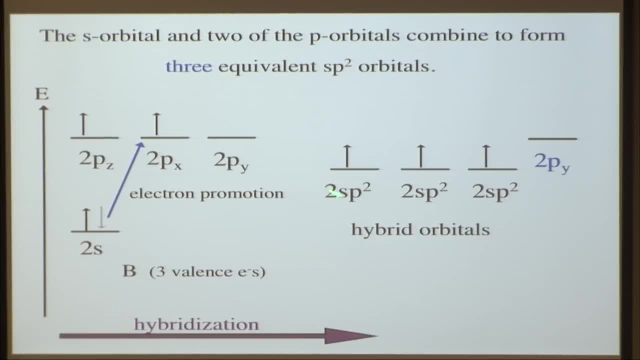 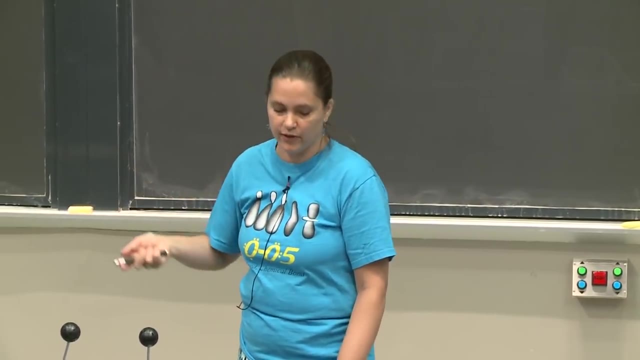 and form three hybrid orbitals. So we have three 2sp2 hybrid orbitals And we still have r2py orbitals, So don't forget to mark it. It seems lonely, It's over here, but it's going to be important later. 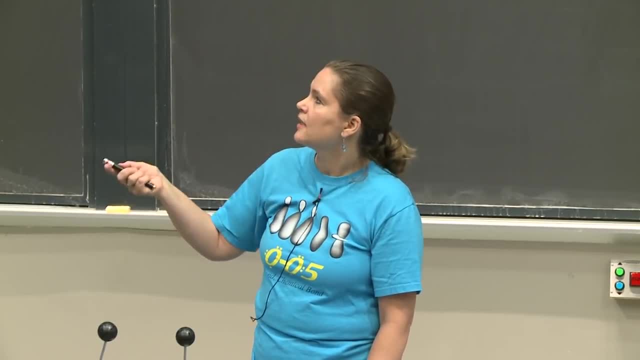 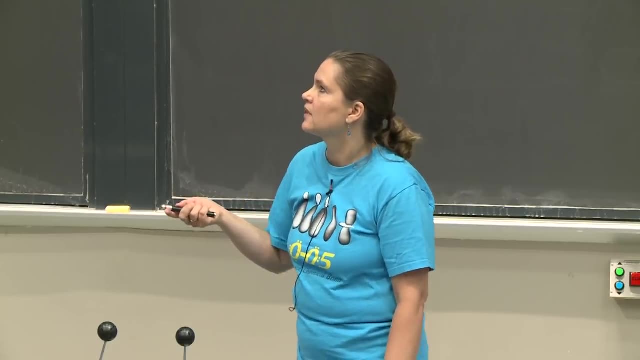 So don't feel bad for it yet. All right, so boron, Let's think about these hybrid orbitals and how this gives us the structure that we know occurs when we have boron. So boron now has its three sp2 orbitals. 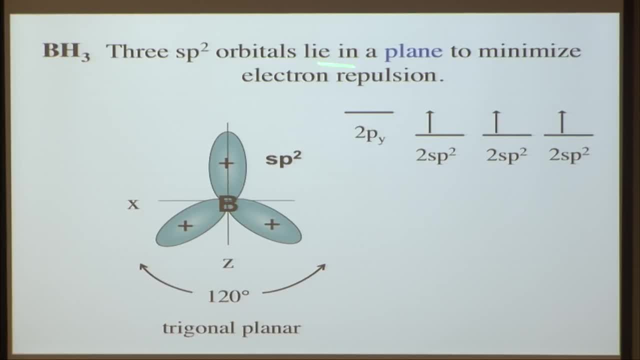 And these are going to lie in a plane And they're going to be as far apart as they can to minimize electron repulsion. And if you're in a plane then you need the far part as you could be is 120 degrees. 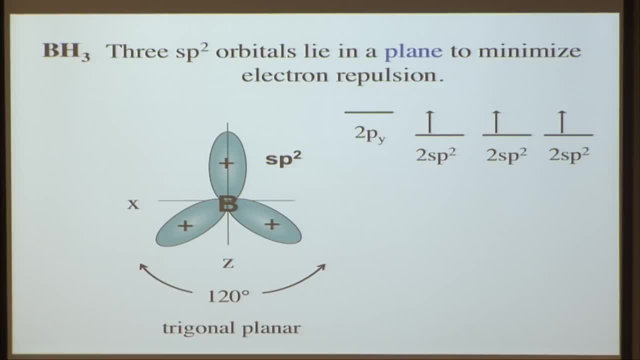 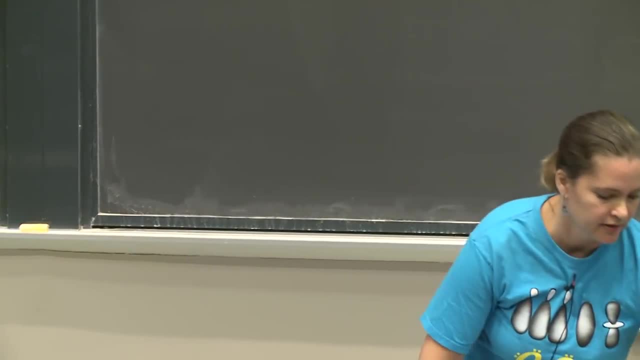 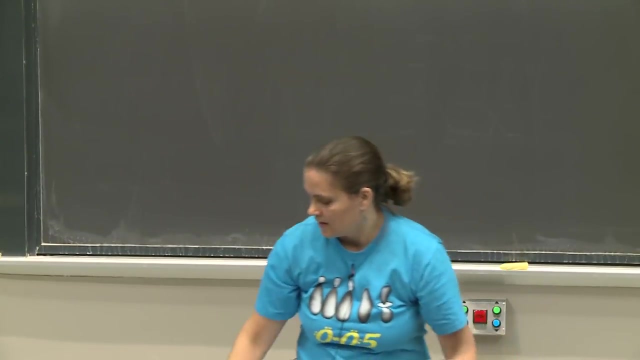 And this is what gives us our trigonal planar geometry. So we saw that boron formed these trigonal planar complexes before And again. they're trigonal planar because they're like a triangle And they're in a plane- trigonal planar. 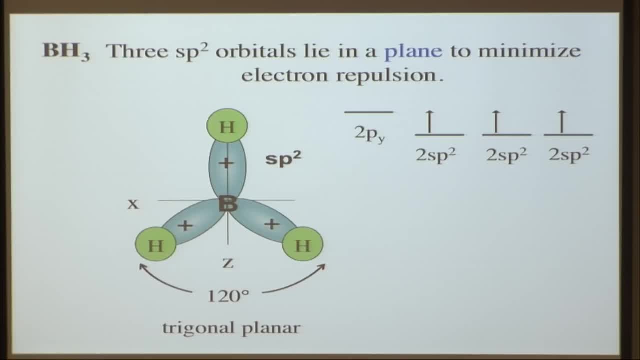 And we can now bring in our hydrogen. The hydrogens come with an electron, So we have an electron for them, And there we have our structure. We can also name that bond. So again we have single bonds. So sigma B for boron 2, sp2, comma H1s. 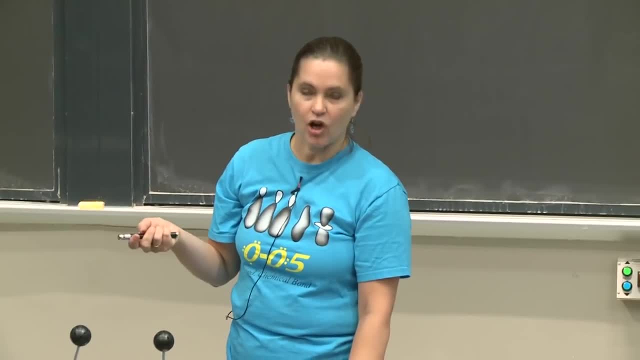 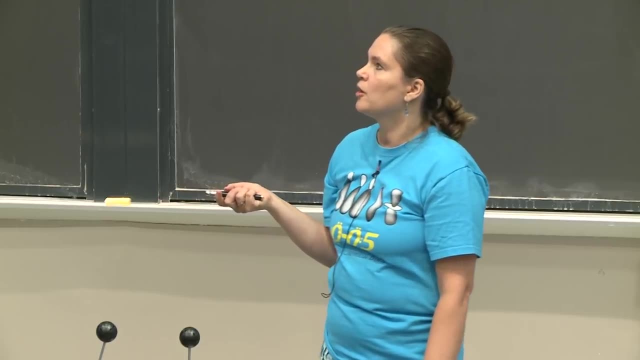 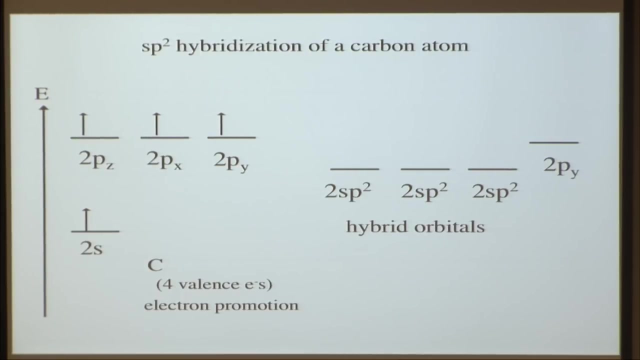 And there are three of those. Carbon Carbon can also do this. We talked about carbon being sp3.. Carbon can also be sp2, hybridized Carbon is amazing. That's why life is based on carbon. Carbon can do lots of things. 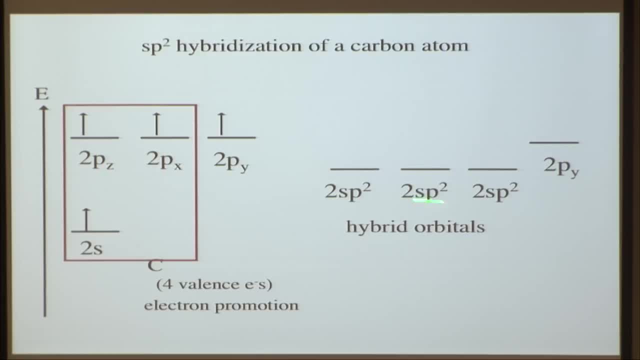 So again, we're going to hybridize two p orbitals, one s orbital, to give three hybrid orbitals, And we have our 2py over here in the corner. But don't feel bad for it, It's going to do something useful. 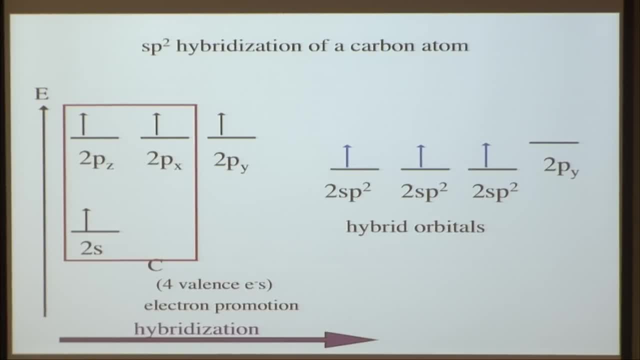 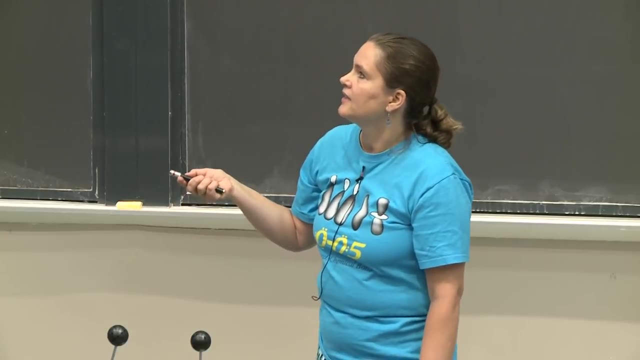 So we now have three electrons in these hybrids. So we have three hybrid orbitals, And now we have one electron in our 2py unhybridized orbital as well. So let's see what carbon, with this kind of arrangement of orbitals, can do. 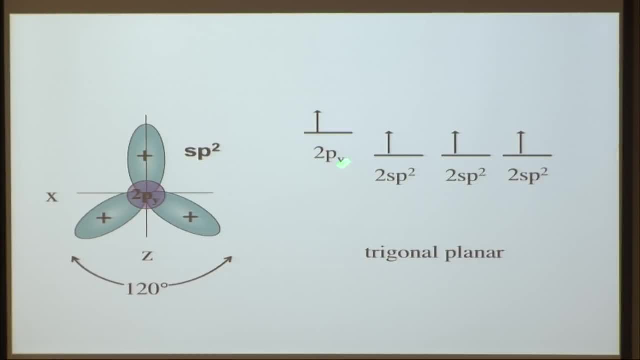 And again, we're going to have trigonal planar geometry for our two sp2 hybrid orbitals. So we have carbon there And these are all in a plane. But now, coming out of the plane toward us, we have a 2py orbital. 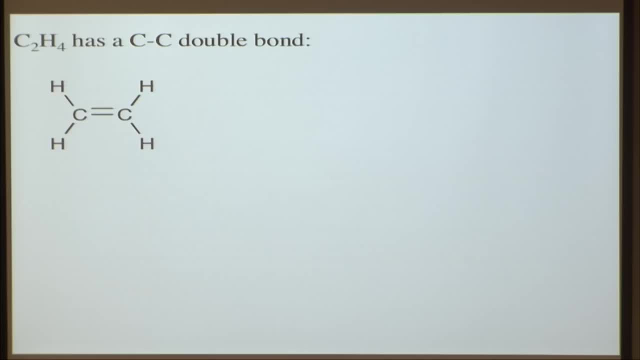 So it's coming out 90 degrees away from the trigonal planar geometry. So an example of sp2 hybridization is in this molecule, C2H4.. And it has a double bond, which means if it's a double bond, 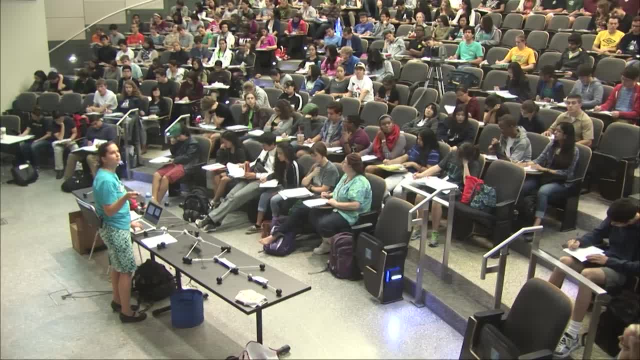 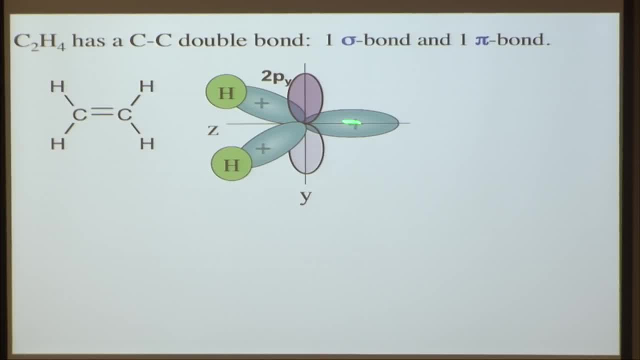 it has what kind of bonds in it: Sigma and pi. So one sigma, one pi bond. Now, and this is the trigonal planar geometry. It's supposed to be in a plane, But you can't really see it. if it's really in a plane, 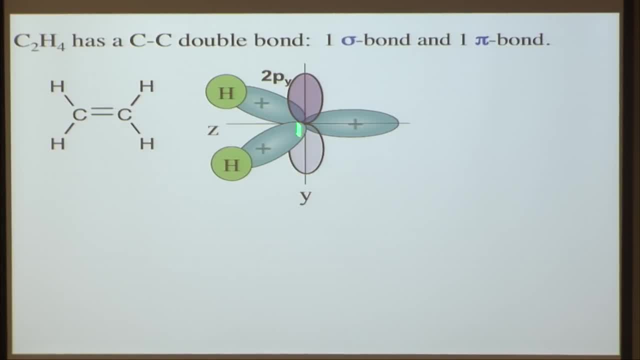 But 90 degrees away from that plane is our 2py orbital. We brought in our two hydrogens. So this is this: carbon here. Carbon is there. Two hydrogens are there. This would be 120 degrees. Now we're going to bring in another one. 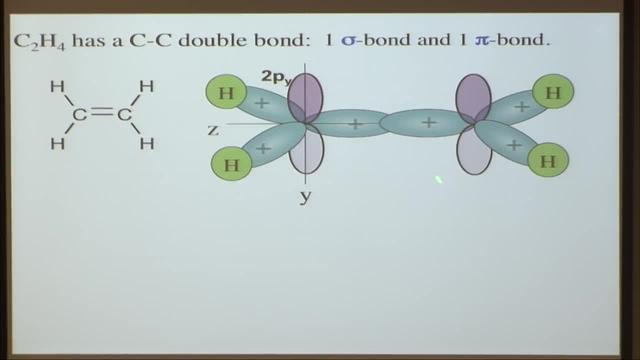 That's the one over here. It comes in with its carbon. It comes in with its two hydrogens, forming these single bonds. These are the bonds between the carbon and those hydrogens, And now we're going to form a carbon-carbon bond. 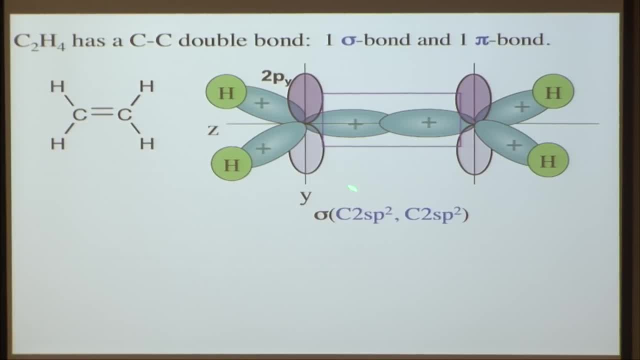 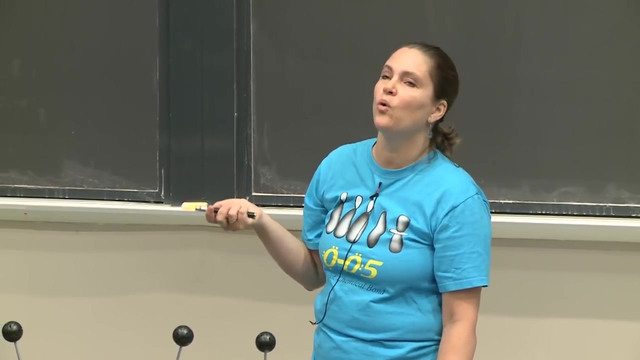 This carbon-carbon bond is a sigma bond, And so it's C2sp2 comma C2sp2.. But we're not done. We said this is a double bond. So that's our sigma bond, But we need our pi bond. 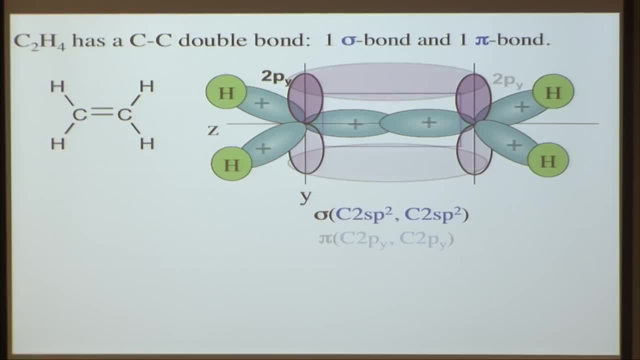 And now py, our unhybridized orbital, is excited because it can form the pi bond. So we form a pi bond And that's formed by our C2py comma, C2py unhybridized orbital. And we also have four CH bonds. 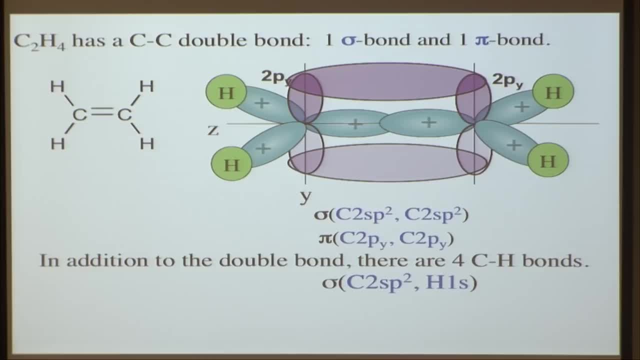 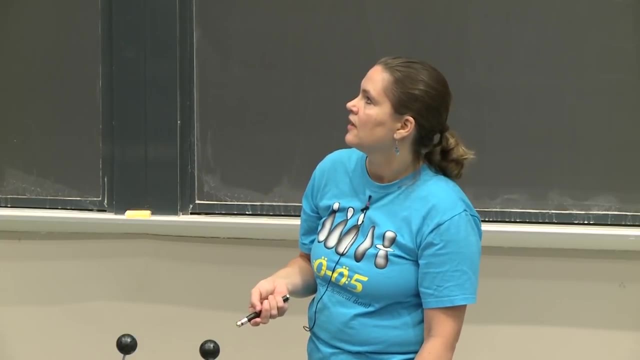 And those are single bonds, Those are sigma bonds, And so they're formed by our C2sp2, carbon And hydrogen 1s, And there are four of those. So that's an example of sp2 hybridization And one thing that's very important. 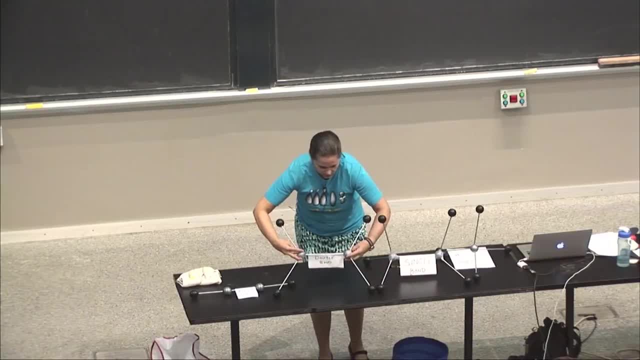 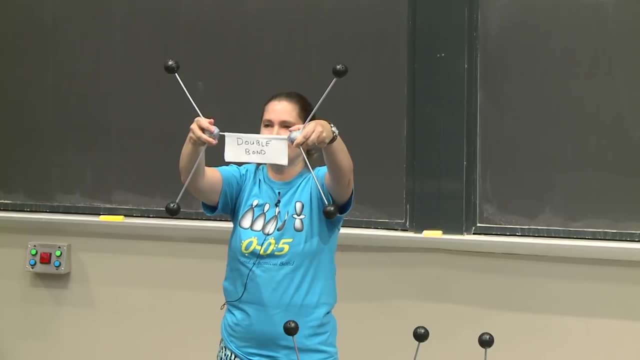 and here you can see what that molecule looks like. It doesn't all fall apart. So this is a double bond, These molecules don't let me make double bonds. So I have a sign, double bond, And you can see the angles and the geometry of this molecule. 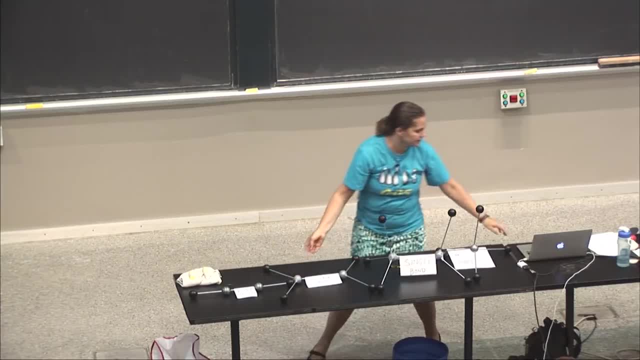 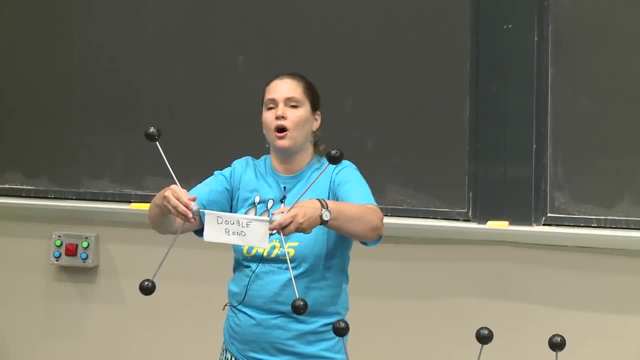 And another property of something with a double bond like this Is that it's not really free to rotate. So when you have these two kind of points of attachment, when you have these orbitals forming between your unhybridized p orbitals, 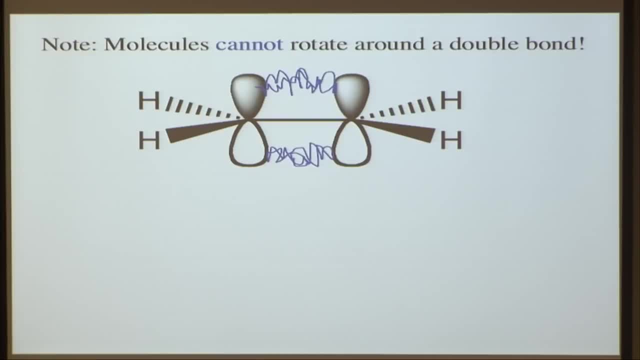 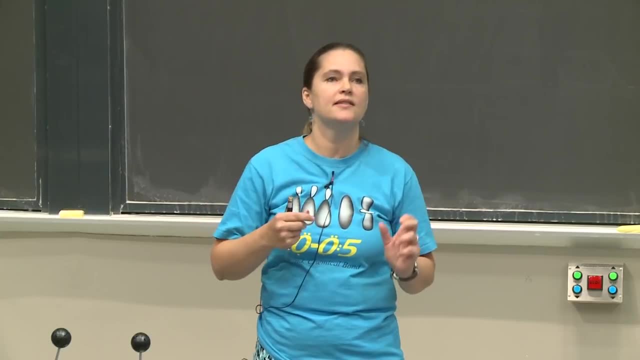 that does not allow for rotation around the double bond. So if you're an organic chemist wanting to make a molecule, that's going to be rigid. if you put a lot of double bonds in it it can't twist and turn very well. 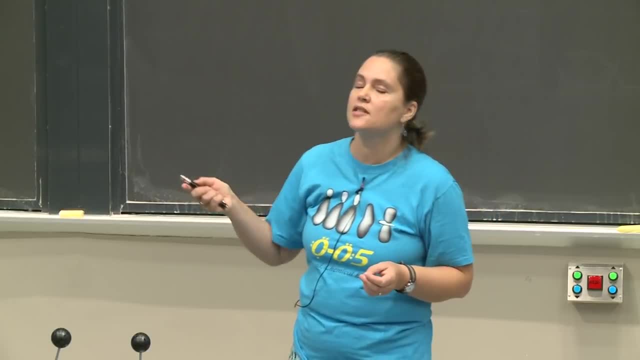 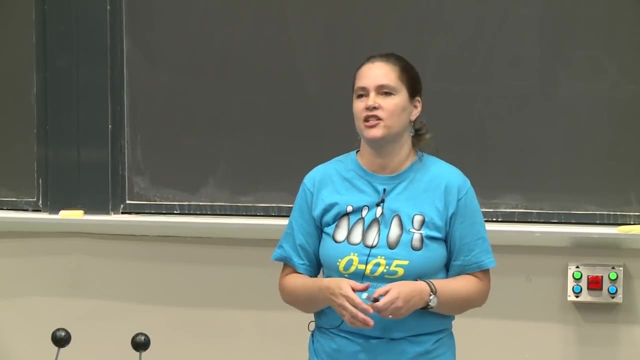 It's often very rigid, which is useful. OK, so we'll stop here And we'll finish up on Friday. sp2 hybridization. For the clicker question, the bond over there on that is also the same as the one on the board. 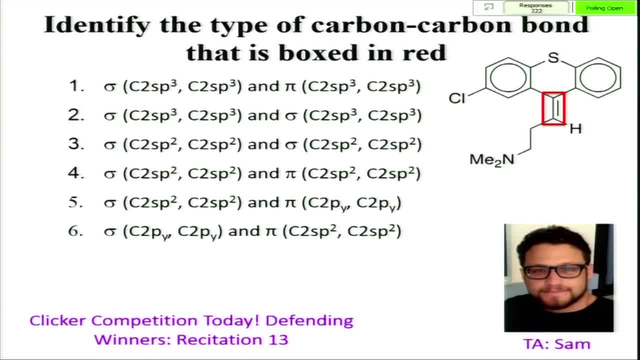 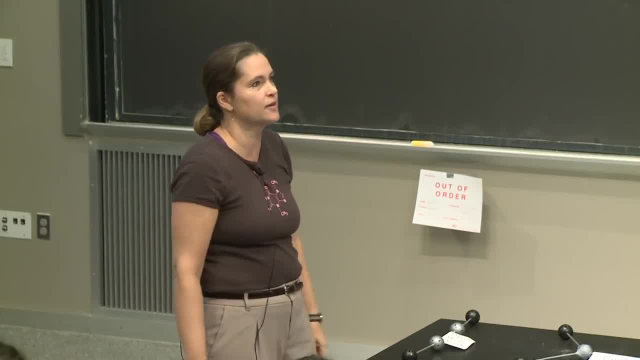 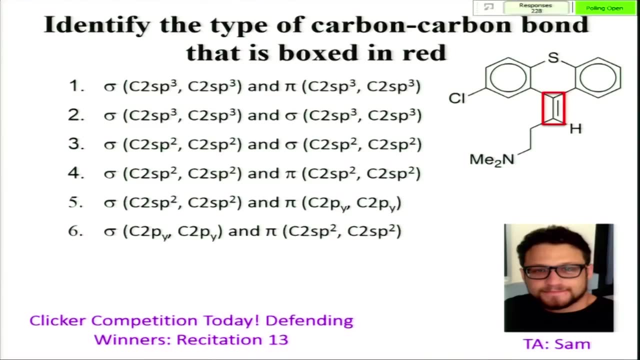 But the one on the board is written with atoms in it And it has squiggly lines to abbreviate. So make sure that your answer is consistent with the picture on the board as well. All right, let's just take 10 more seconds. 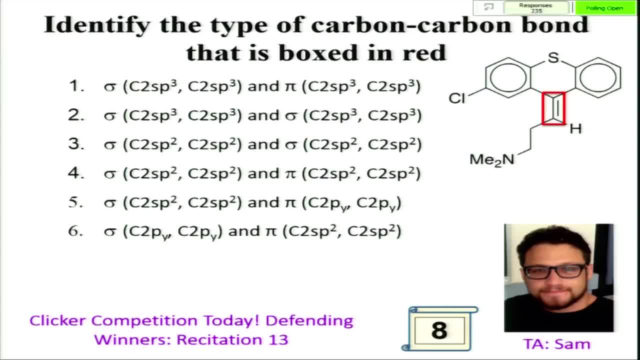 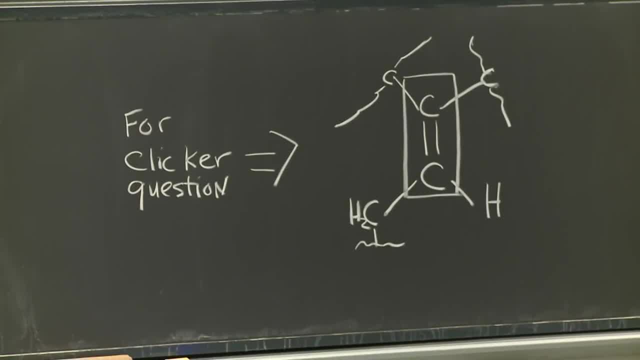 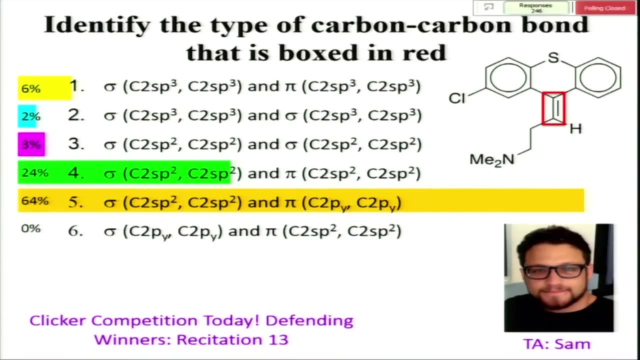 Remember, this is a clicker competition, So we want to get the right answer in for your recitation. All right, It's pretty good because that's the right answer, OK, so let's just take a look at this for a minute. 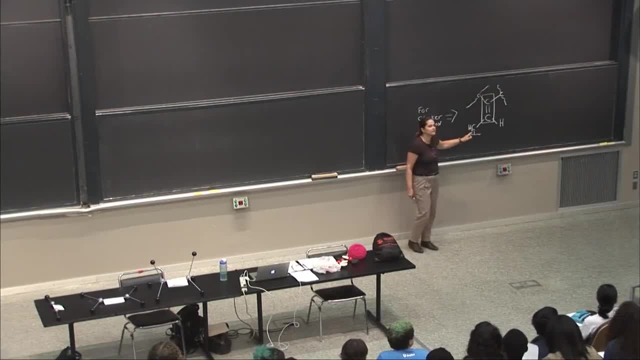 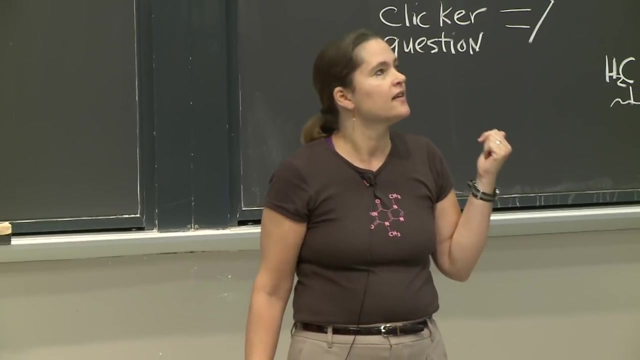 First let me explain. Let's settle down, quiet down. Let me just explain the diagram too, because you'll be seeing these diagrams. So when you just have a bond, a line, and there's no atom indicated, that means it's carbon. 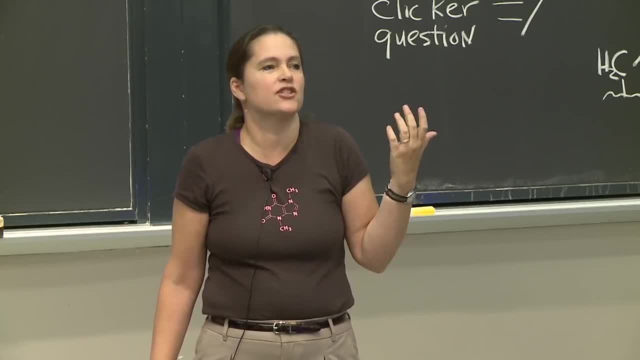 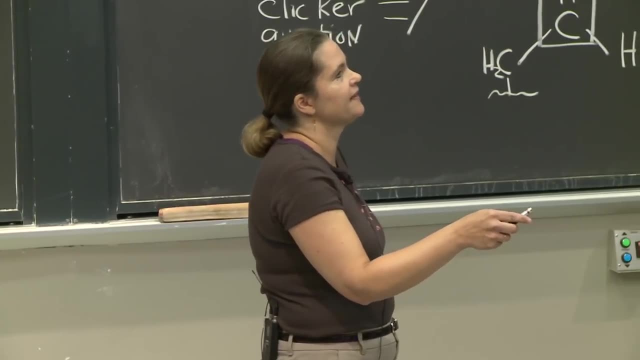 Organic chemists, I think, came up with this rule: Carbon. they just said: if nothing's indicated, of course it's carbon. Carbon is such an important element we don't really need to say more about it than that. So you could interpret this diagram. 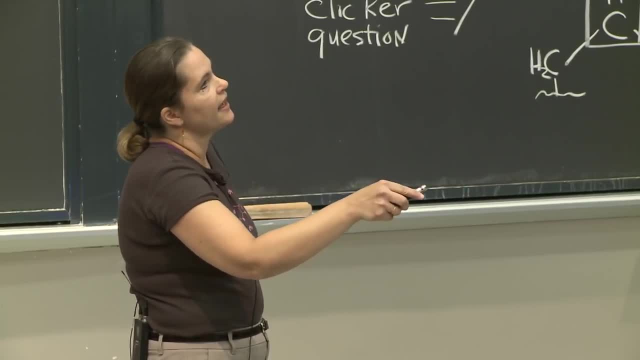 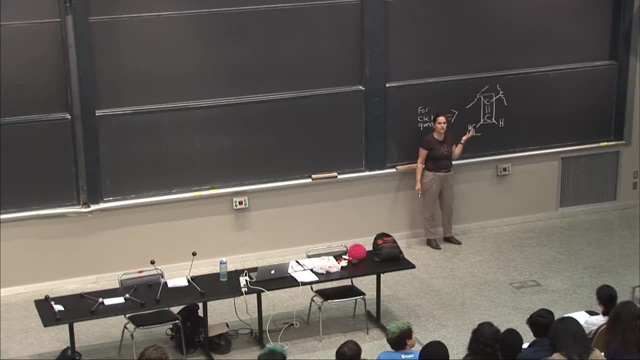 You have a carbon double bonded to another carbon And then up here there's a carbon in that ring. So I just put in this diagram carbon with squigglies. You'll see that sometimes That means that there's more atoms there. 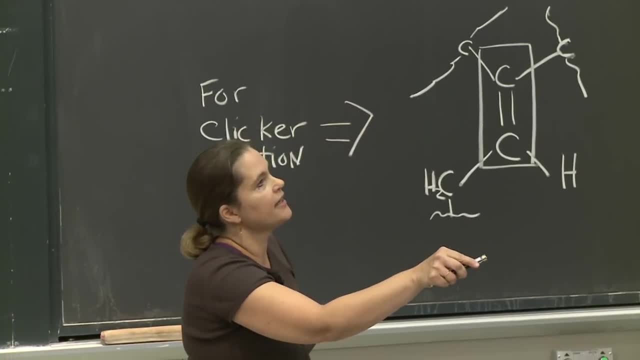 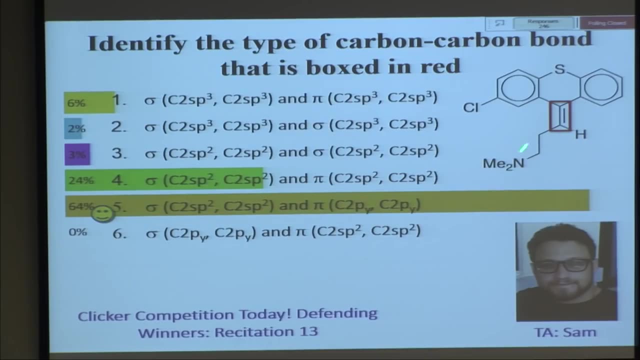 but I'm too lazy to draw them. And on this side There's a carbon, but there's more atoms there and I'm too lazy to draw another squiggly. Then we have the double bond. So there's a carbon down here as well. 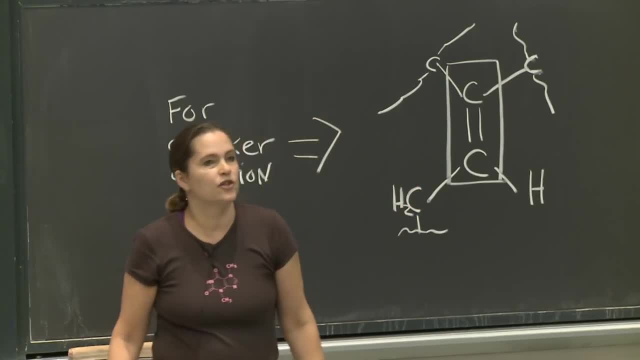 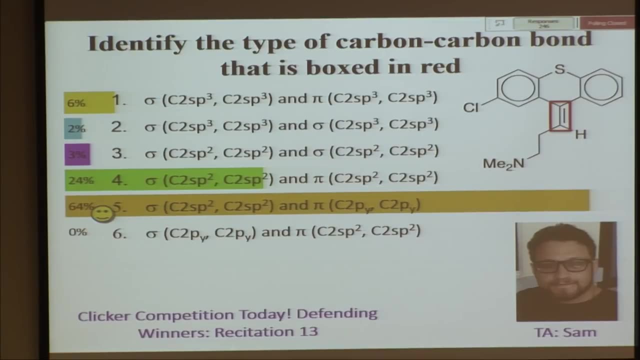 It wasn't indicated. It's just the line in the drawing And you have to predict how many hydrogens. Hydrogens are often not indicated. This one is indicated. There are other hydrogens in this drawing that are not indicated. You need to figure out where they go. 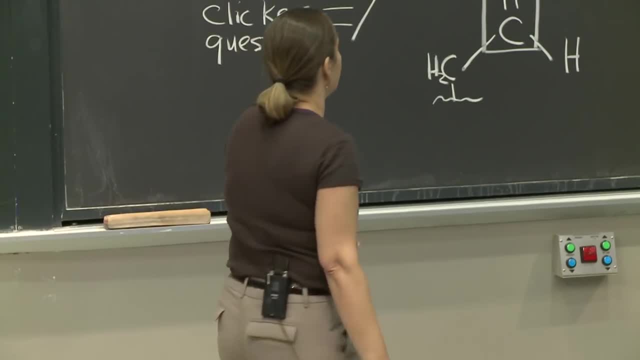 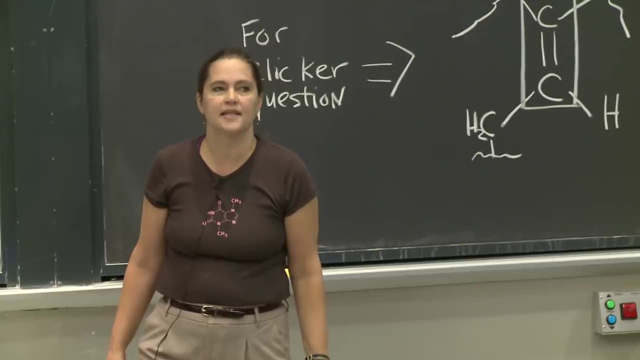 And the material we're doing now is going to help you do that. And then I also drew something in another squiggly, because I was too lazy to draw the rest. So these are different kinds of diagrams that you'll see, that all mean there's more than one way. 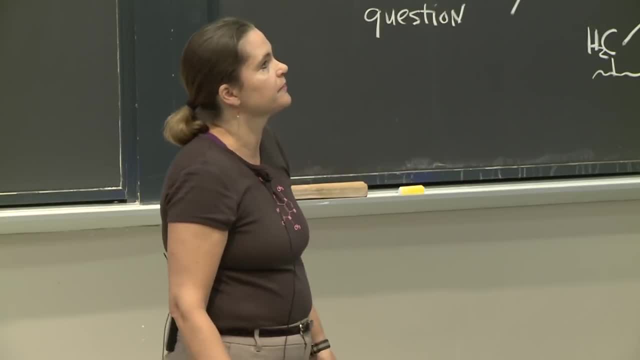 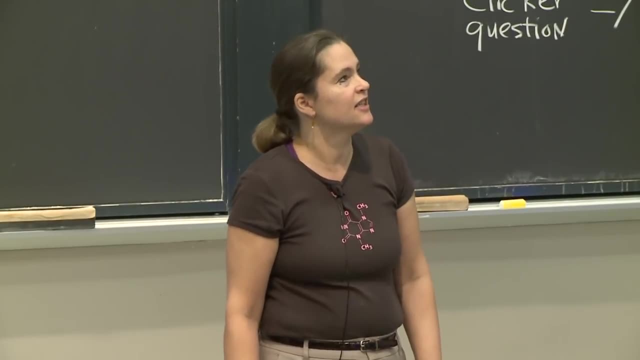 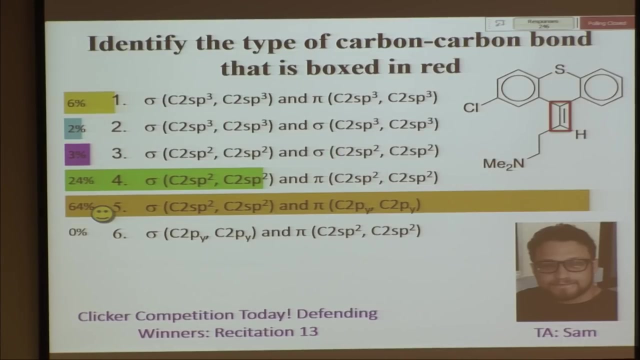 to write the same structure. So this particular molecule was used to treat schizophrenia in the 1950s And key to the usefulness of the molecule was that double bond, As we talked about last time. double bonds restrict movement. You can't talk. 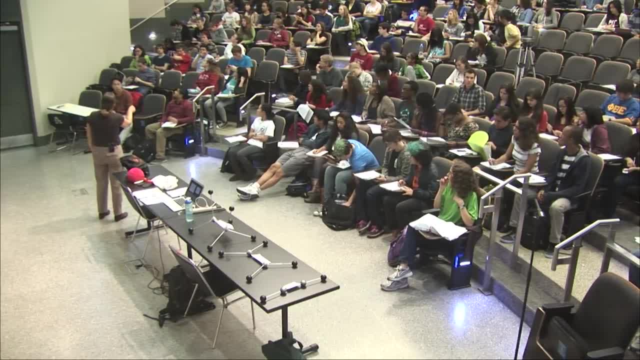 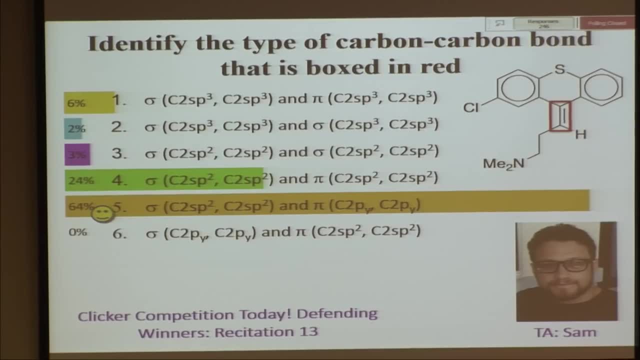 You can't twist around the double bond And so if you had exchange and you had this group over there and the hydrogen over here, it wouldn't be an active molecule. So this double bond fixes the orientation of those other atoms such that it was an active molecule. 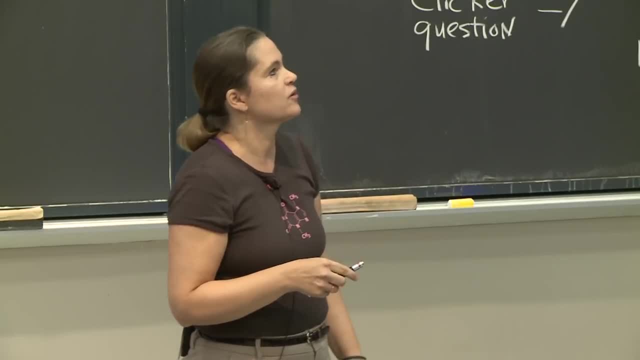 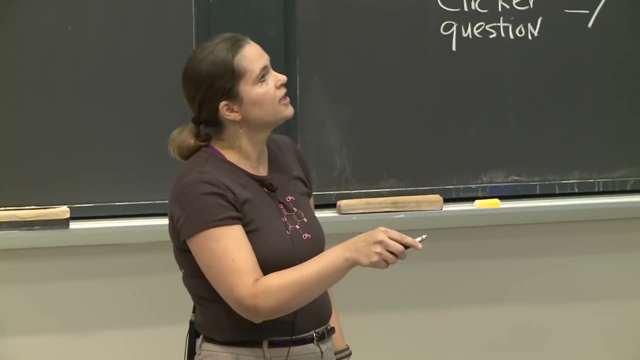 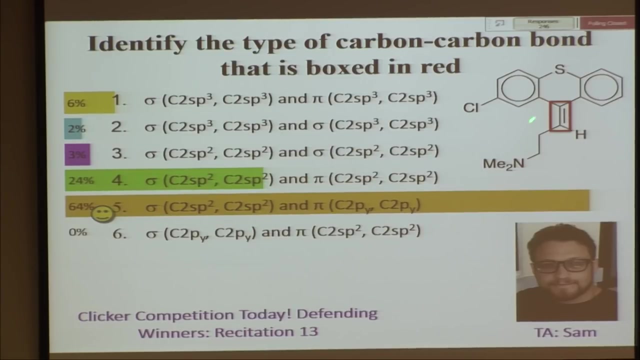 and could be used as a pharmaceutical to treat schizophrenia. So, in terms of the bonds, then we have a double bond, which means we have one sigma and one pi bond, And so the sigma bond down here. we had to know, We had to know what the hybridization was. 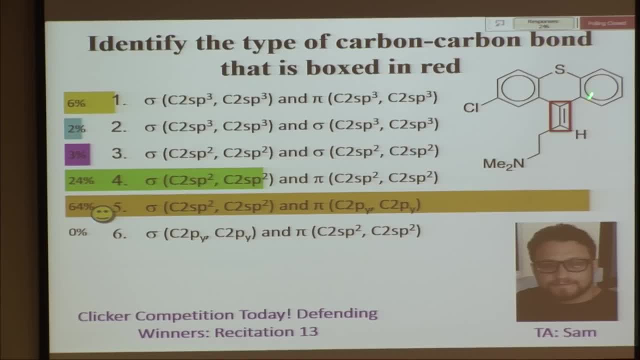 And here those carbons are bonded to three other atoms, And so it would be sp2 carbons, And also with a double bond, sp2.. And then we also have a pi bond, And pi bonds are made up of non-hybridized orbitals. 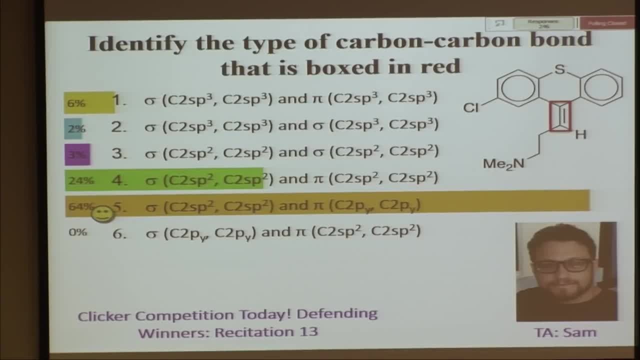 rpy or rpx, And so those are the ones that make up the pi bond. And then we have some variations, Some you had two sigmas. That's not right. We have a sigma and a pi, So most people figured that out. 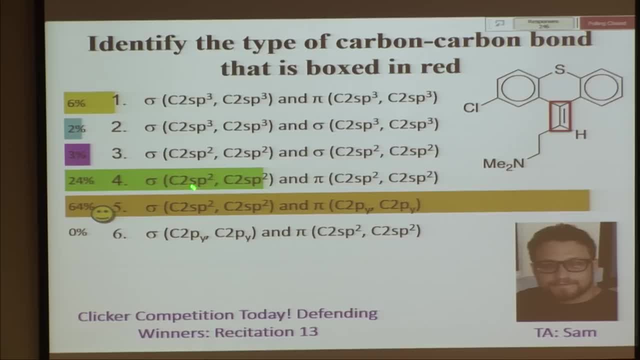 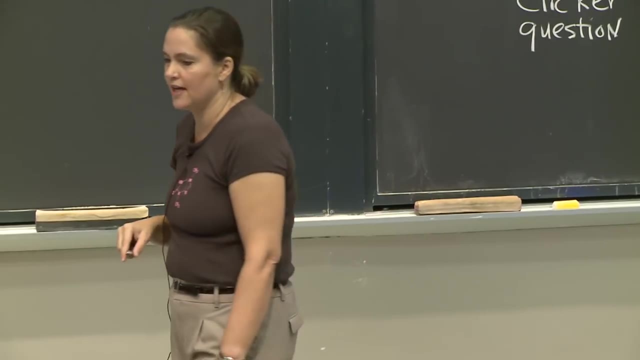 They picked the ones that had those categories for the most part, And then you had to pay attention to whether it was sp2 or sp3. And then here this one is. the pi bond is not made up of hybridized orbitals. It's made up of the atomic orbital left over. 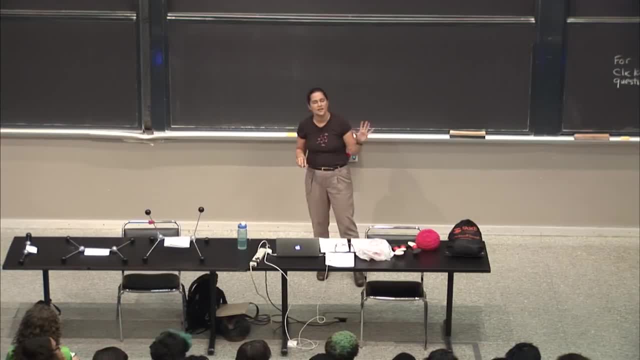 So a lot to look at that particular problem, But this is really good practice For the exam which is coming up a week from Monday. there's going to be lots of hybridization And today we're going to post extra problems for the exam. 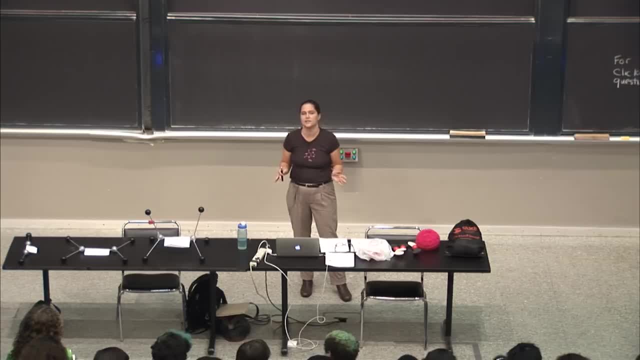 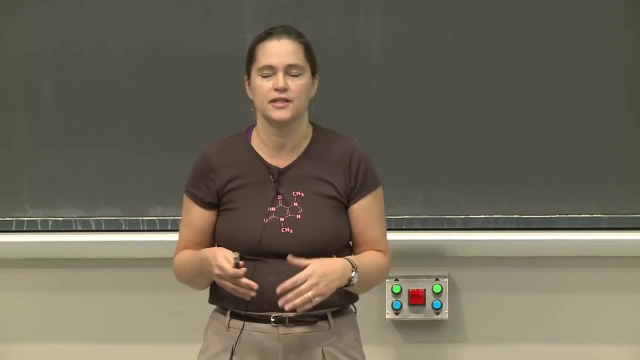 So you have really a whole week to start getting ready for this exam and to keep up with the new material, And so extra problems in an old exam are also going to be posted later today. All right, so let's just finish with hybridization now. 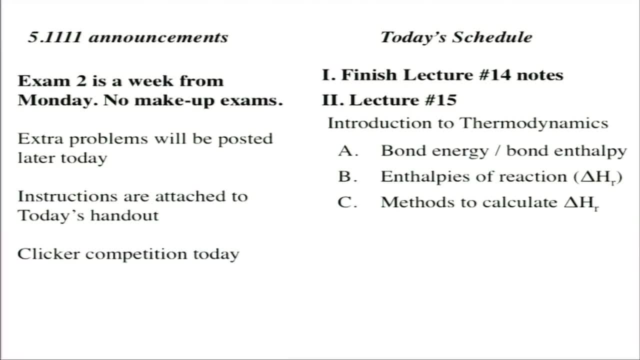 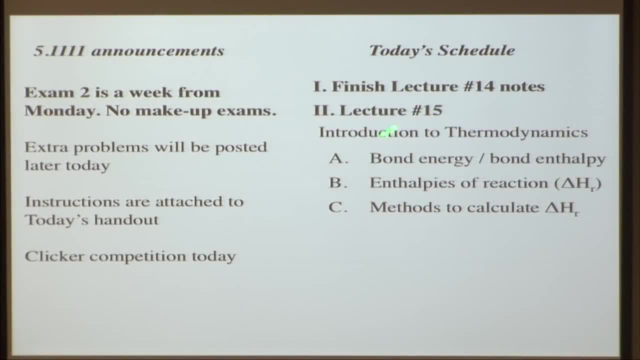 And this is good, because this is all stuff that's going to be on the exam, and also the instructions for the exam are attached to today's handouts. And, of course, remember, no makeup exams and clicker competition, So I'm not really going to go through anything. 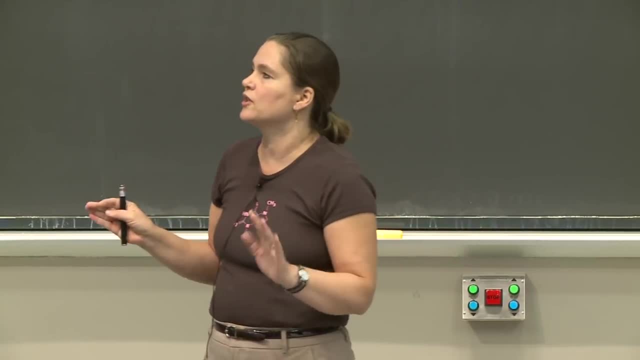 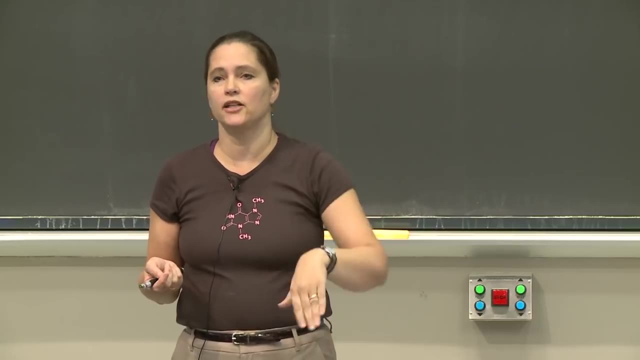 in the instructions. It's very similar to last time, So you can take a look at that and see the material. The material starts with the periodic table, periodic trends, and goes through the material that I'm going to finish with partway through today's lecture. 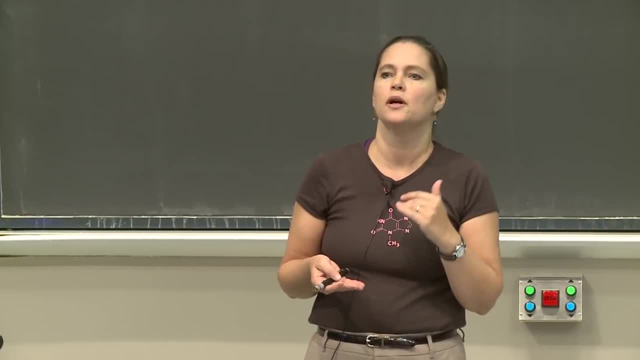 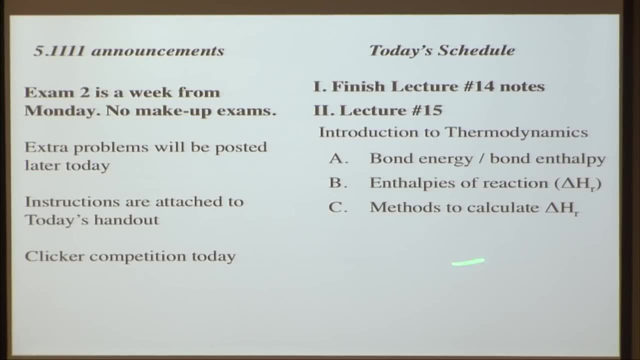 So at the end of hybridization, that's the end of exam two material. So we're going to finish our lecture notes from last time, So pull those out, And then we're going to move on to thermodynamics. So once we hit thermodynamics, that's exam three material. 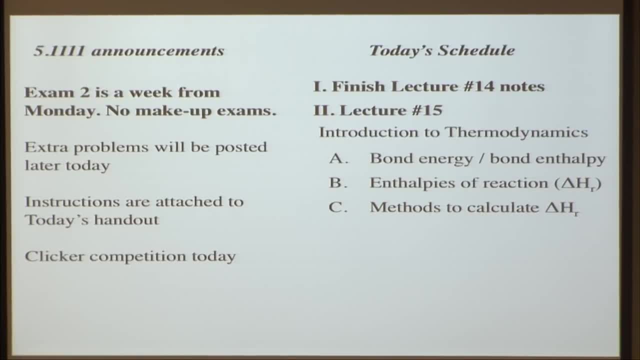 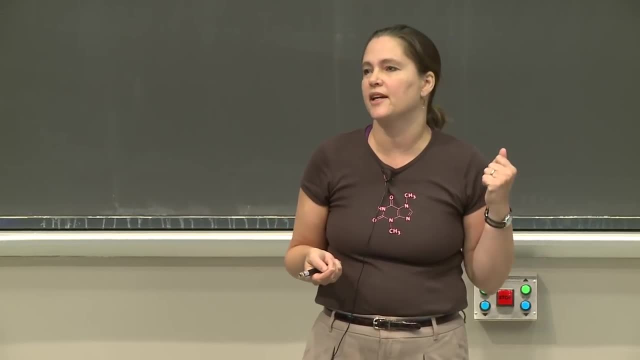 So we're almost done with exam two material A week in advance to get ready for the exam. so that's great Lots of time to review exam two material And let's see if we can have an A average on this exam. That would make me really, really, really happy. 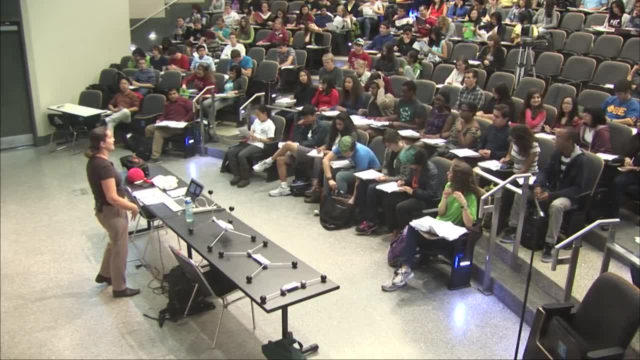 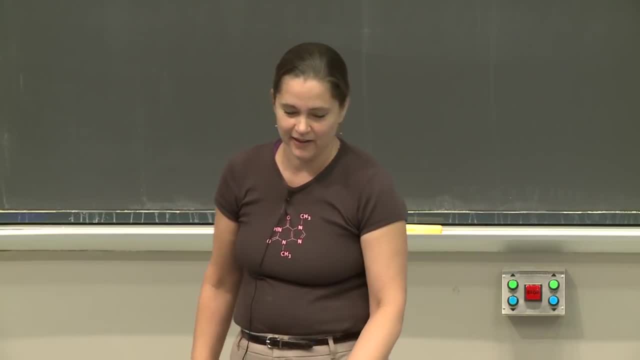 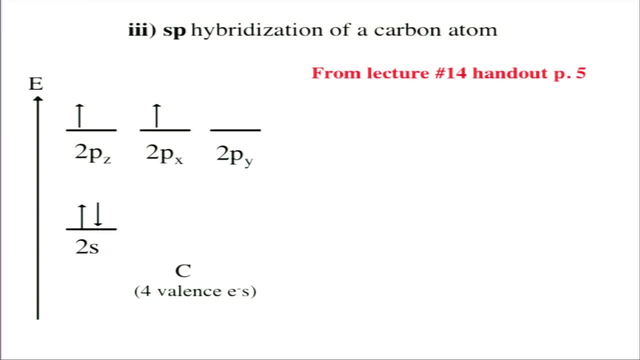 I would wear my periodic table. I would wear my periodic table leggings again, if we could get an A average on the exam. I'm just saying I'd be very excited. OK, so we better finish up that material so that you can get started. get ready for this. 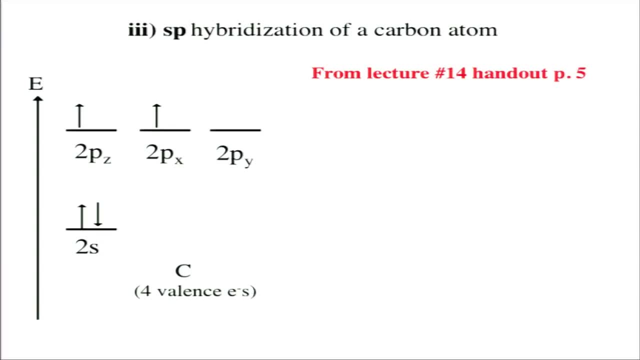 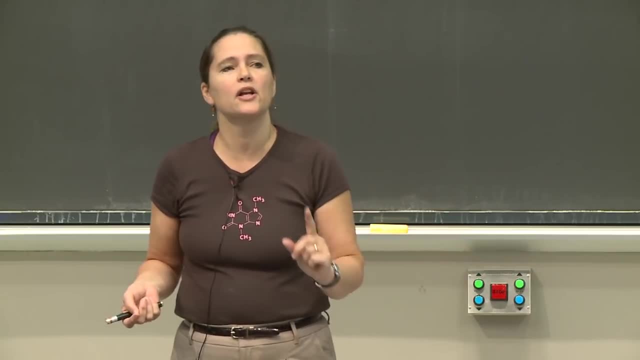 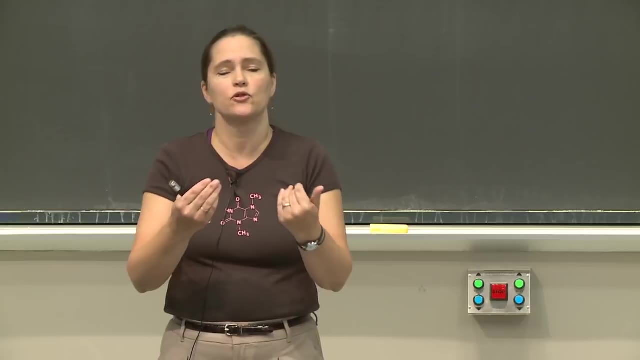 So we're talking about valence bond theory and hybridization and forming these hybrid orbitals. And valence bond theory is this idea that when you have a single electron in an orbital you can form a bond, and bonding happens when two atoms spring together- single electrons. 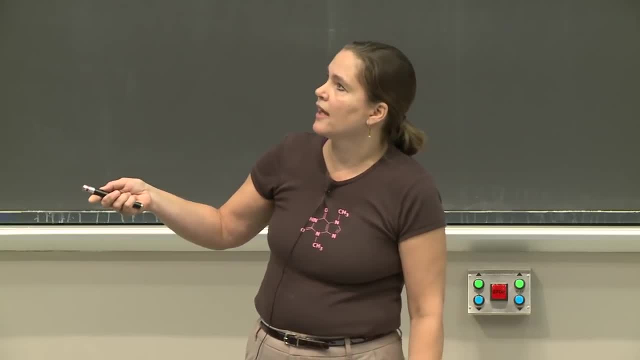 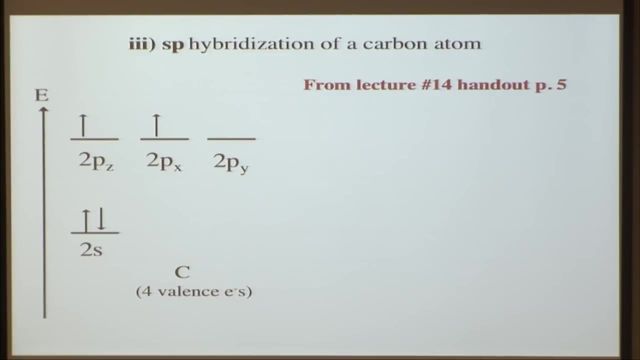 and those pair up to form a bond. So we talked about electron promotion before, And let's just review what that meant. So if you have an empty orbital, you can promote one of your electrons to that empty orbital, And so now we have four valence electrons. 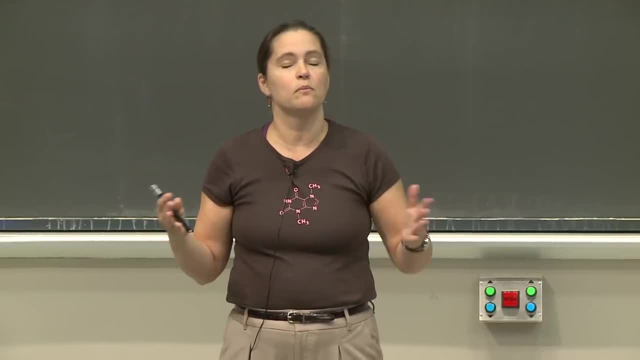 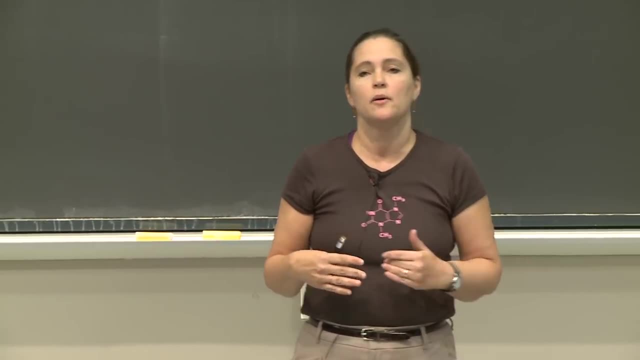 after electron promotion, so that we have the more possibility of forming bonds. Now, if you don't have an empty orbital, you can't promote your electron. If you do have an empty orbital, you can promote it. more single electrons available for bonding. 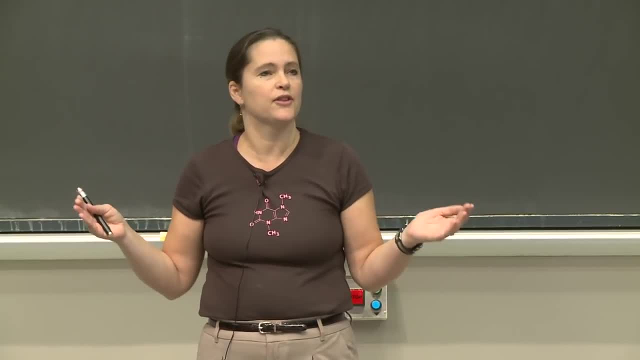 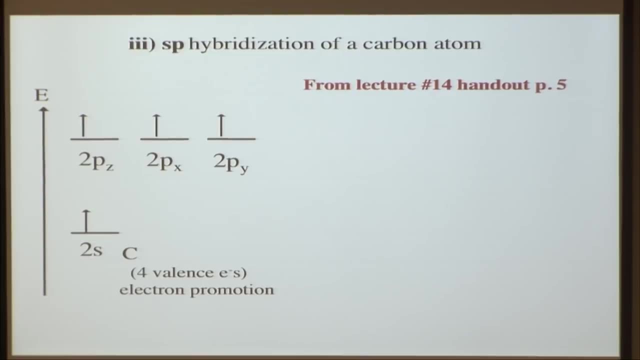 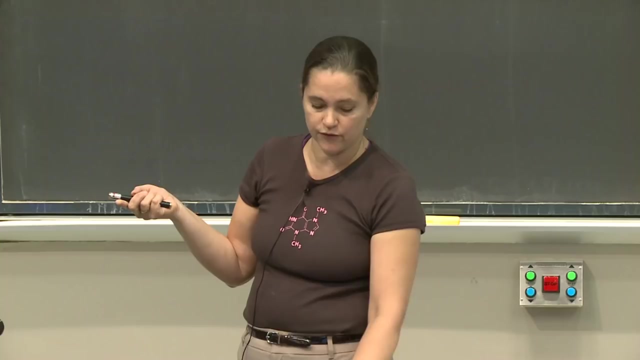 If you don't have an empty orbital, there's nothing to do with that. So that's the trick to electron promotion. All right, so now we have one electron in each of the four valence atomic orbitals that we have for carbon. 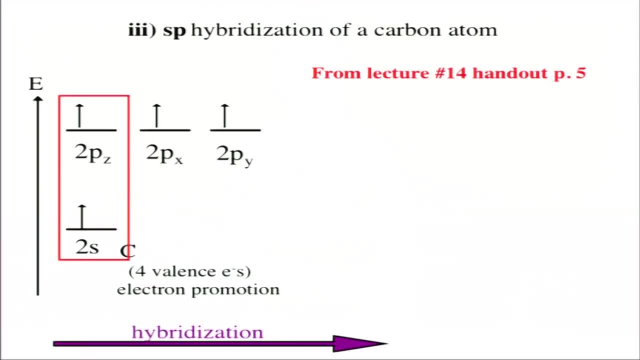 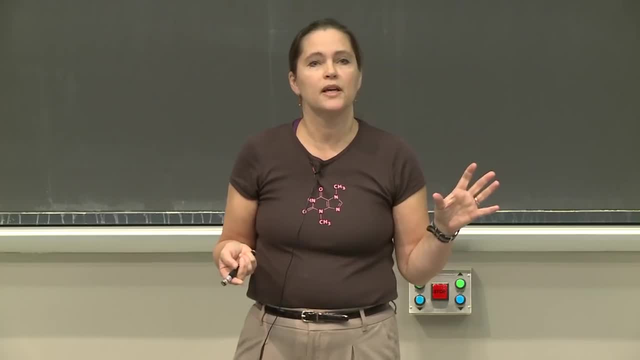 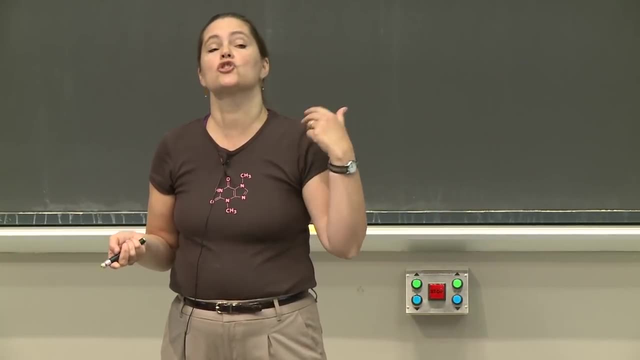 But we're going to only hybridize two of them. We saw already last time that we can hybridize all four orbitals and have sp3.. We can hybridize just three of those orbitals and have sp2.. Now we're going to see that we can hybridize just two. 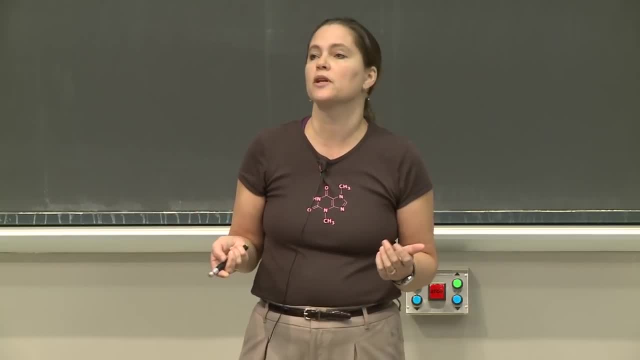 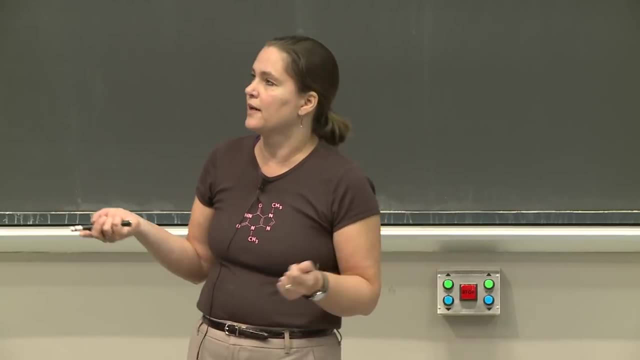 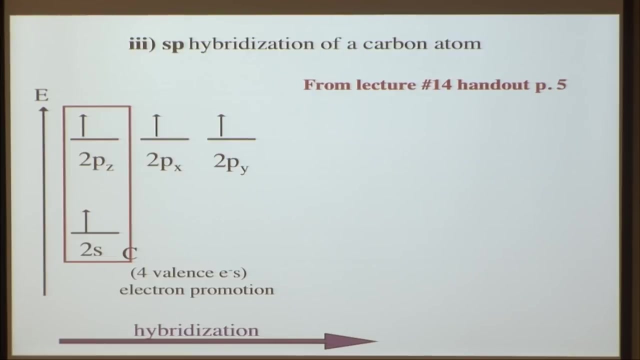 of those orbitals and have sp. So carbon is really amazing. It can do all three of these kinds of hybridization. That's why carbon-based life forms are able to exist and do so much. So we're going to now hybridize our 2s and our 2pz. 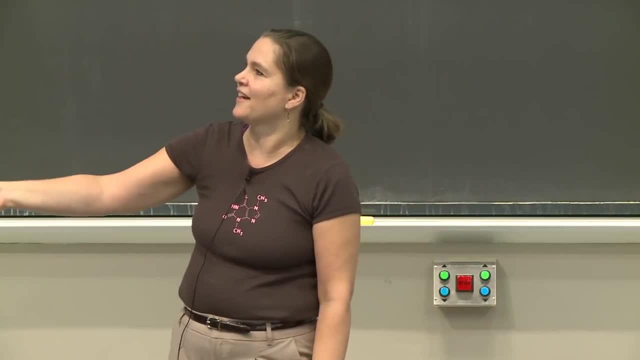 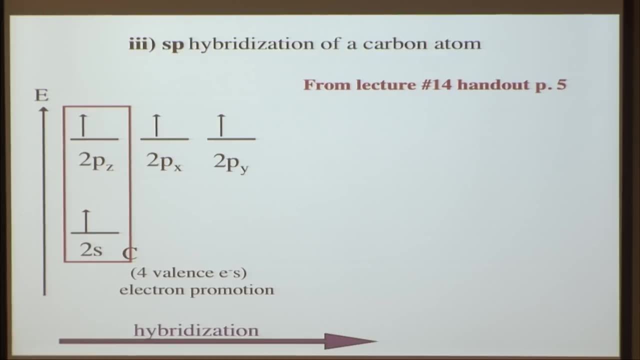 z is just special, And so it gets to hybridize with the 2s, leaving two of the other orbitals just by themselves. So we're going to form two hybrid orbitals Again if we hybridize two atomic orbitals. 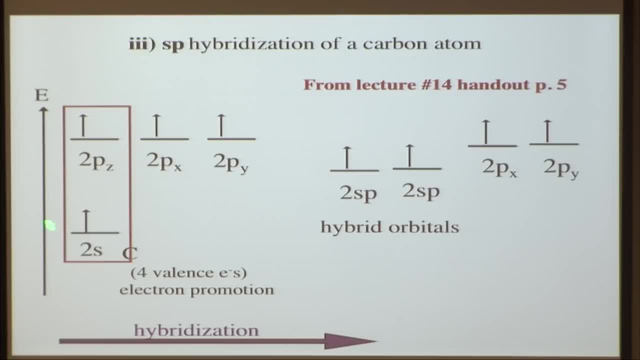 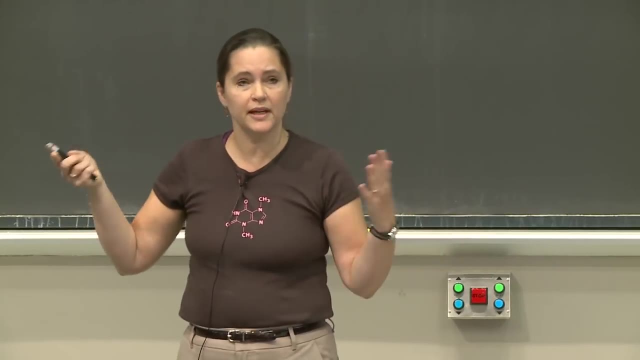 we're going to form two hybrid orbitals And if we hybridize 2s and 2pz, we're going to get 2pz And we're going to get hybrid 2sp orbitals And we'll have our 2px and our 2py, just the same as always. 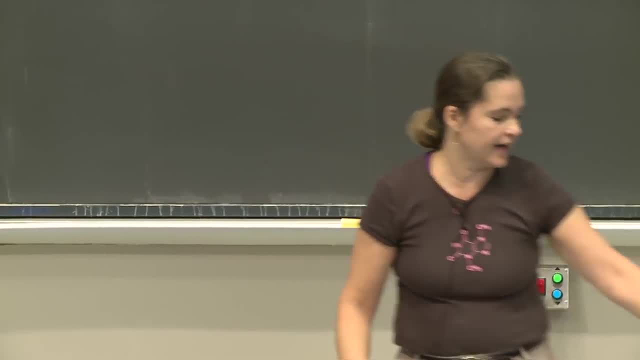 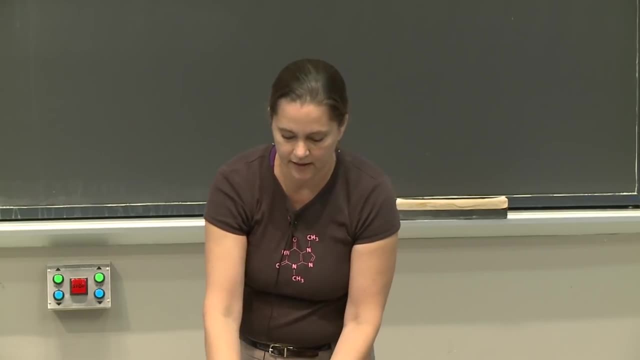 All right, so we can think about this in terms of shapes as well. So we have again our spherically symmetric s orbitals and our p orbitals, And we have the three of our p orbitals. that are the same shape, they're just different orientation. 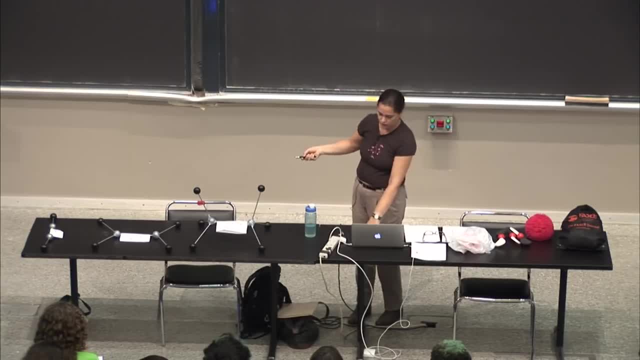 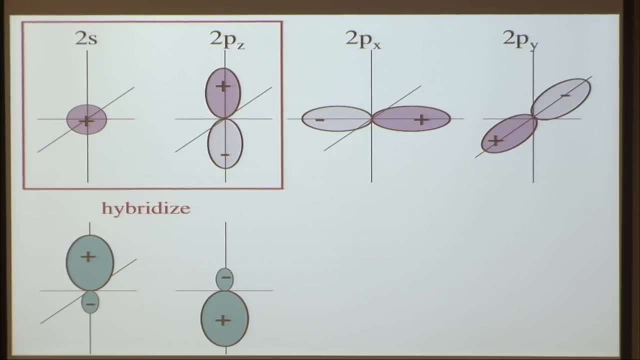 in space. So we're going to hybridize our 2pz and our 2s And so we'll have our kind of funny looking- I think of them as turtle shaped hybrid orbitals. And then we also have our 2px and 2py orbitals. 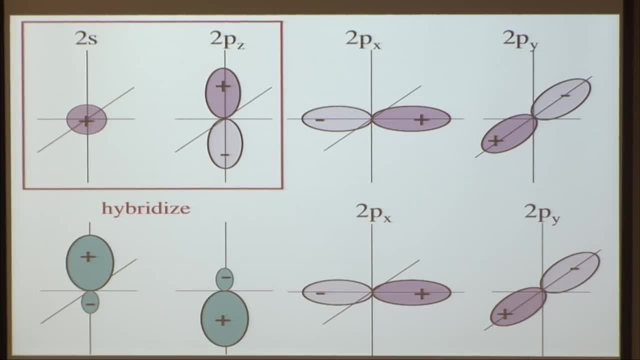 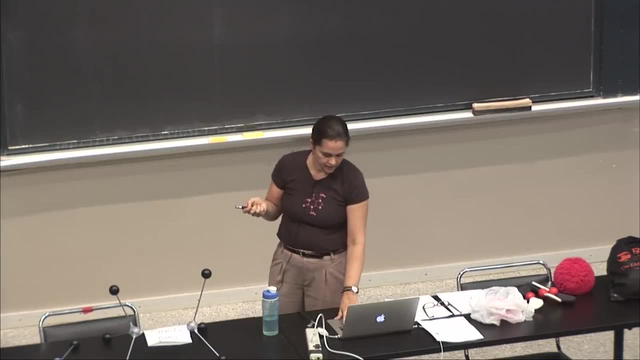 the same as always. So what are we going to do with our 2sp orbitals and our 1 2px and 1 2py? Well, we can form a pretty cool molecule with it, So we're going to. 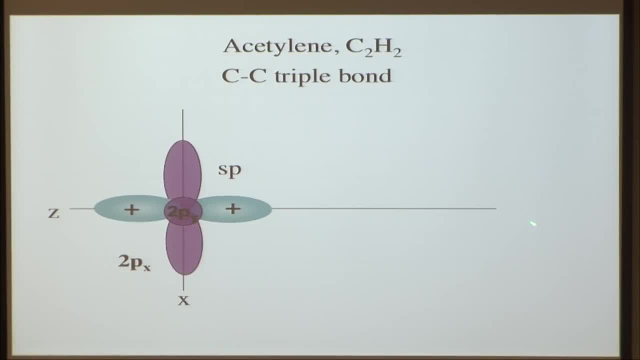 Form, something that has a carbon-carbon triple bond, So this is C2H2.. So now in cyan is the sp orbital, the hybrid orbital that is formed on this carbon here, And then we have a 2px orbital here in the plane of the screen. 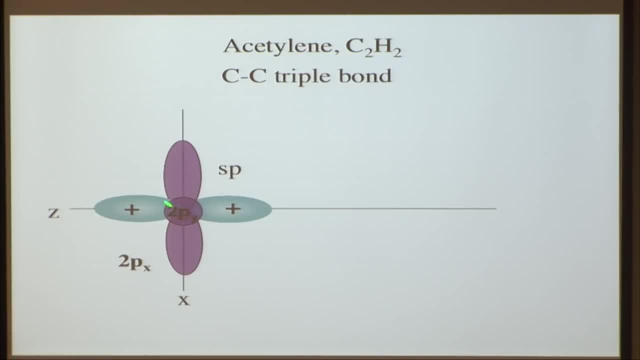 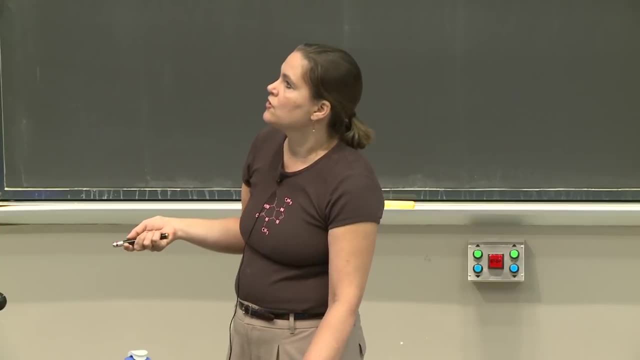 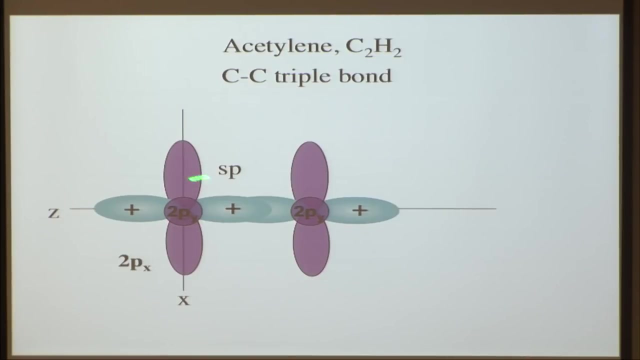 And we have a 2py orbital coming out toward us And of course, our 2pz orbital had been hybridized with the 2s. So here we have this structure, We're going to bring in our other carbon, And the other carbon has the same situation going on. 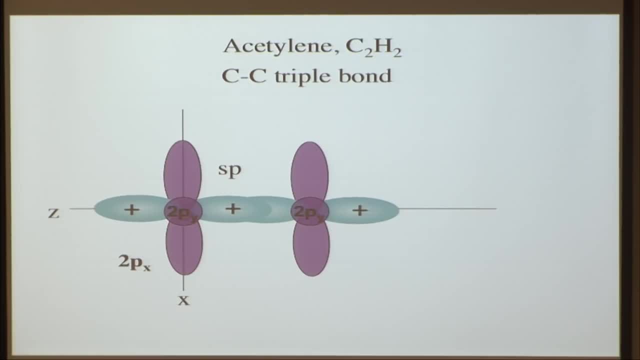 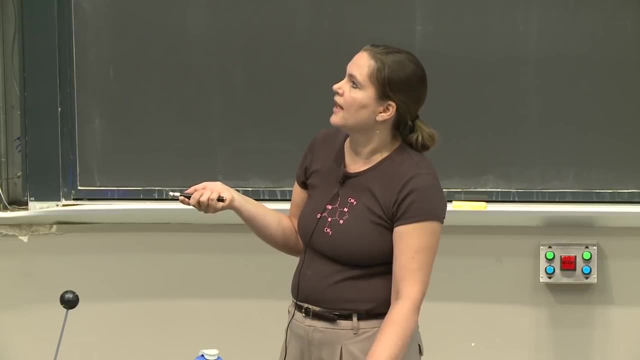 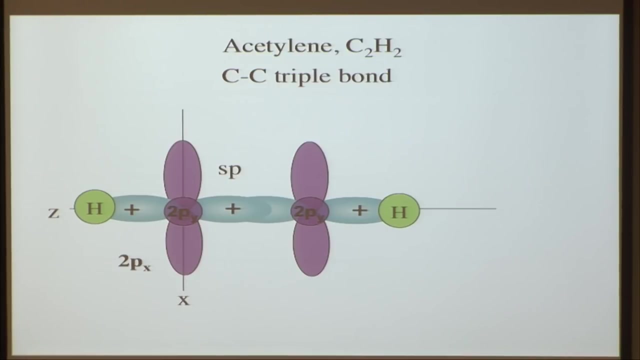 And we can form a bond between the two carbons with our sp orbitals And we can form also with the sp hybrid orbitals bonds to hydrogen. So we have two hydrogens, one over here and one over there. So what is the angle between these hydrogens here? 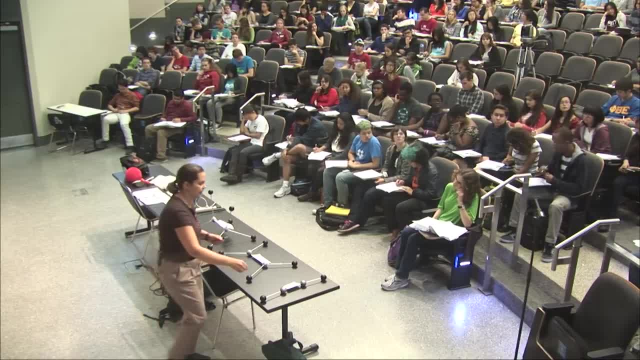 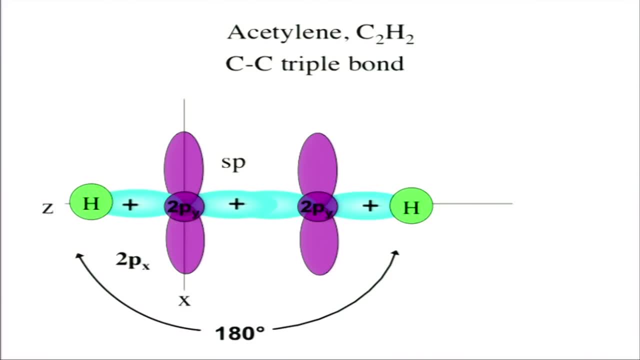 Yeah, so that's 180.. And again, we have an example here of the molecule we're going to build that's going to have a triple bond. So now let's name those. OK, Let's name those types of bonds. or, as sometimes in a problem, 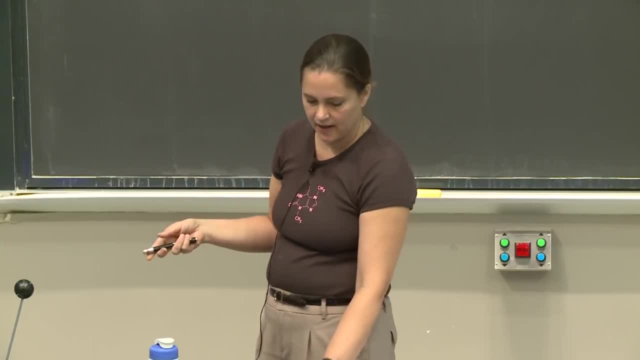 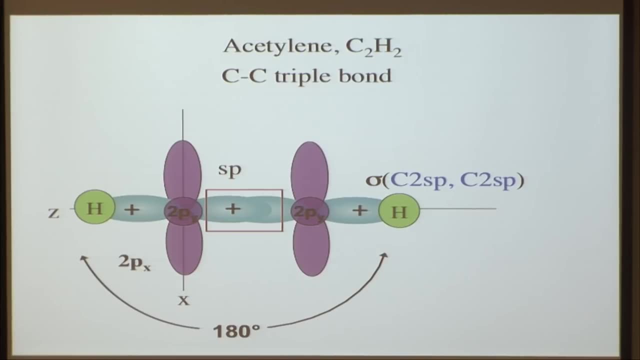 set. it will say: describe the symmetry of the bond. And what it means by that is the following: It means that that's either say name the type of bond or describe the symmetry. There's multiple ways to ask the question. 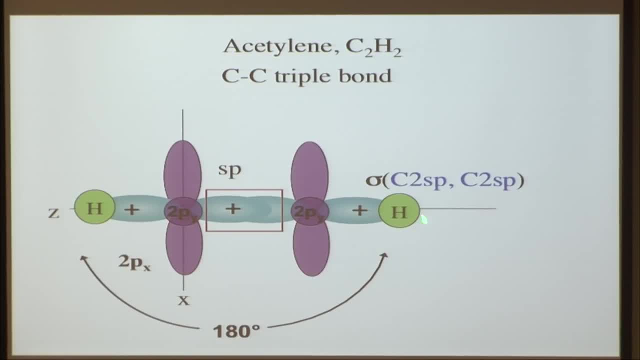 And this is the answer to those questions. So the bond that's formed, the first one that's formed between the two carbons- is a sigma bond And it's formed between the sp orbitals. So we have a sigma bond, a carbon 2sp, a carbon 2sp. 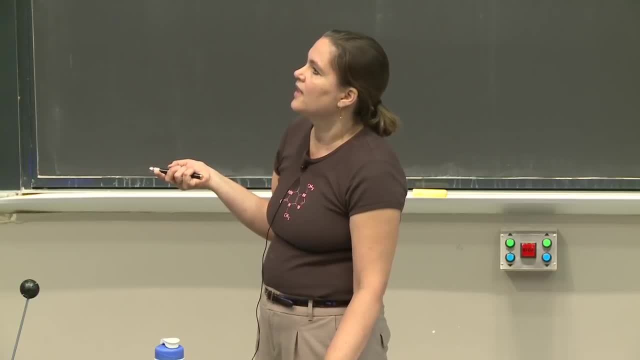 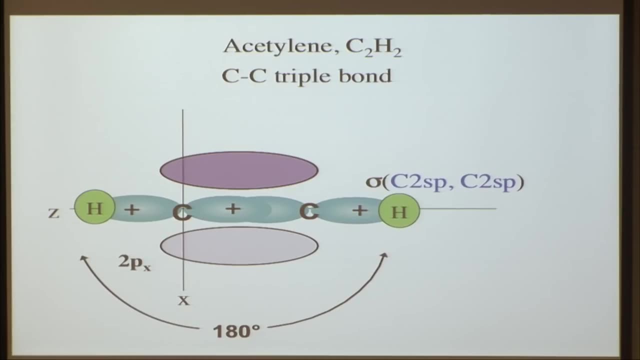 That's the first one, But this is a triple bond. So we have two more bonds to form, And this is where our atomic px and py orbitals will come in. So we're going to form the next bond, which is what. 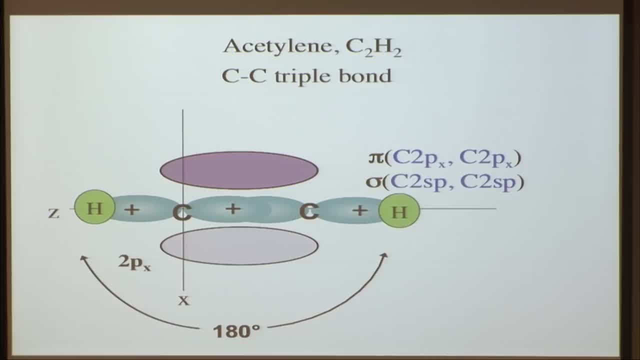 A sigma or pi Pi bond, And that can be between our xpx orbitals. So pi carbon 2px, carbon 2px, And now we have the 2py orbitals as well, And that allows us to form our triple bond. So we're also going to have a bond: pi c2py, comma c2py. So, again with a triple bond, we're going to have one sigma and two pi bonds. The sigma is formed from the hybrid orbitals And the pi bonds are going to form. 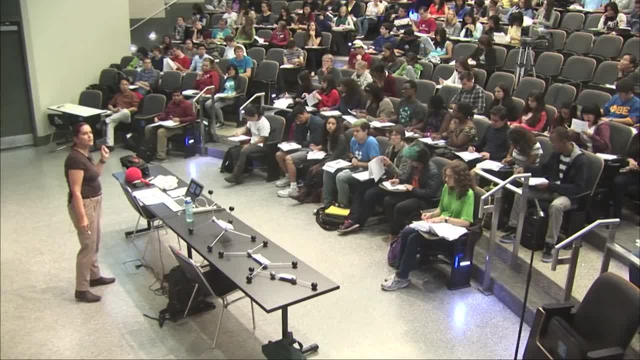 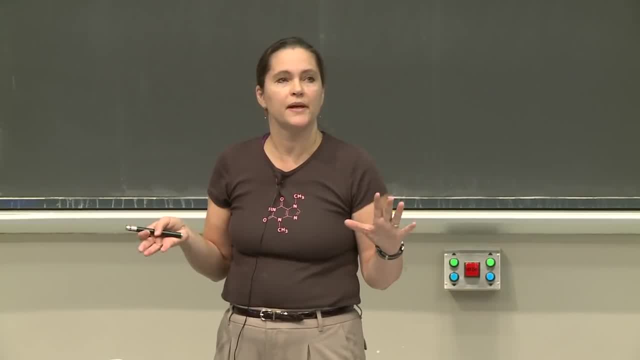 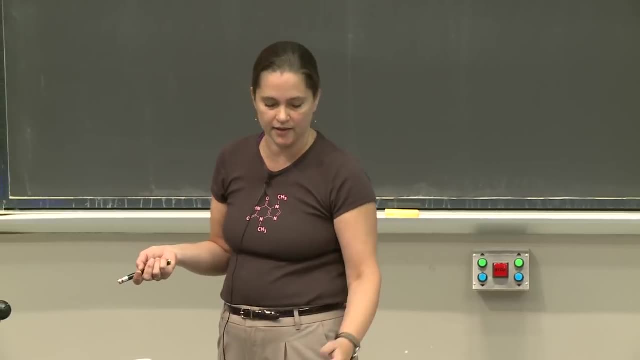 by the two px and 2py orbitals. So carbon really impressive. Carbon can form all of these three types of hybrid orbitals. It can form molecules with single bonds, double bonds and triple bonds. So let's just have a little cheat sheet to think about that. 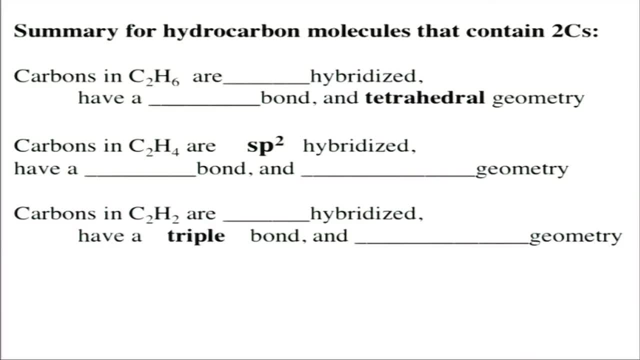 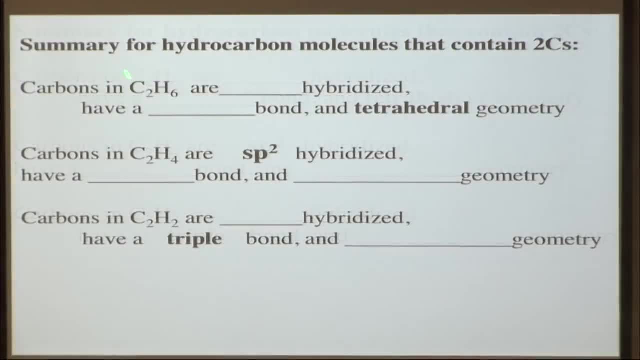 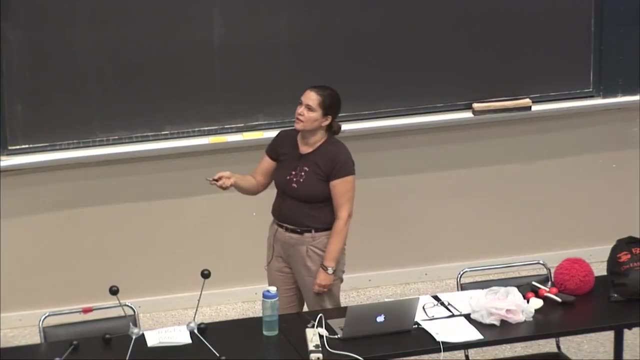 So again, this is for hydrocarbon molecules, like we've looked at so far, that have two carbons in them. So let's look at carbon in C2H6.. So that's over here What is going to be the hybridization. 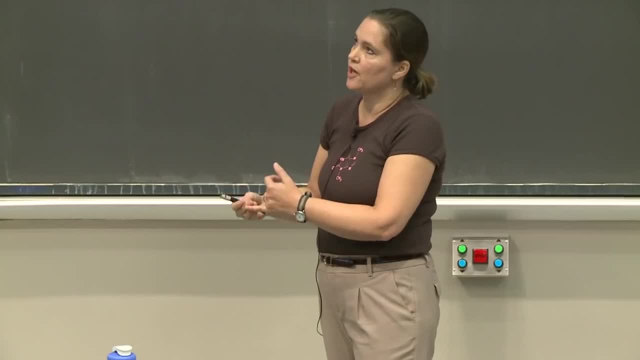 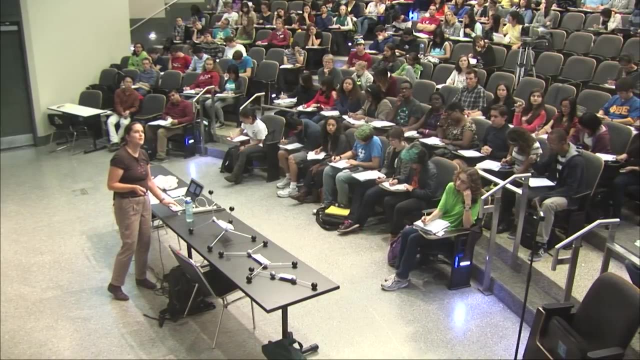 when you have a carbon that has a bond to another carbon and a bond to three hydrogens. here, What hybridization? sp3, that's right, And it's going to have what kind of a bond? Single, double or triple? 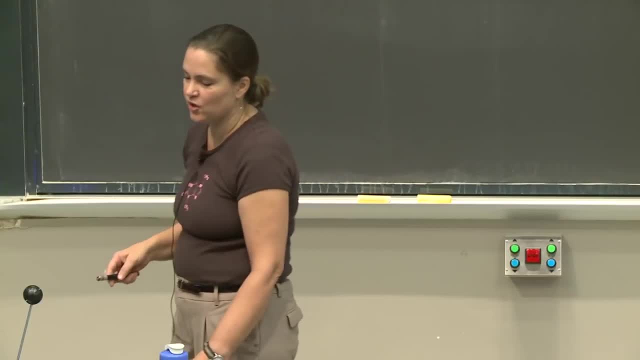 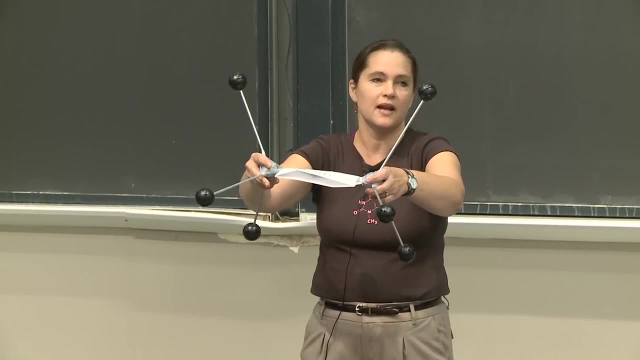 It's going to have a single bond And it's going to have tetrahedral geomagnetic geometry around both of the carbons. So both of these carbons are going to have tetrahedral geometry, which is not a blank in your note, but what's the angle? 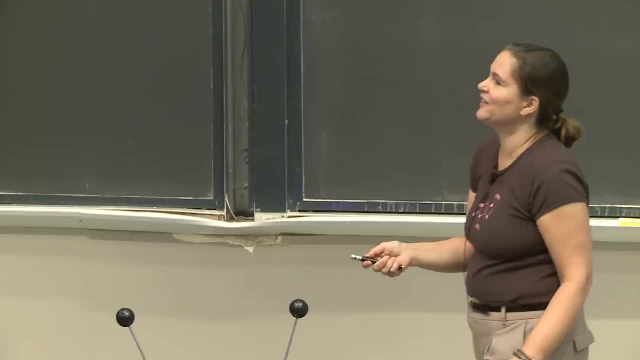 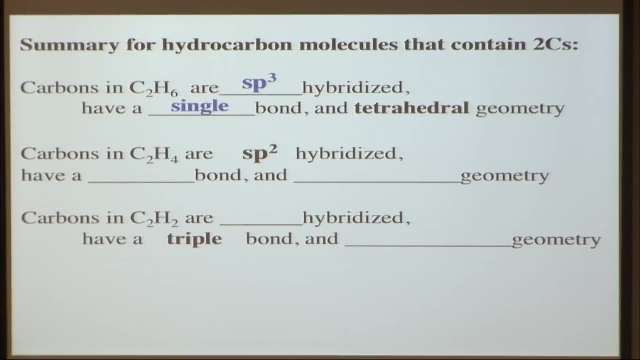 109.5, right, Thank you. So we have carbons C2H2 are going to be sp2 hybridized, And what kind of a bond are they going to have between the two carbons? That'll be a double bond. 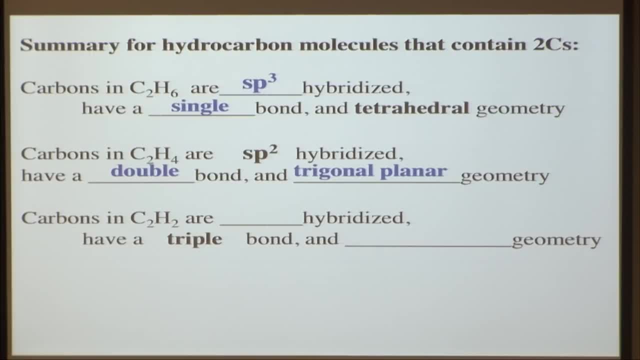 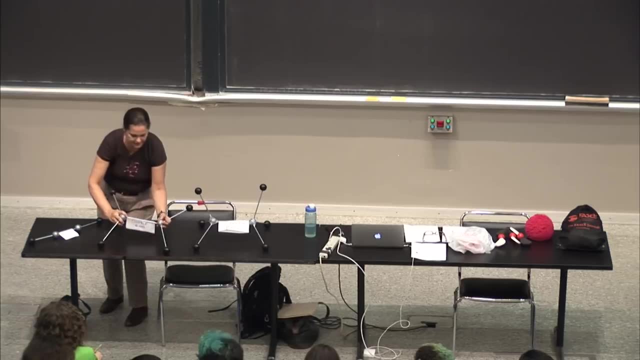 And what is the geometry of that Trigonal planar, Right trigonal planar? And here you have to pretend this is a double bond. My model kit didn't come with double bond possibilities And I have to hold it very carefully. 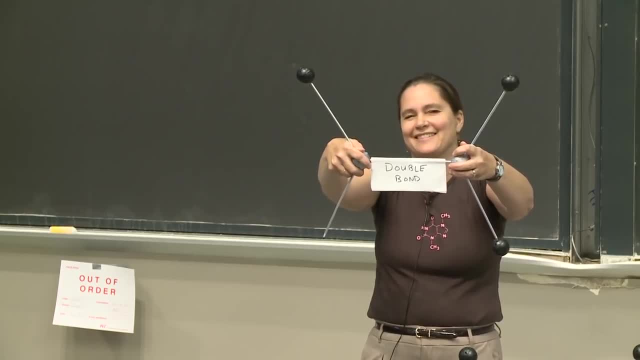 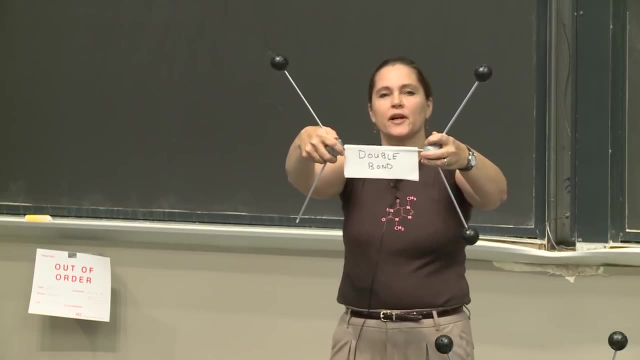 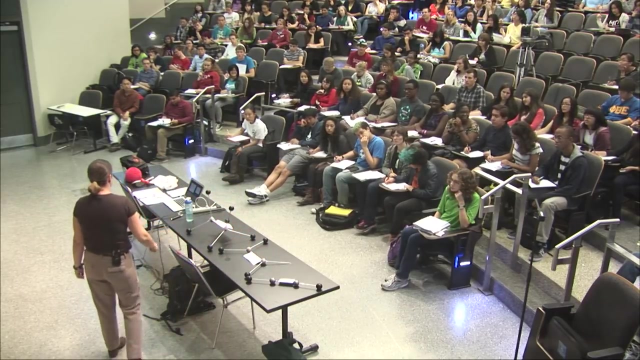 But if I hold it very carefully, the bonds are still there. You'll see that the angles are 120. And so this is trigonal planar geometry at each carbon. We didn't tape that one. You can see there's scotch tape all over the others. 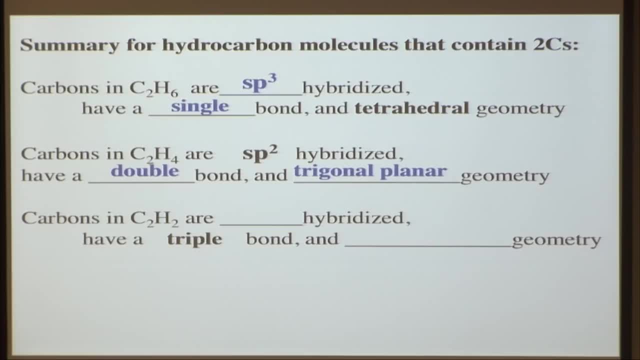 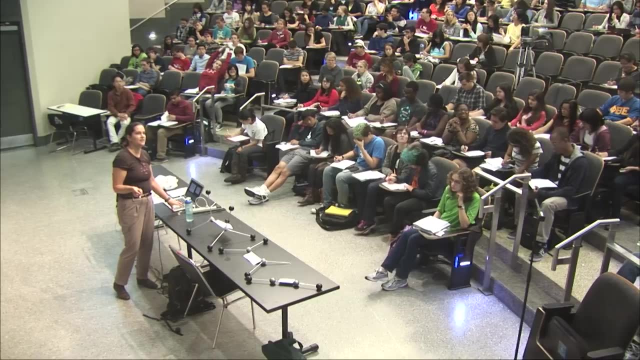 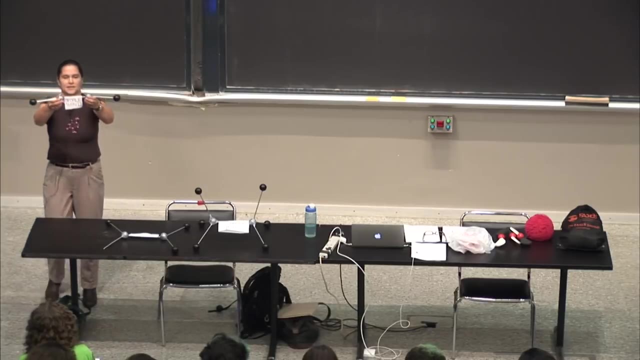 It was not a happy molecule. OK, so now C2H2, what kind of hybridization? Sp. That is our friend, the triple bond, And we're going to have linear geometry and 180.. So both carbons have linear geometry. 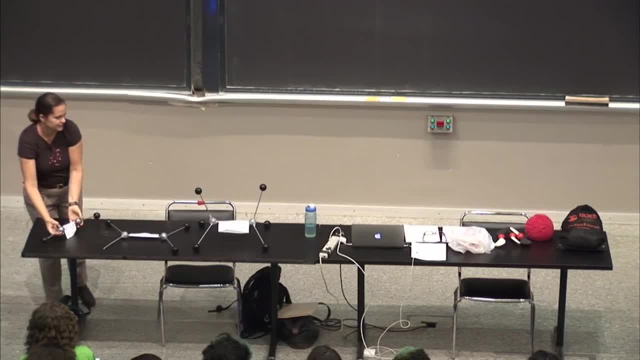 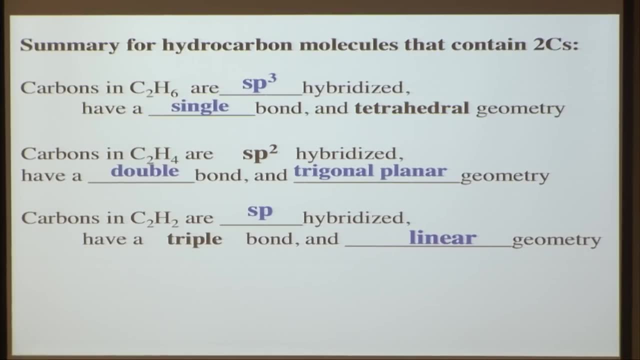 That works. Triple bonds are much more stable. They don't fall apart as much. OK, so that's a cheat sheet for carbon. Now, if you're thinking about nitrogen or oxygen, those often have lone pairs on them. Carbon likes to form all bonds. 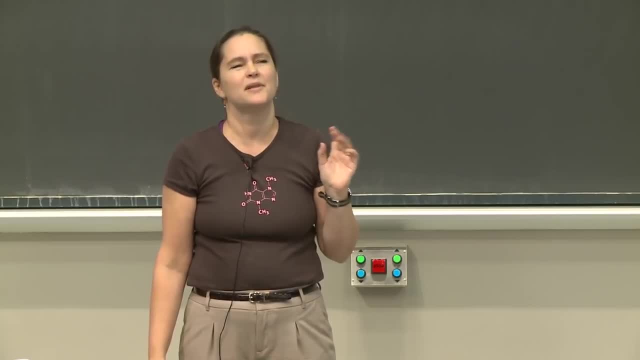 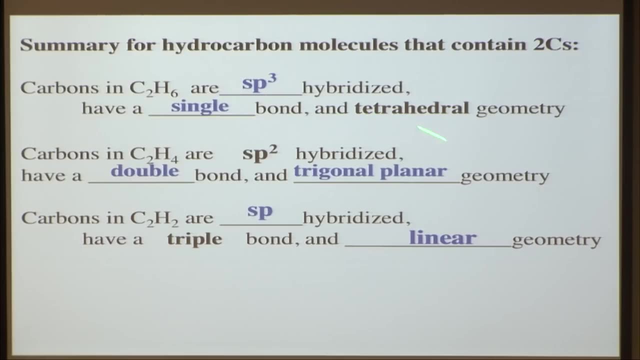 It doesn't care, double, triple, single, whatever- But it doesn't really have a lot of lone pairs on it. But oxygen and nitrogen have lone pairs And whenever you have lone pairs you have to worry about what the geometry is. 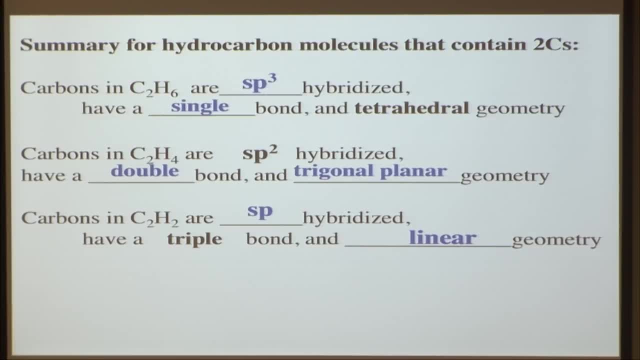 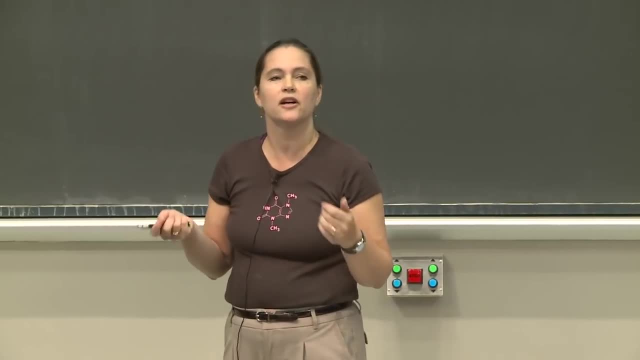 because the geometry gets named based on the atoms that you do see, not the lone pairs. So this cheat sheet works for carbon without lone pairs. If you have lone pairs, you've got to go back to your VSEPR and think about what the name is. 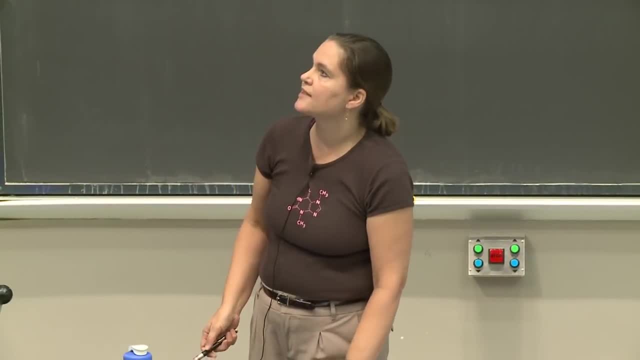 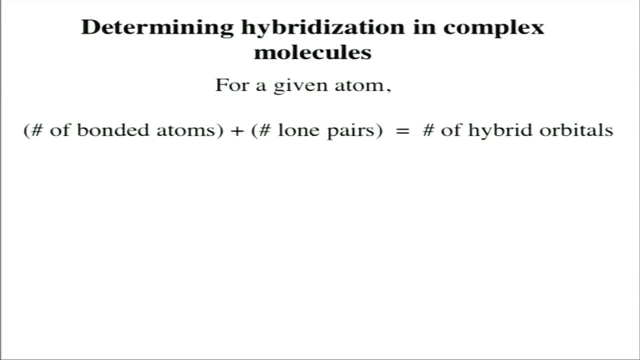 OK, So that's what the names of the geometries are. OK, so rules- and I posted this on Stellar for the problem set that was due today And so very simple for determining hybridization, And this is the kind of equation that 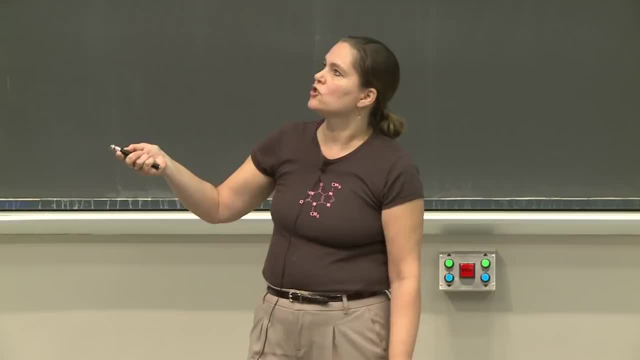 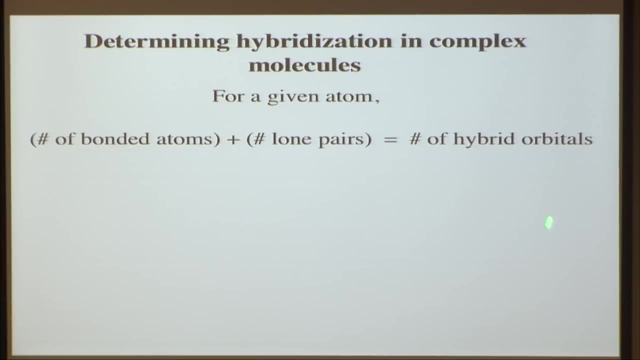 will not be on an equation sheet for an exam. You just need to know that. So in determining hybridization of an atom in a complex molecule, you're going to be thinking about the number of bonded atoms plus the number of lone pairs is going. 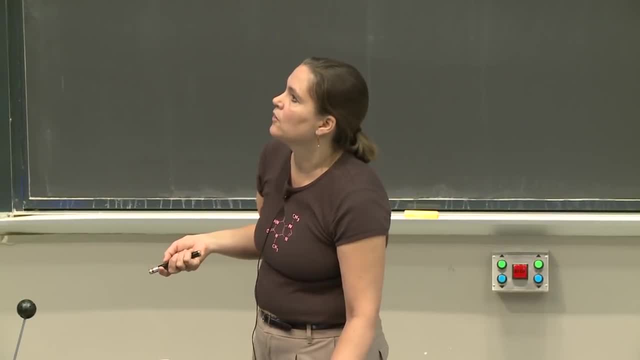 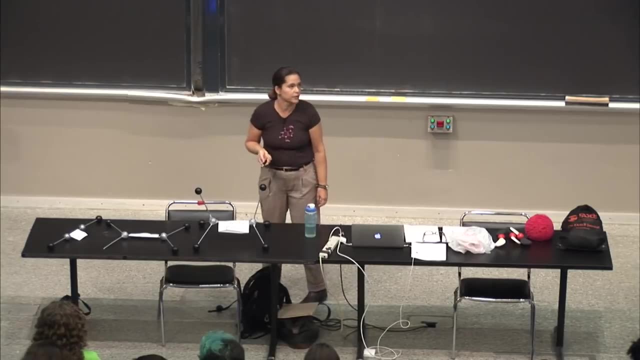 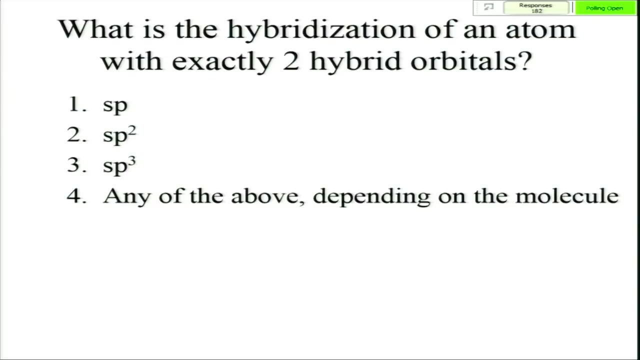 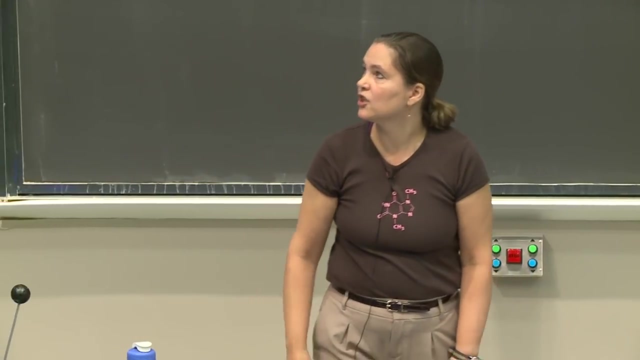 to be the number of hybrid orbitals. So now clicker question: what is the hybridization of an atom that has exactly two hybrid orbitals? All right, 10 seconds. Yes, right, sp. So we can take a look at that. 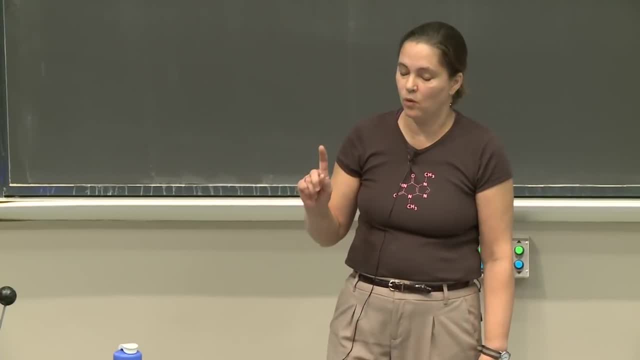 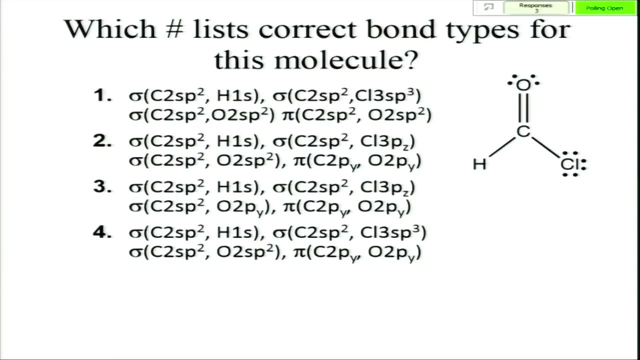 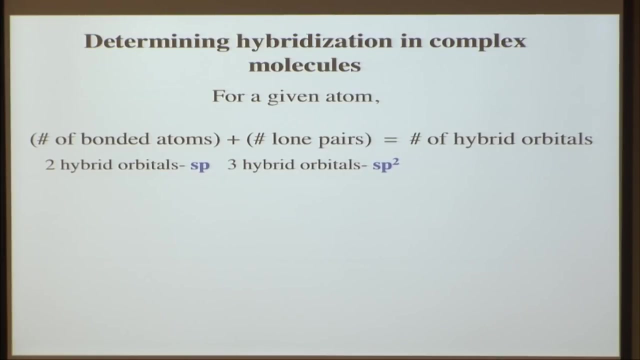 Two hybrid orbitals are formed by one s orbital and one p orbital, And if you have two things bonded and no lone pairs, that's what you would get. Three hybrid orbitals would be sp2, and four would be sp3.. So, again, you're going to just be thinking in these problems. 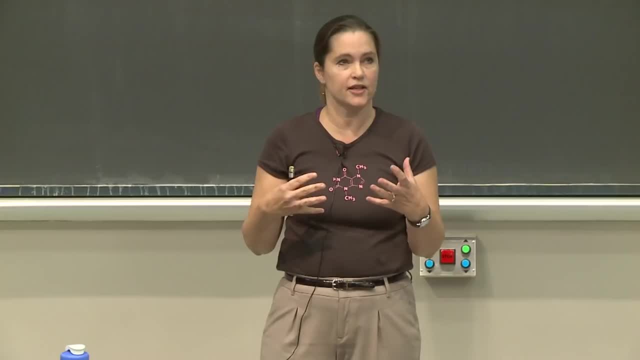 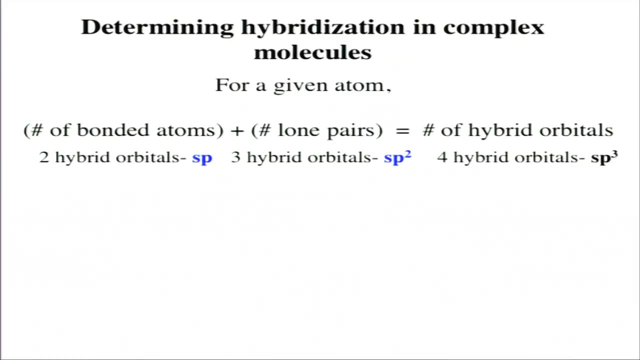 about how many atoms are bonded to that central atom and how many lone pairs do you have? And that's going to then let you figure out what your hybridization is. And we have one exception, which is that if an atom has a single bond, 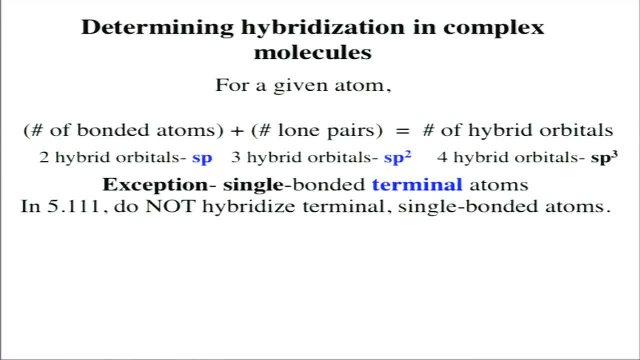 and it's terminal on the edge of the molecule, then we're not going to hybridize it. So we can now take a look at an example of this, And there are in. this is going to be another. Yeah, just keep your clickers out. 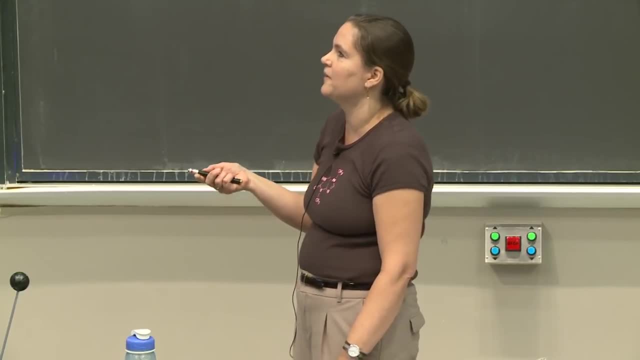 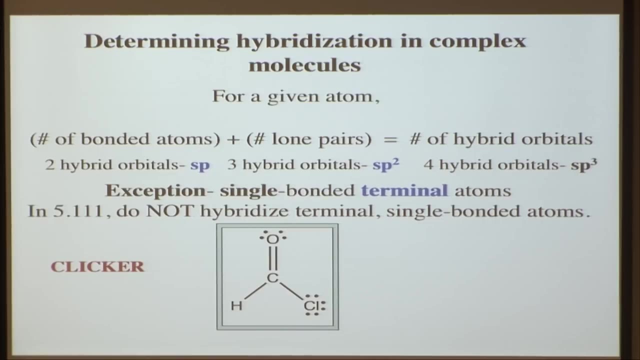 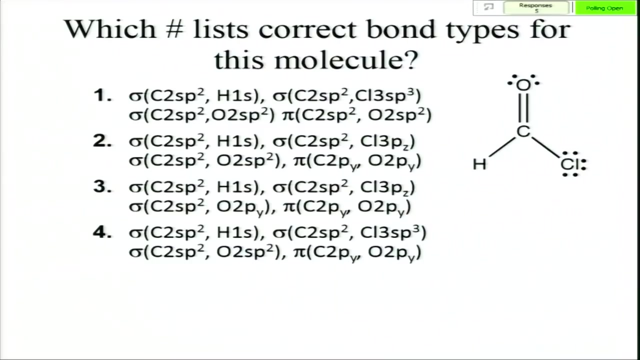 We've got a whole bunch of clicker questions coming at you kind of in a row here, And if we have this molecule, it has a central carbon and three terminal atoms. Now help me figure out what kind of bond. So which one of these has the correct bond types? 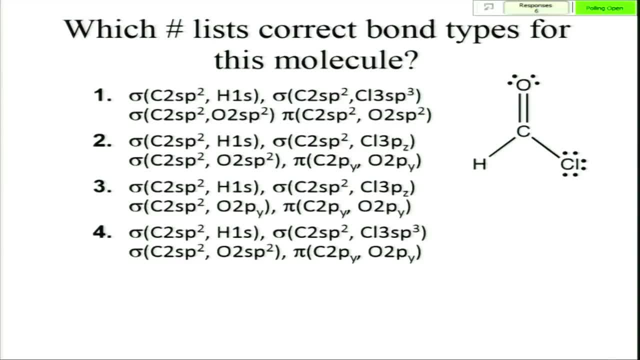 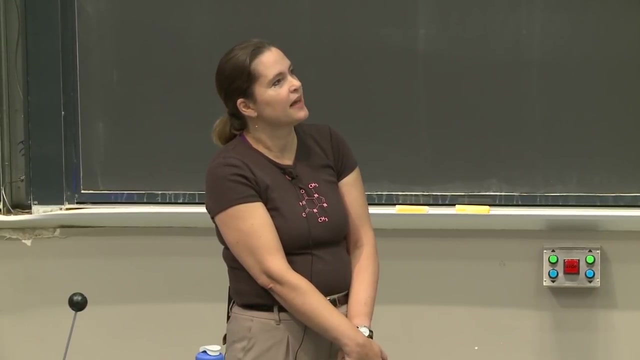 for this molecule. All right, Let's make a decision. Let's just take 10 more seconds Interesting. I think sometimes we might repoll, but I think that we'll just kind of go over this one And then we'll. why don't you? do you want to go ahead? 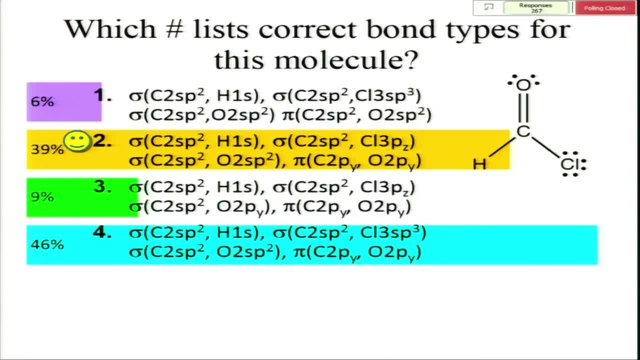 and show the answer. and then this isn't it. And if it wasn't a clicker competition, I might have you discuss it more and repoll. but it's a competition, So let's go over it. So this one isn't in your notes. 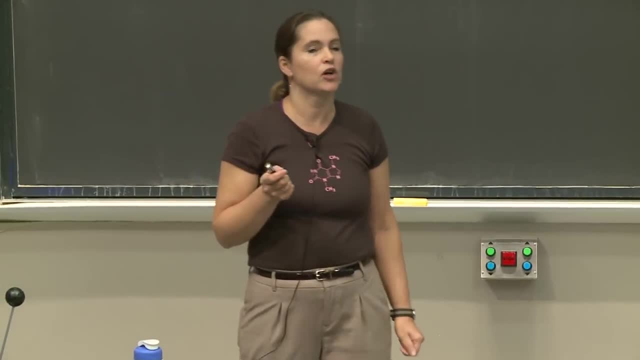 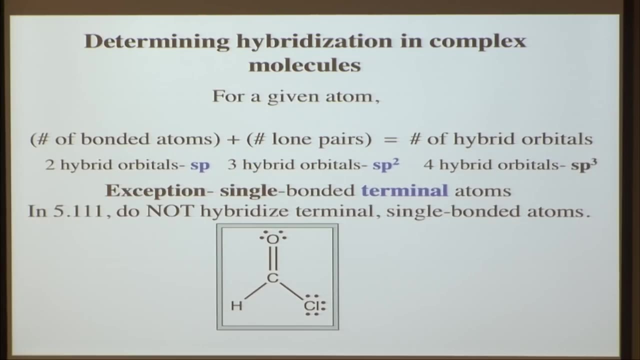 So if you want to write it at the bottom of the page, we'll go over what the answer is. Hopefully there's not a typo in there, but we'll see when we go through. All right, So let's take a look at this molecule. 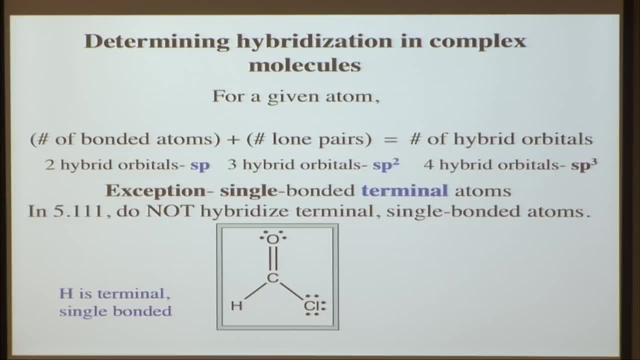 Hydrogen is terminal and single bonded. We've already talked about hydrogen, so we kind of knew that Oxygen is terminal but it's double bonded so we need to hybridize it. Cl is terminal and single bonded, So we don't hybridize this and we don't hybridize hydrogen. 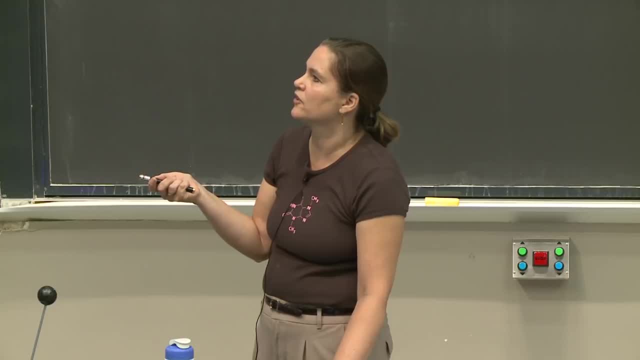 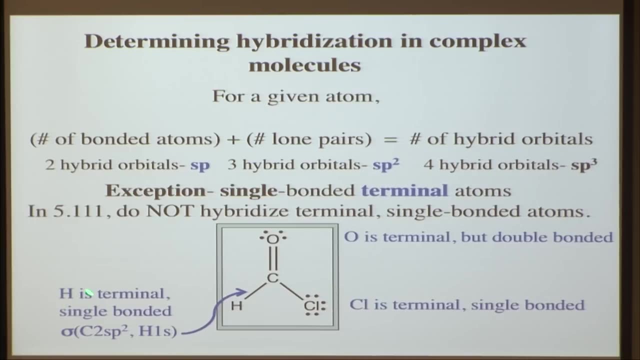 never hybridize hydrogen. OK, So let's look at the kind of bonds that are formed. So we have a sigma bond, single bond. This carbon is carbon 2sp2.. It's bonded to three different things and it has no lone pairs. 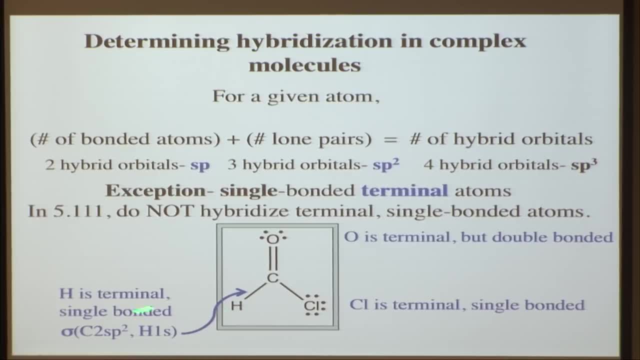 So that makes it three, the three things. So we have three hybrid orbitals, which is sp2.. Our hydrogen is just 1s. It's always just 1s, That's all it is. So let's look at this bond now. 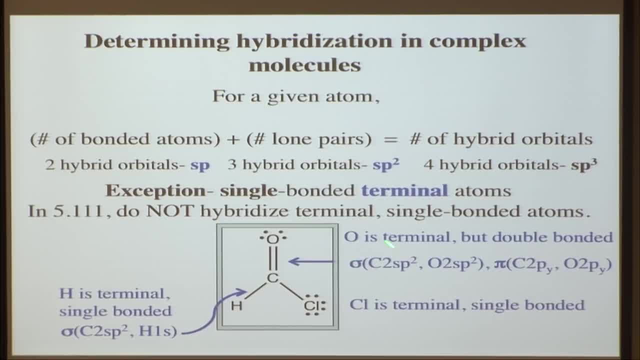 So we have a single bond between our carbon, that is 2sp2.. And then we also have this oxygen. We do hybridize it because it has a double bond And it has two sets of lone pairs and it's bonded to one atom. 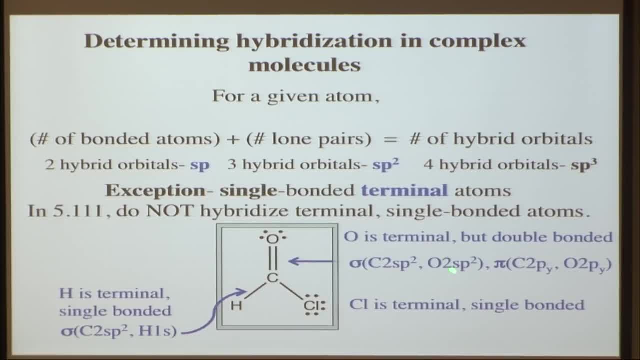 So it has three hybrid orbitals, So it's sp2, just like the carbon. And then we have a pi bond, and the pi bond is made up of atomic orbitals. And then we have a pi bond, and the pi bond is made up. 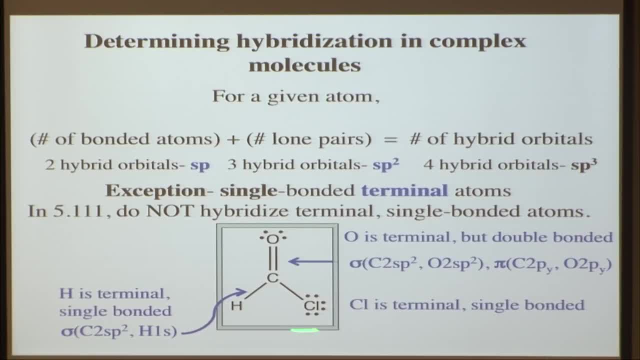 of atomic orbitals, either 2px or 2py. Chlorine is single bonded, So we're not going to hybridize it because it is single bonded and it's terminal, So it's a single bond. It's from this carbon. 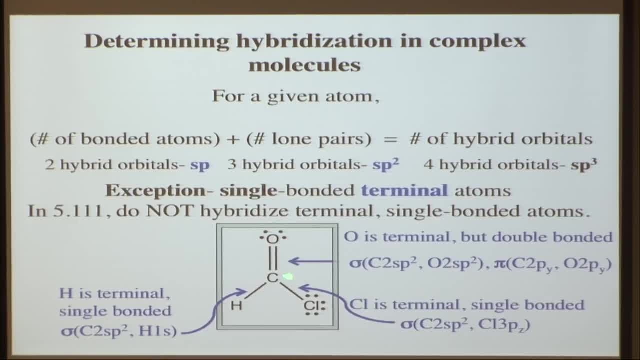 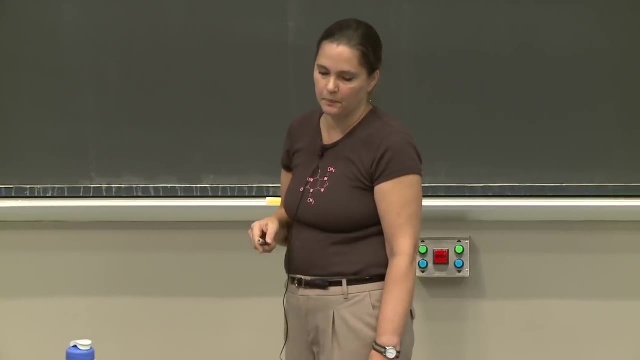 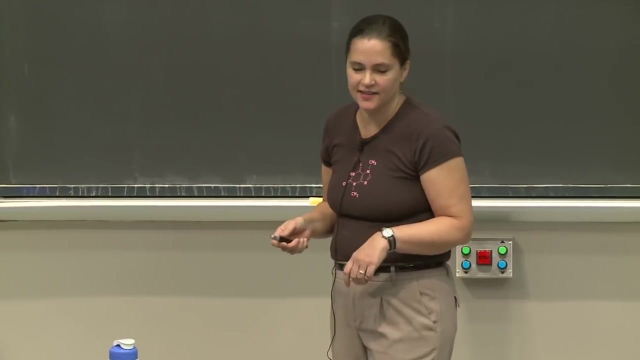 That's carbon 2sp2.. We already saw that. And then the chlorine is going to be terminal, And so it's chlorine 3pz, And so we don't. that's a non-hybridized orbital, So good practice for the clicker. 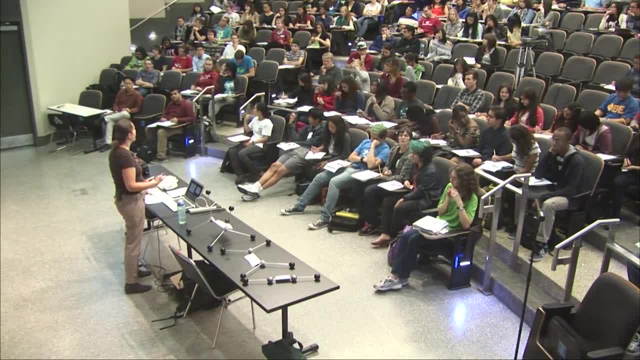 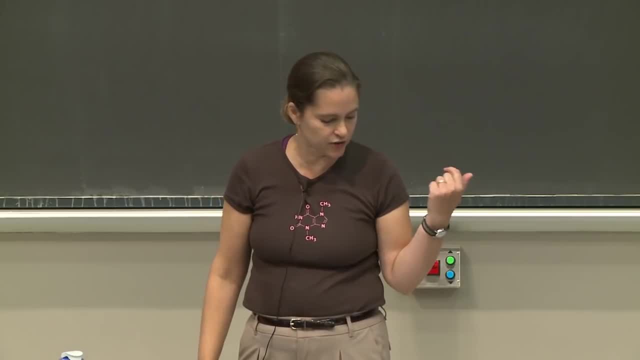 I think that one could help, But we're going to have more practice now. I threw in a bunch of extra problems, So that one was extra, And now let's do the one that is in the notes from last time, which is vitamin C. So I'll give you. 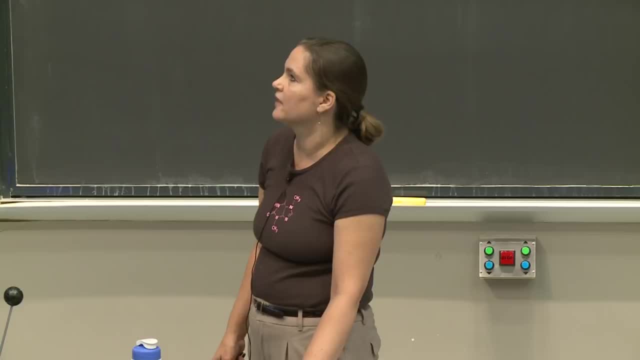 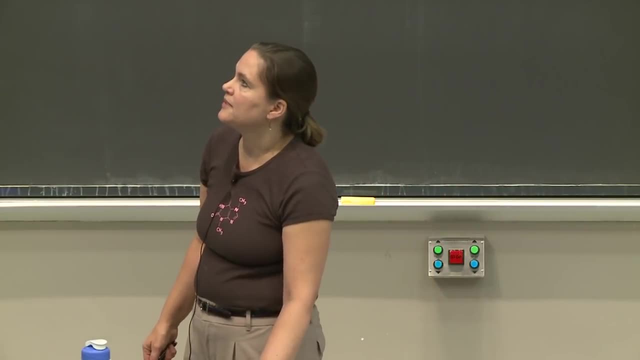 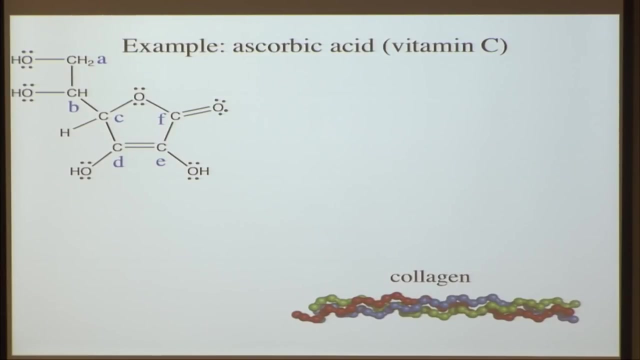 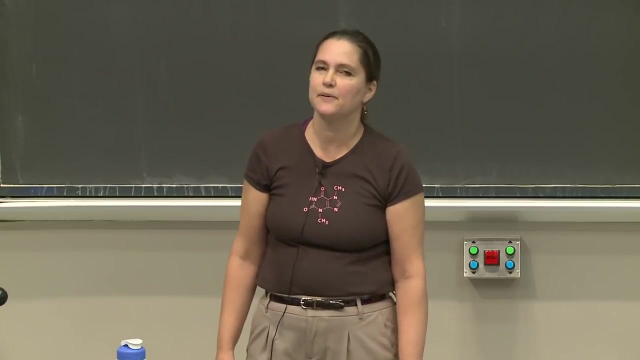 another minute if everyone has that one down. OK. So let's look at vitamin C. So vitamin C is needed to form collagen in your body. Without enough vitamin C in your diet you could be in trouble, So it doesn't happen too much anymore. because there's vitamin supplements and all sorts of things, But often vitamin C. Vitamin C deficiency is associated with sailors who went out to sea and didn't have a healthy diet And they became deficient in vitamin C and got scurvy, And so then they had to figure out. 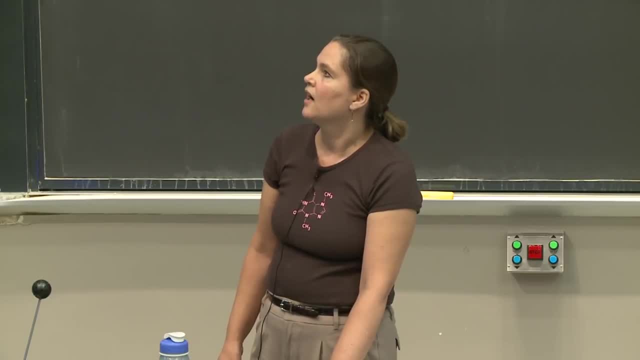 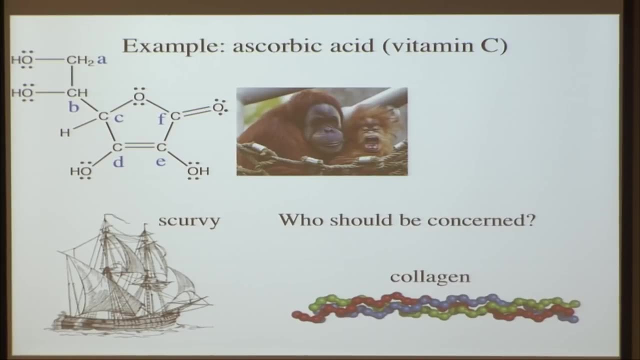 they had to eat oranges or other things that were rich in vitamin C. In terms of who should be concerned about vitamin C deficiency: us primates. we don't make vitamin C, So we have to get it in our diet. And also guinea pigs. 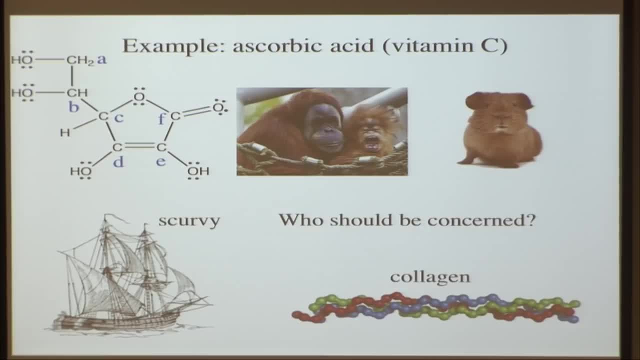 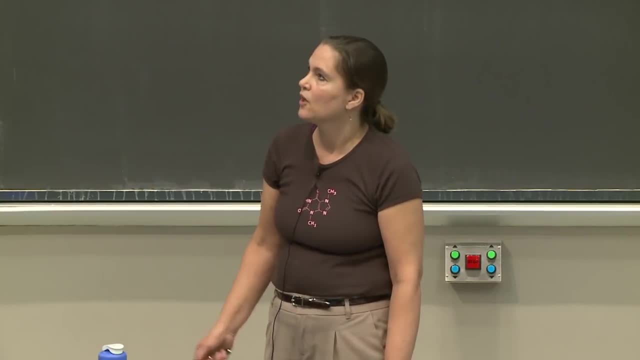 Most other animals make it. I don't really know why. Maybe this is why guinea pigs are called guinea pigs. They're good for scurvy experiments because they don't make vitamin C All right. So let's look at this vitamin C molecule. 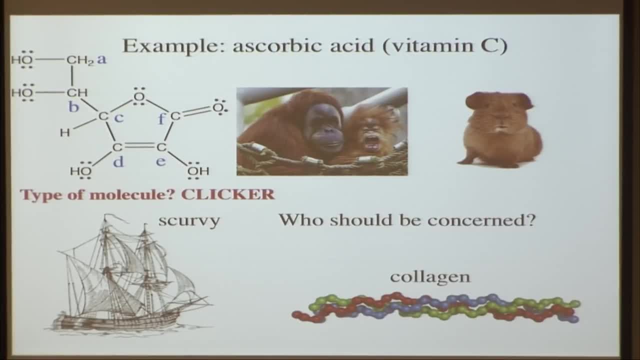 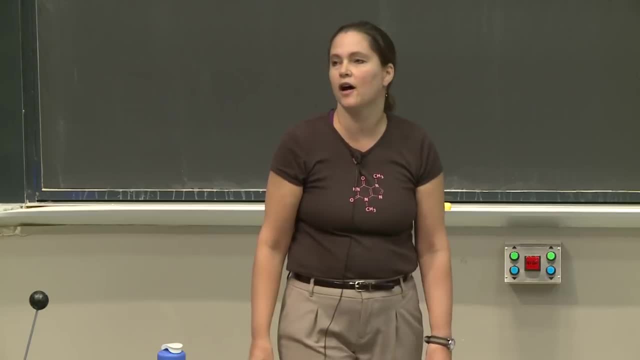 and think about what type of molecule it is, And this is a clicker question, So we have to remember back more material that's going to be on exam. two: Does that look like a polar or non-polar molecule, And what's true about polar and non-polar molecules? 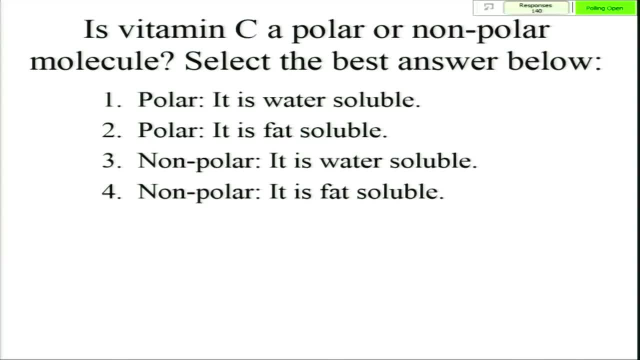 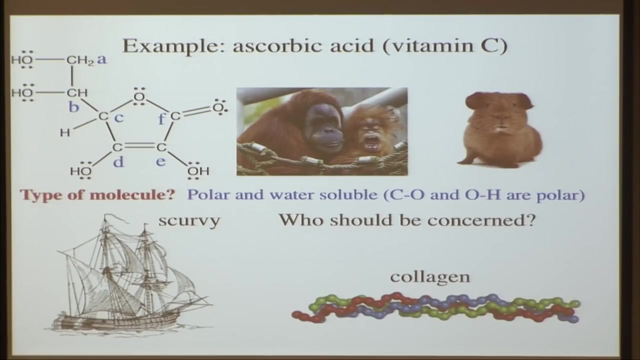 All right, Oh really, No more questions. All right, 10 more seconds. All right, 10 more seconds, All right, Great, Awesome, Thank you. So it is polar and it's therefore water-soluble. 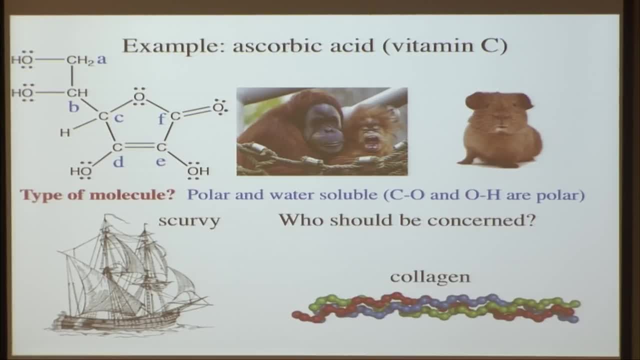 And so you know that, because if there's atoms in there that have differences of electronegativity of greater than 0.4, carbon and oxygen have a difference in electronegativity of greater than 0.4, oxygen-hydrogen also. 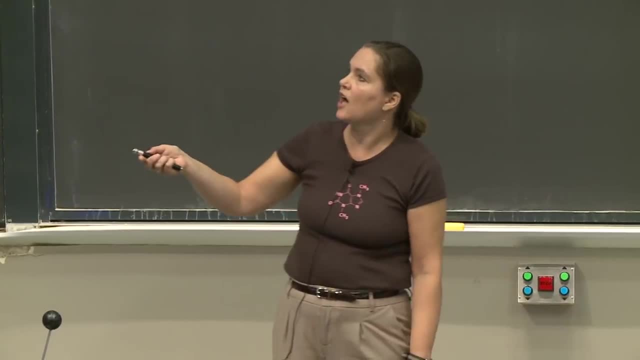 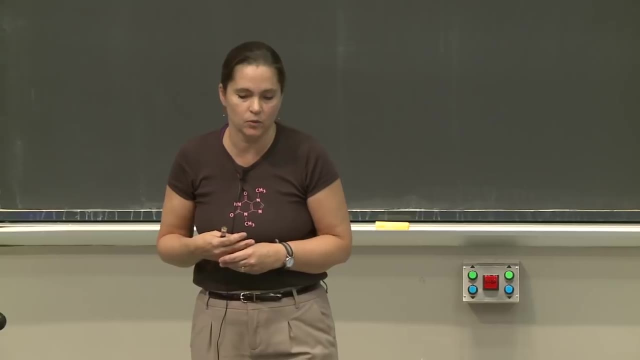 electronegativity difference is greater than 0.4.. So we have a lot of polar bonds and they're not canceling each other out. It's not a symmetric molecule, So therefore it would be a polar molecule and water soluble. 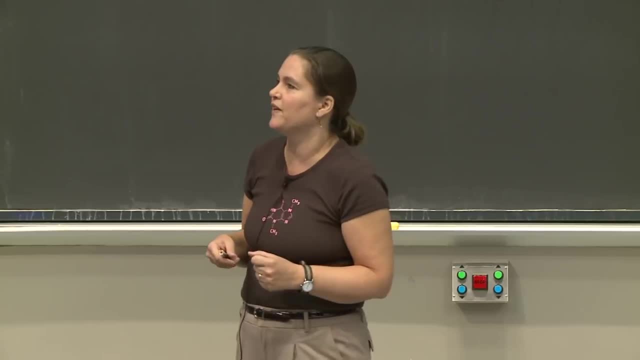 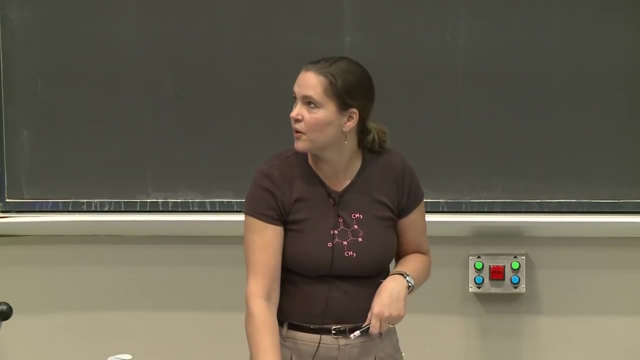 OK, great, So I think you're good on your polar covalent bonds, which is also going to be on exam two. All right, so let's go back to hybridization and have a little more practice on that, So don't put your clickers away. 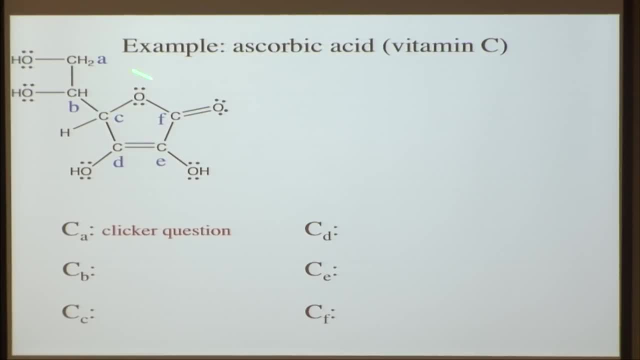 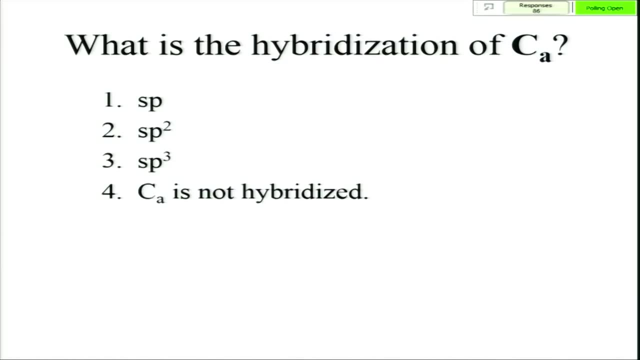 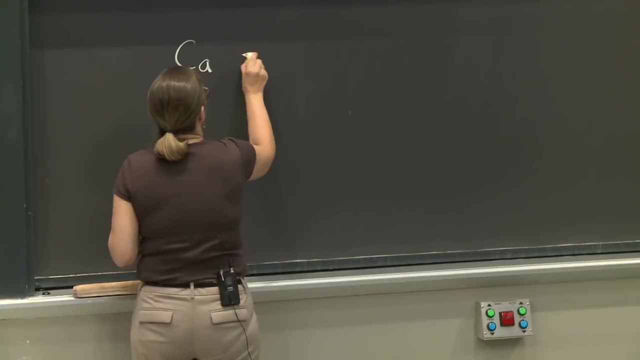 Why don't you tell me the hybridization of carbon A labeled up here And in your notes? All right, 10 more seconds. All right, So we know what clicker questions are going to determine the winners. OK, so carbon A was sp3 hybridized. 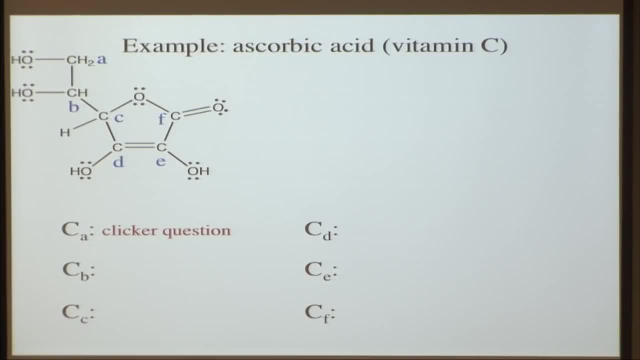 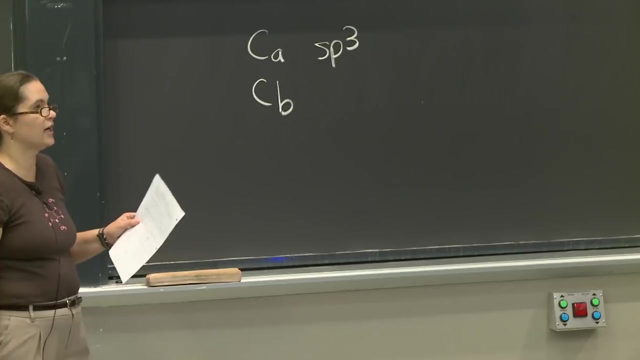 So if we look at it over here, it has bonded to four things. So there's four, which makes it sp3.. OK, so let's just do the rest And you can yell these out. Carbon labeled B. what kind of hybridization for carbon B. 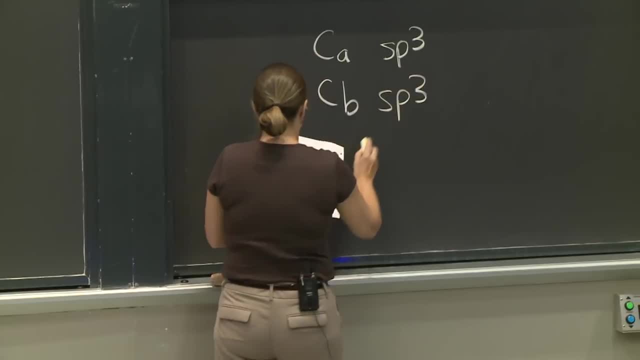 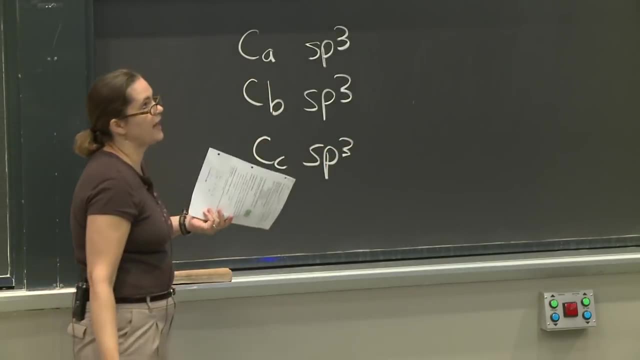 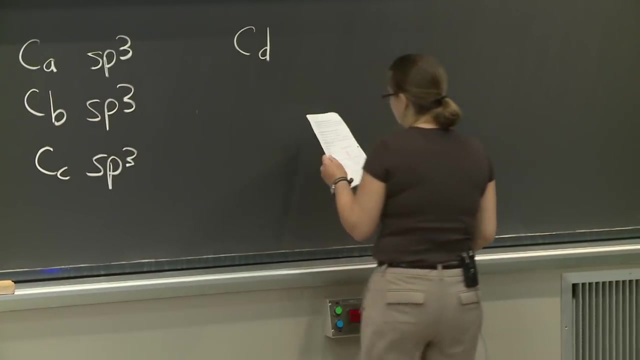 OK, Sp3. Sp3.. Carbon C: Sp3. Sp3.. Again, we just want to count how many bonds you have going on or lone pairs, But carbon doesn't usually like to have lone pairs. What about carbon D? 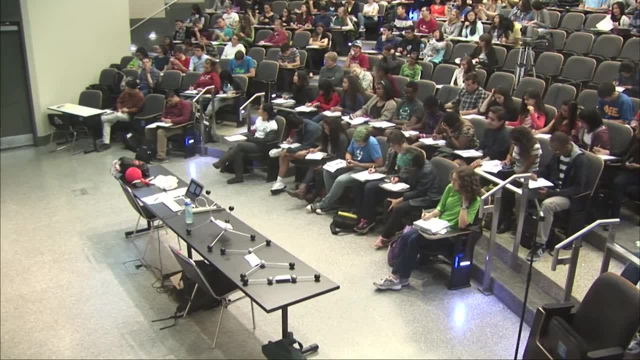 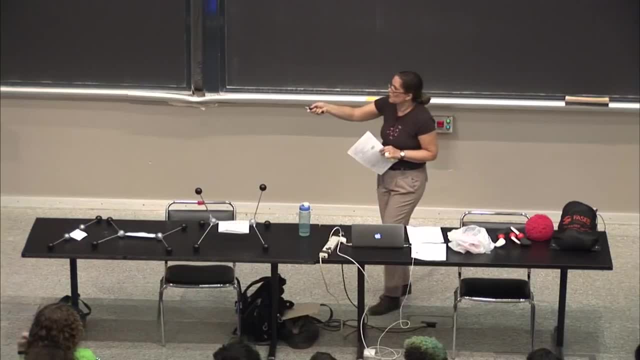 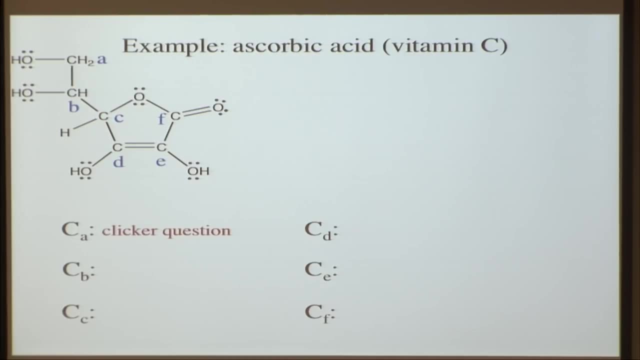 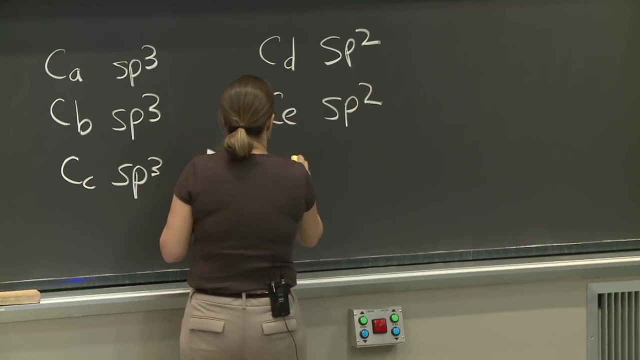 Sp2.. Sp2, right, It only has. if we look at that one over here, I'm supposed to point to this one. So carbon D over here it has three atoms that it's bound to: carbon E- sp2, and carbon F- sp2.. 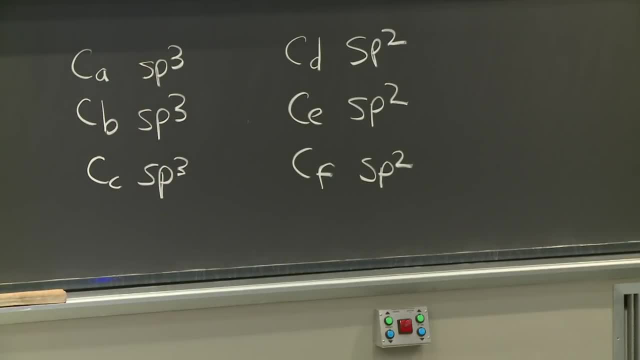 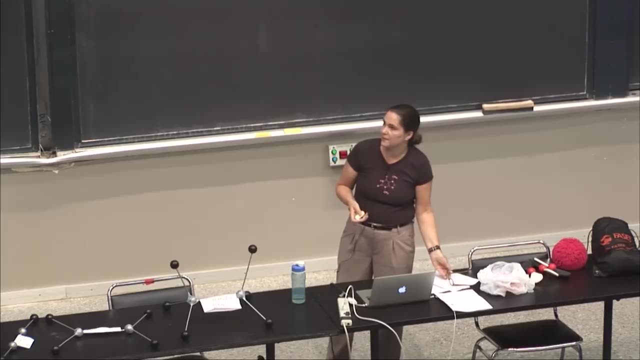 All right. so now that we did that, we can use this information when we think about the bonds that are formed between these carbon carbons and the other atoms. So let's look at bonding now. So if we look at carbon B to hydrogen, 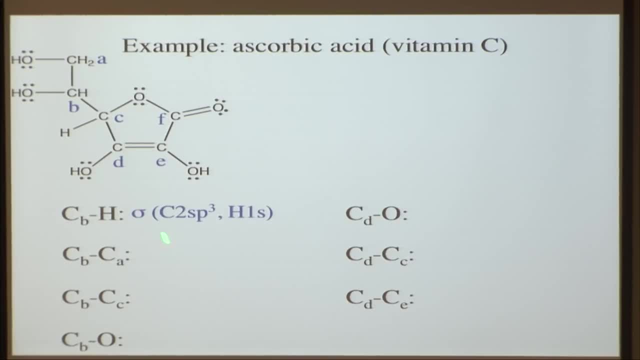 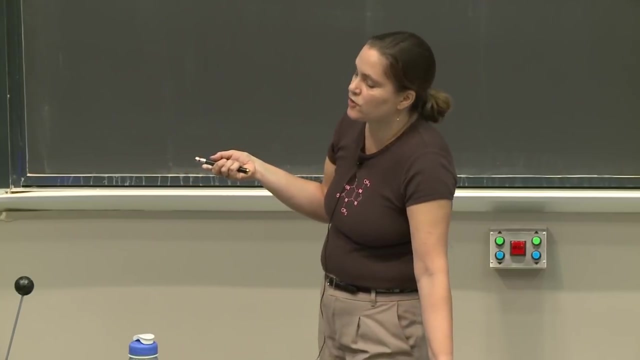 that's going to be a sigma bond And you told me that carbon B was sp3, so we write that. So describe the symmetry around the bond name: the bond carbon 2sp3, hydrogen 1s. We do not hybridize hydrogen. 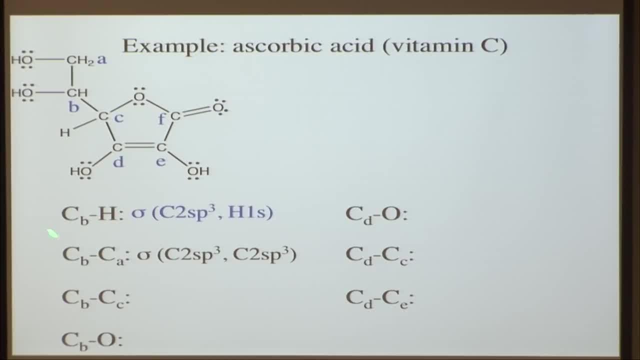 So now for the bond between B and A, again a sigma bond. We already looked at the fact that carbon B is 2sp3.. Carbon A was the same. Now, if we look at the difference between B and C, B was carbon 2sp3, and then C is also the same. 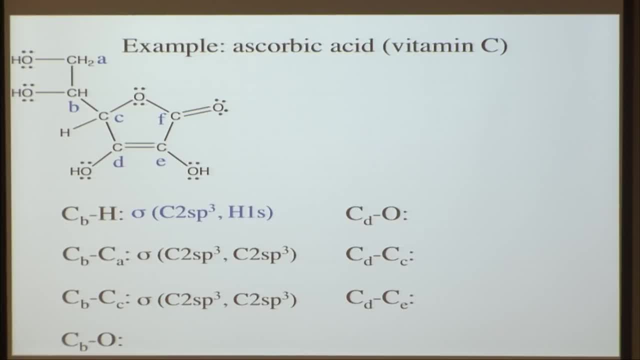 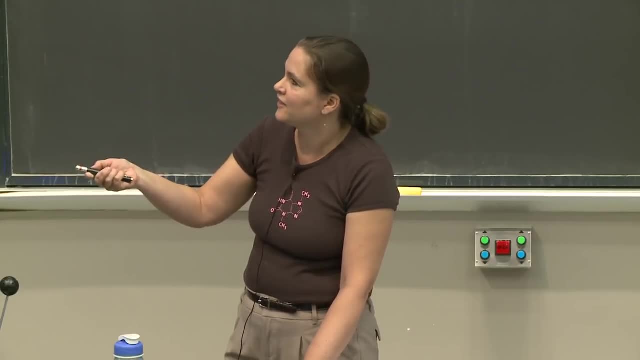 Remember to write the 2s. Remember to write the hybrid. Remember to write the element. Remember to write sigma for the single bond. Grading these questions on the exam is not fun. You've got to remember to have all those things in there. 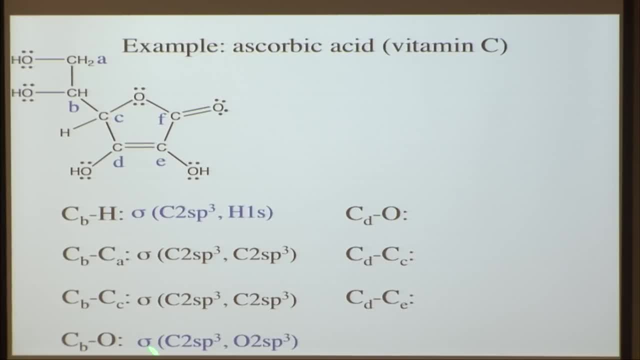 So if you get them all in there, it makes everyone very happy. OK, now let's look at carbon B. to the oxygen, It's also a single bond. So, sigma, we know that carbon B is C2sp3.. The oxygen here is also going to be sp3. 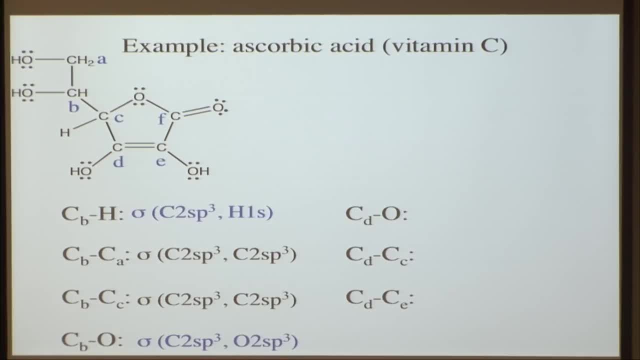 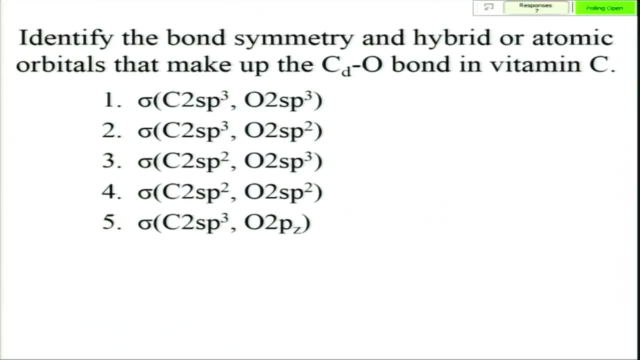 And so we're going to have to read this one: The oxygen here is going to be sp3, because it has 2 bonded atoms and 2 sets of lone pairs. OK, one more clicker, Great yup. So that is correct. and if we take a look at that over here, we have carbon D. It has 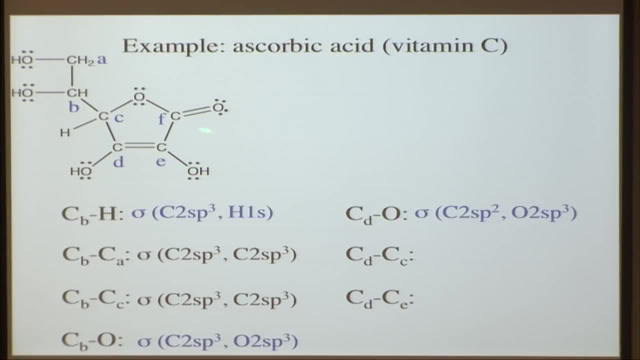 bonded to three things, so it's sp2, and the oxygen is bonded to two atoms and two lone pairs, so it's sp3.. We can keep going and finish up between D and C. now We have- oops, sorry, D and C up here. 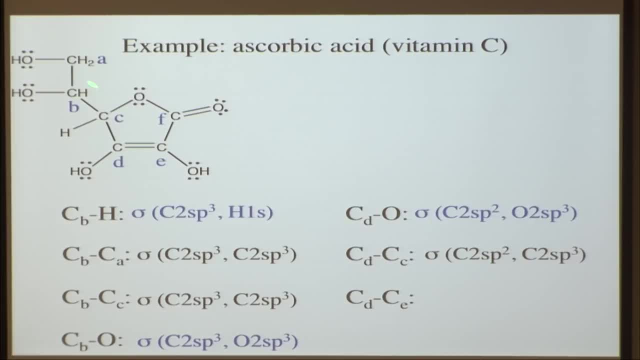 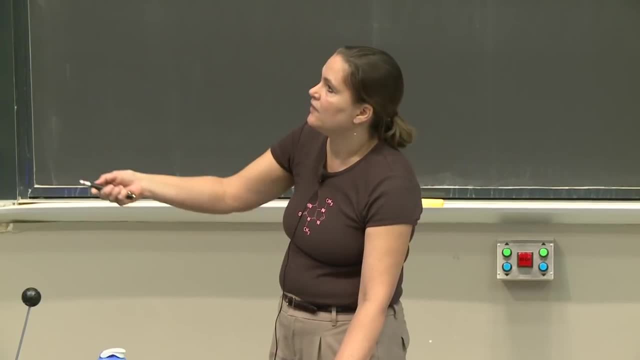 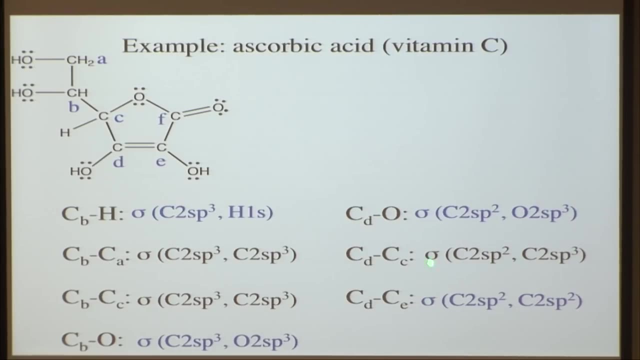 We have D, which is 2sp2, bonded to three things. C has bonded to four things, It's c2sp3.. And then, finally, D2e. We have two bonds, We have a sigma bond, so that's between these two carbons, here our hybridized orbitals. 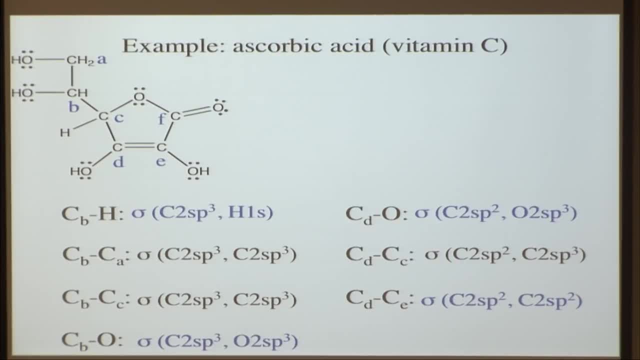 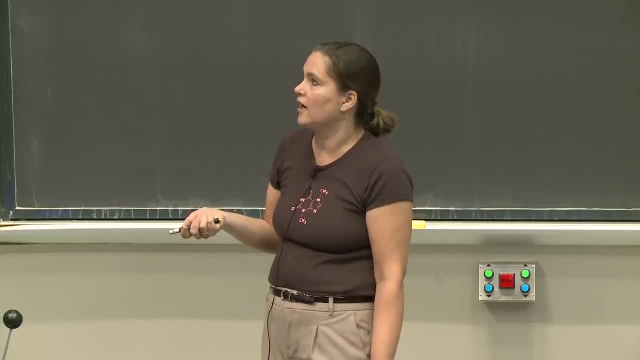 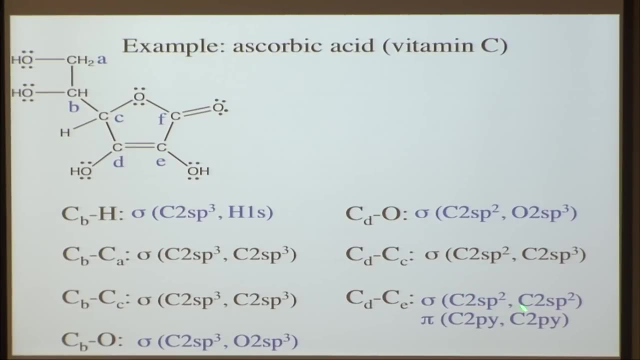 and again it's 2sp2,, 2sp2, and it's a double bond. so we have one sigma and one pi bond, and the pi bond is between non-hybridized orbitals, so it's c2py, c2py or you could. 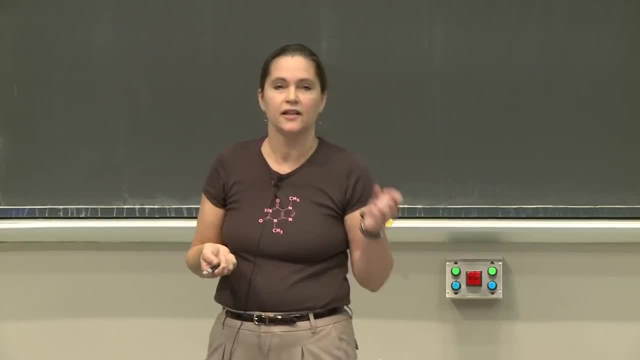 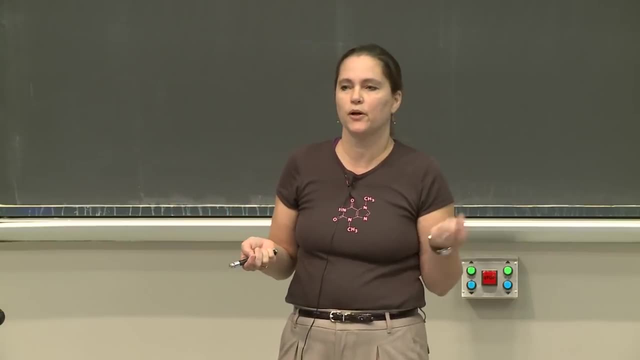 have used x. I don't really care about that. All right, Good practice. I think you're getting the hang of this Again. there'll be more practice problems on hybridization posted today to get you ready for the exam and also to figure out these bonds. 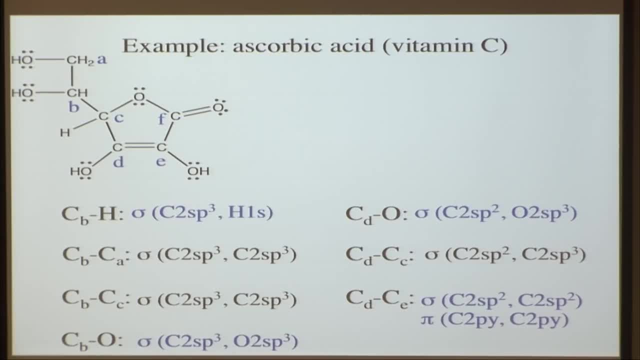 Once you get the hang of this, it's really pretty trivial and good points for an exam.